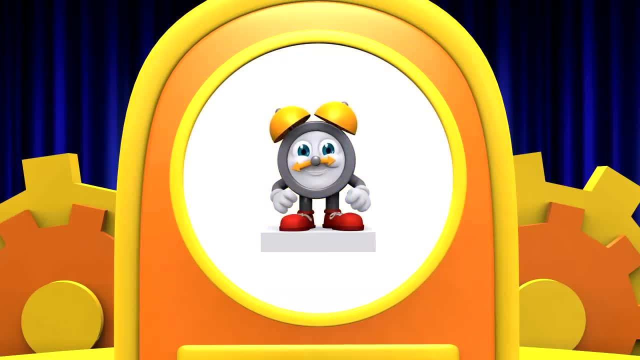 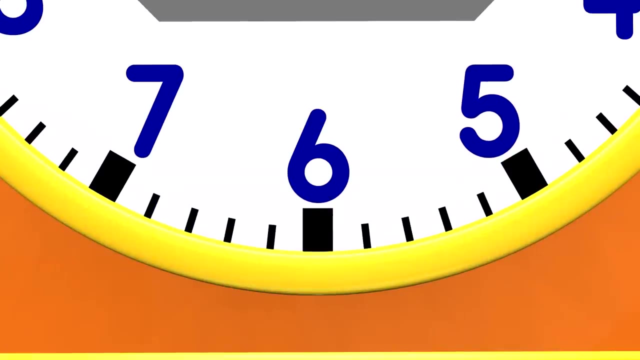 The base of the clock is where the numbers stay In their special places every second of the day. The twelve-inch clock is where the numbers stay. The nine is at the top and the six is at the bottom. Every time you look, that's where you will spot them. 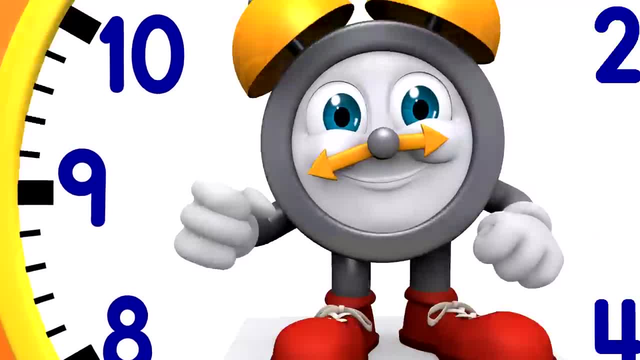 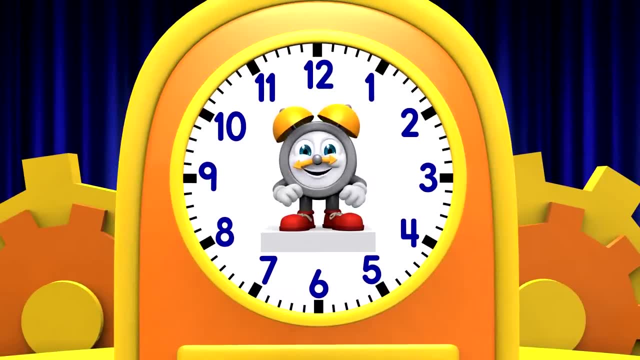 The nine is on the left and the three is on the right. The other numbers fit between in a circle. Let's recite: One, two, three, Four, five, six, Seven, eight, nine, Ten, eleven, twelve. 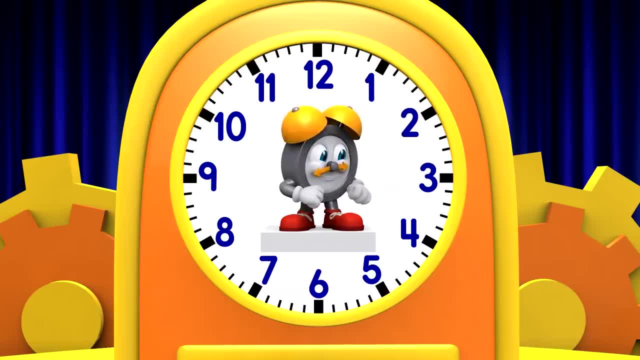 One, two, three, Four, five, six, Seven, eight, nine, Ten, eleven, twelve. Running round the face are at least two hands. The short one moves most slowly as the hour demands. The short one moves most slowly as the hour demands. 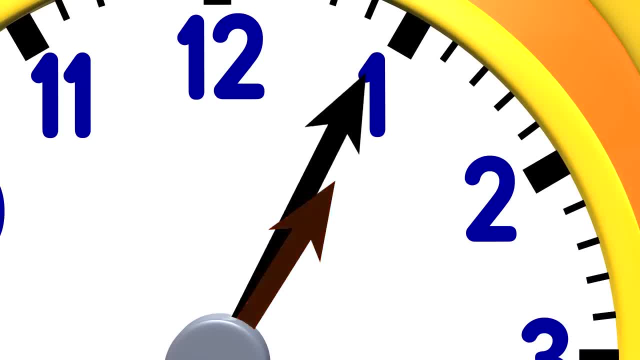 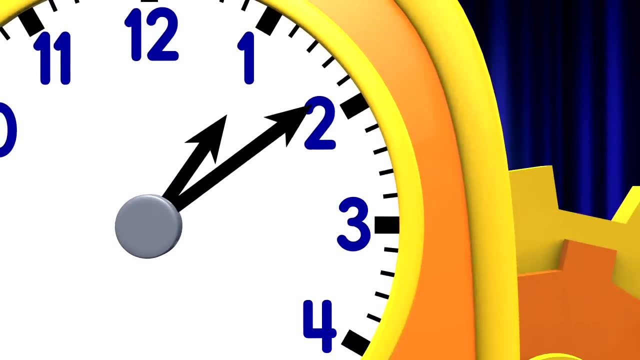 Because the short's hand is the hour hand. He's so slow I could slumber. He takes a whole hour just to reach each number. The long hand is the minute hand. She moves a little faster. Every five minutes she gets a number past her. 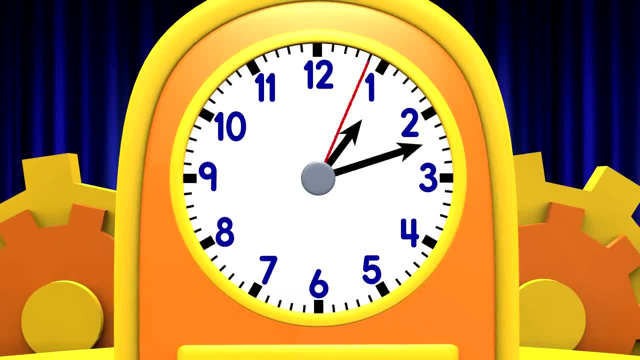 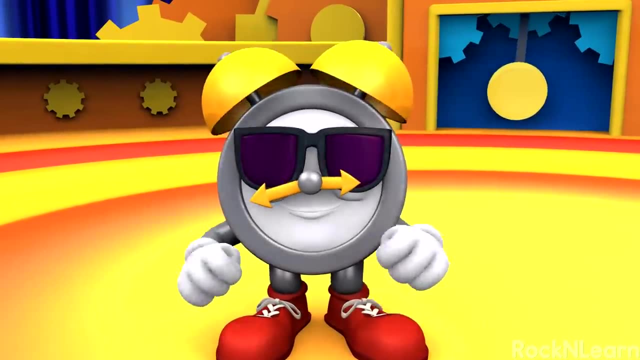 Some clocks have another hand that speeds around the face. This thin one is the second hand. Now, pump up the bass. Yeah, pump up the bass. Pump it up now. Ooh, ooh, Come on, Cuckoo. okay, okay, calm down. 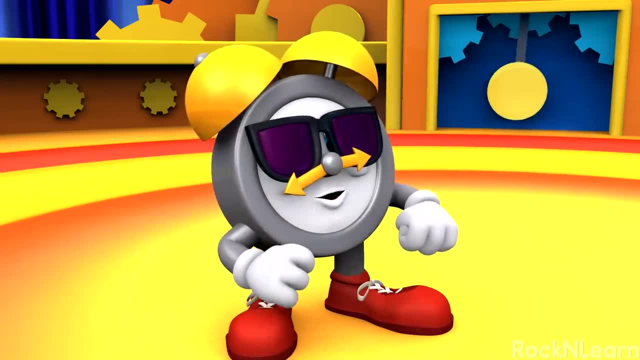 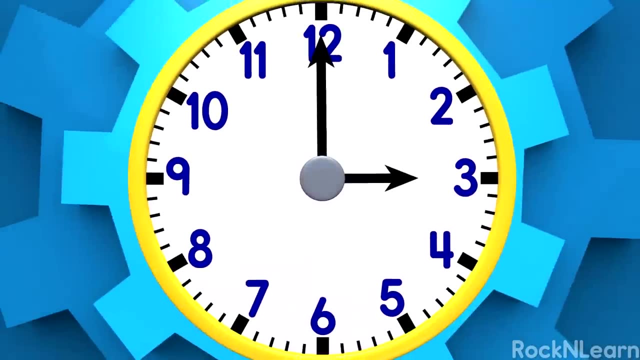 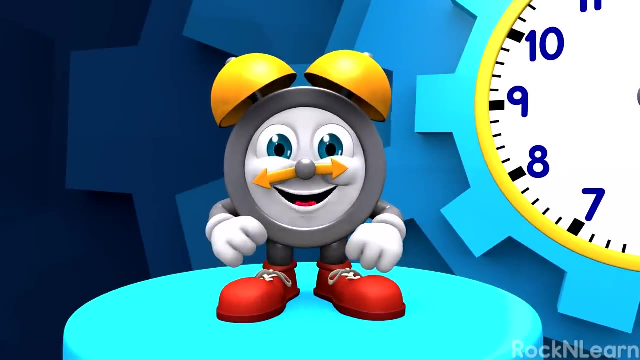 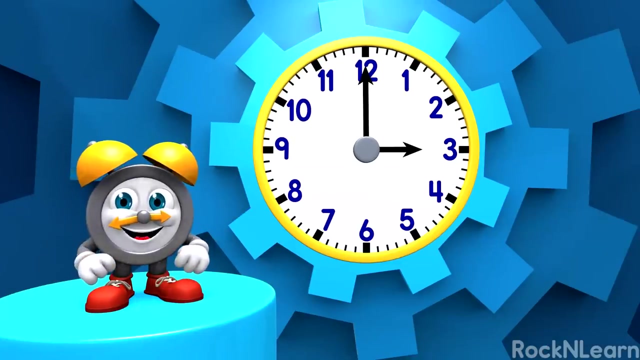 Oh sorry, Cuckoo, I guess I lost track of time. Oh, brother, Speaking of time, Now you know the parts of the clock that you read In order to tell time, a clock is what you need. Let's start out easy. 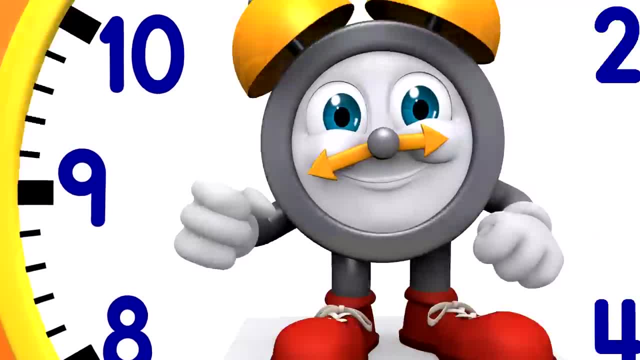 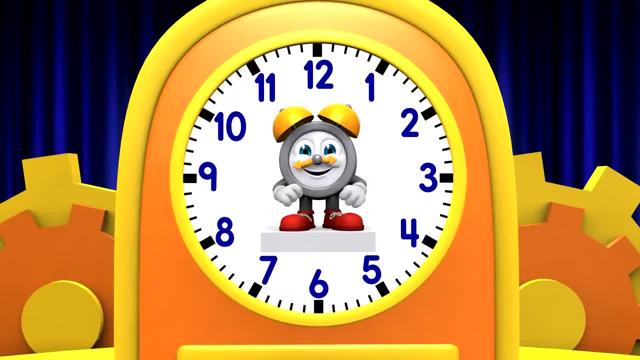 The nine is on the left and the three is on the right. The other numbers fit between in a circle. Let's recite: One, two, three, Four, five, six, Seven, Eight, nine, ten, eleven, twelve. 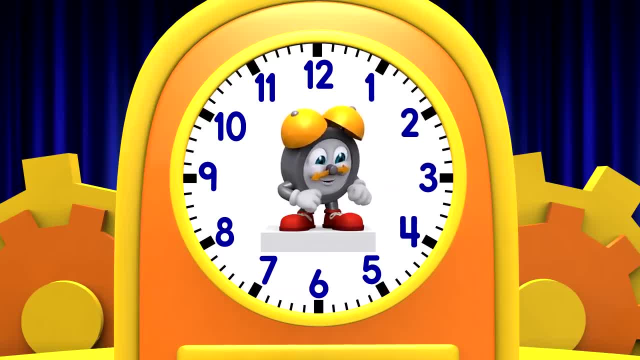 One, two, three, four, five, six, seven, eight, nine, ten, eleven, twelve. Running round the face are at least two hands. The short one moves most slowly, as the hour demands, Because the short's hands are the ones that move the most. 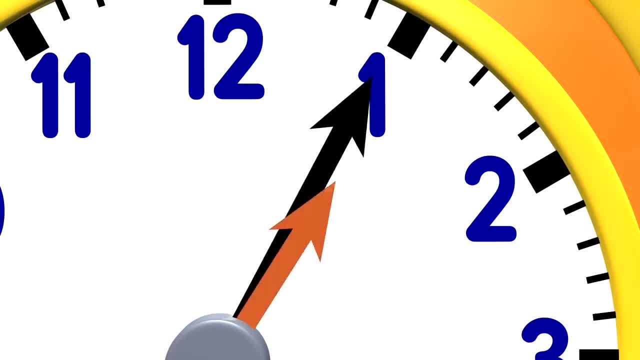 Because the short's hands are the ones that move the most. Because the short's hand is the hour hand. He's so slow I could slumber. He takes a whole hour just to reach each number. The long hand is the minute hand. 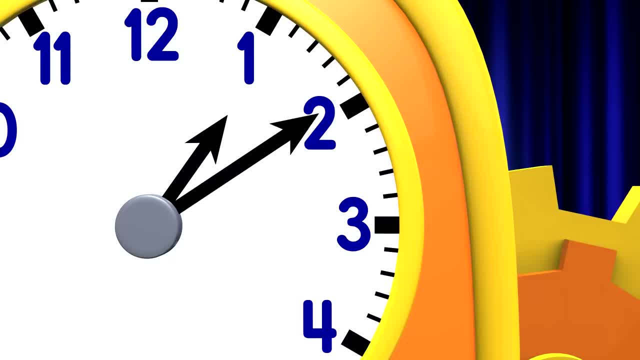 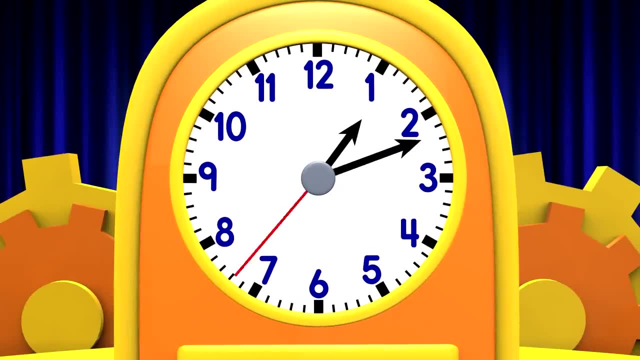 She moves a little faster. Every five minutes she gets a number past her. Some clocks have another hand that speeds around the face. This very one is the second hand. Now pump up the base. Yeah, pump up the base. Pump it up now. 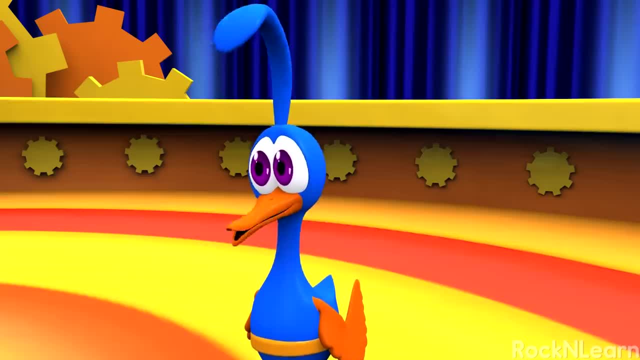 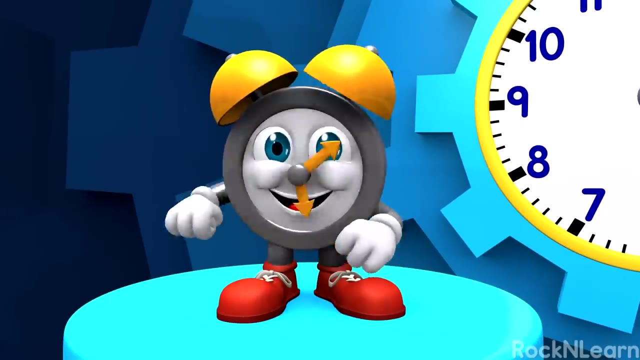 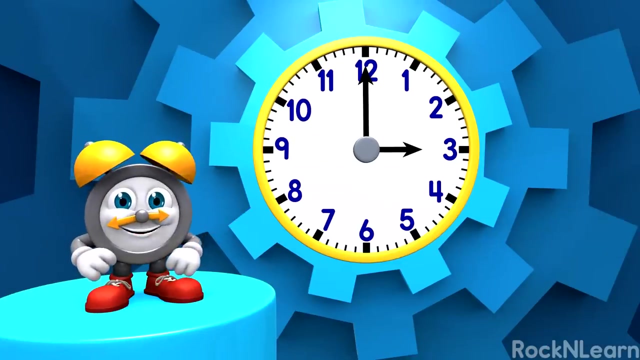 Ooh, ooh, Come on, Cuckoo. Okay, okay, Calm down. Oh sorry, Cuckoo, I guess I lost track of time. Oh, brother, Speaking of time, Now you know the parts of the clock that you read In order to tell time. a clock is what you need. Let's start out easy, Telling time to the hour. I'll teach you a cool trick that will give you the power. 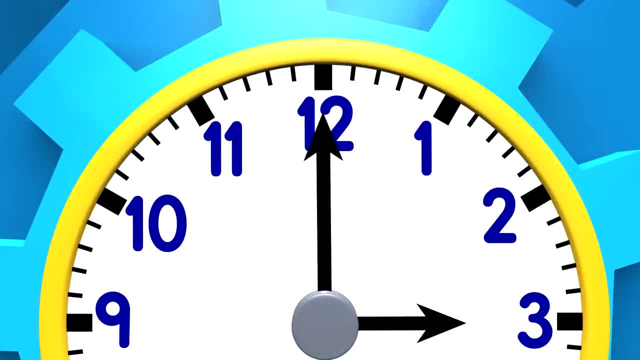 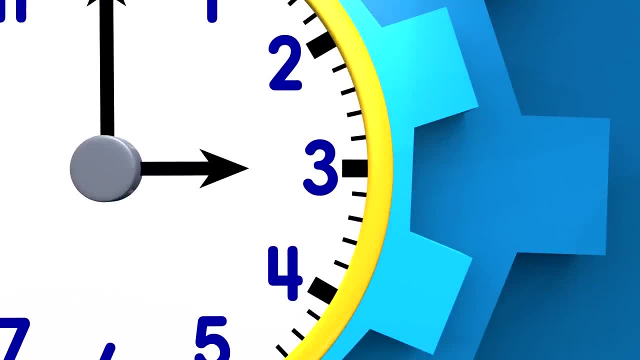 When you see the minute hand pointed straight at the top, it's on the number 12.. So say the word o'clock, Next check out the number the hour hand points to, Then put that number with o'clock. That's all you have to do. 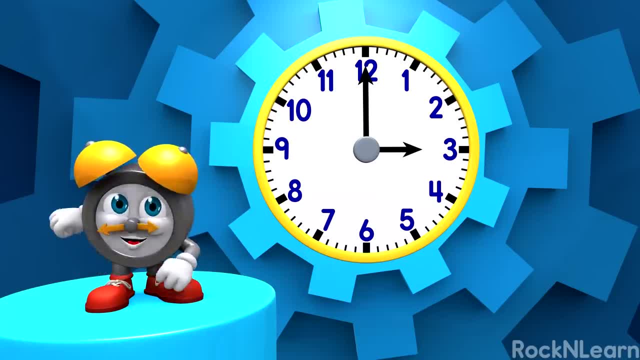 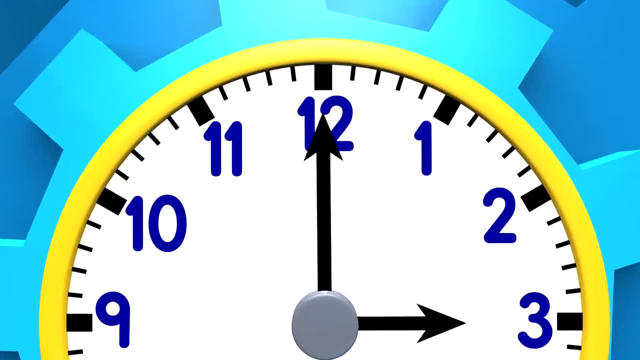 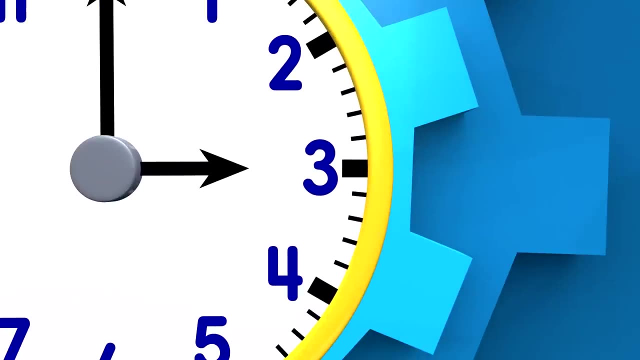 Telling time to the hour, I'll teach you a cool trick that will give you the power. When you see the minute hand pointed straight at the top, it's on the number 12.. So say the word a clock. Next check out the number the hour hand points to. 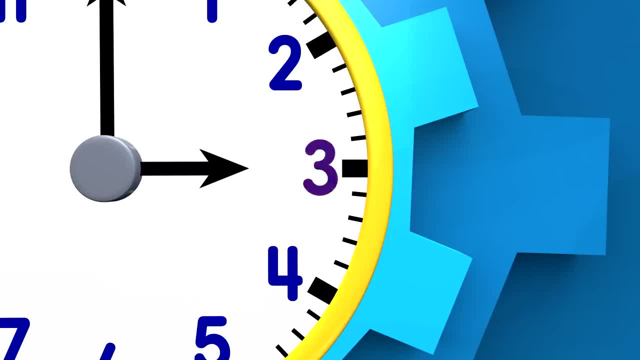 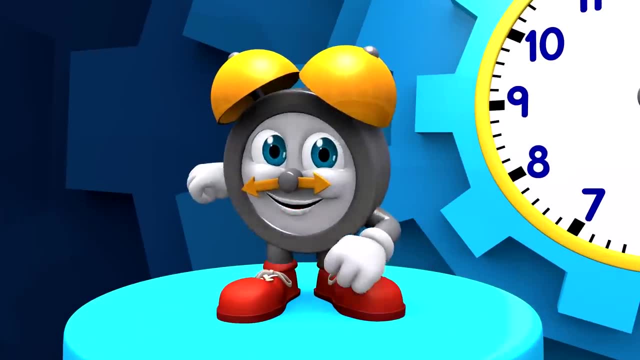 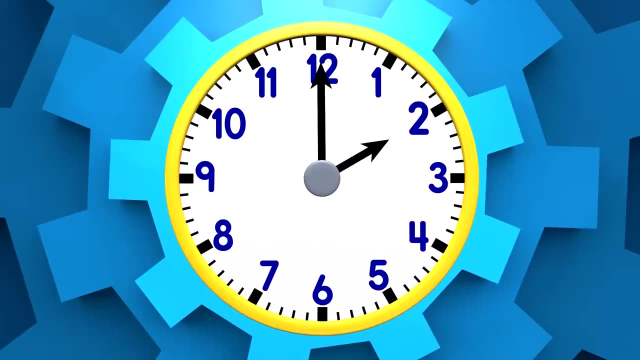 Then put that number with a clock. That's all you have to do. Let's try a few examples. Just take a look at these and say them out loud as quickly as you please: One o'clock, Two o'clock, Three o'clock. 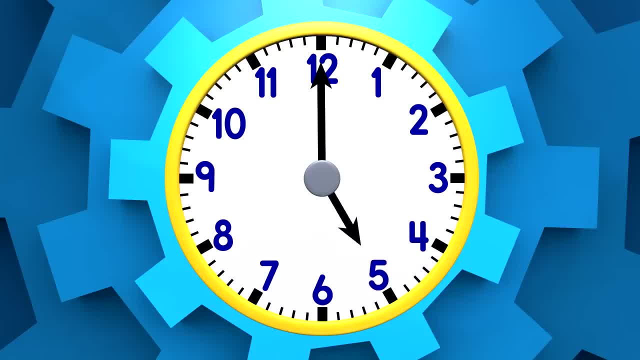 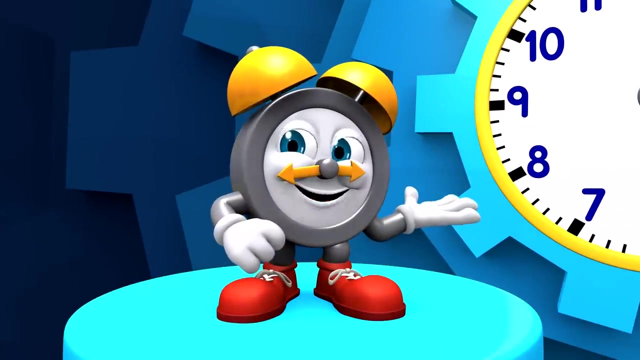 Four o'clock, Five o'clock, Six o'clock, Seven o'clock, Eight o'clock, Nine o'clock, Ten o'clock, Eleven o'clock, Twelve o'clock. Now let's try some other clocks, like ones that you might see, so you get some more practice. 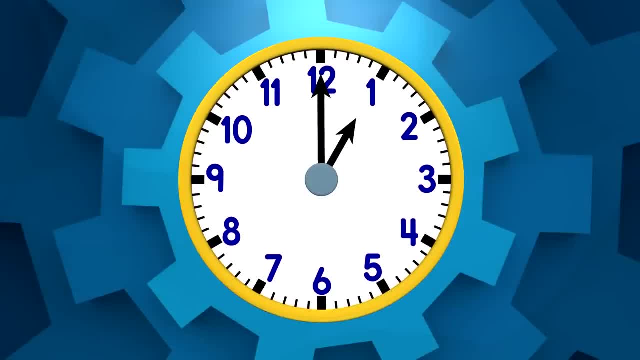 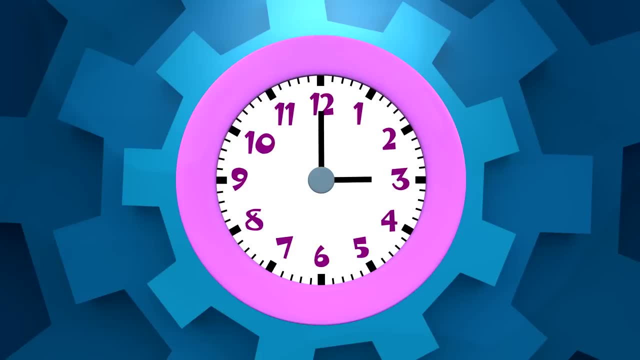 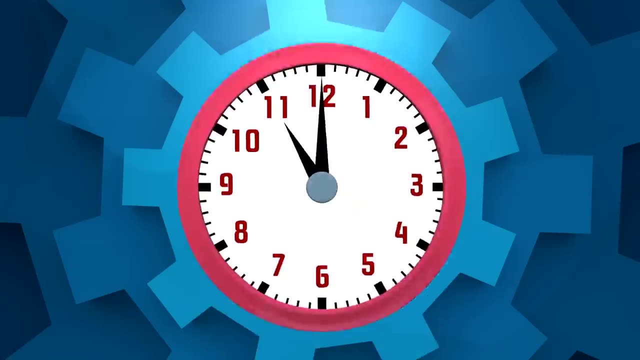 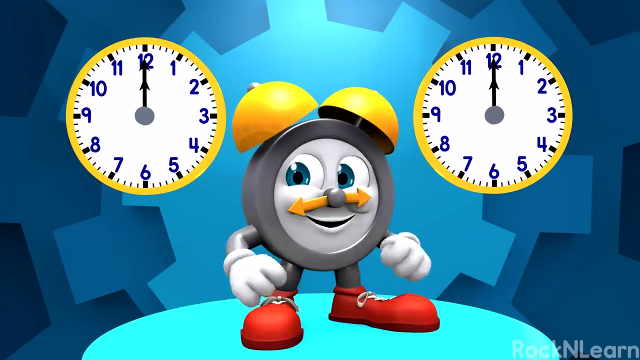 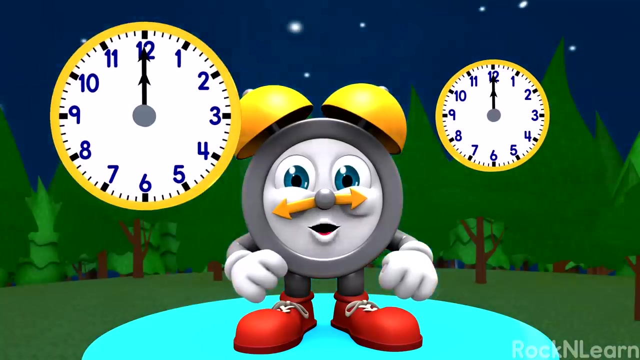 Say these times with me: One o'clock, Three o'clock, Six o'clock, Eleven o'clock. Some of you have noticed something a little strange. It seems we have two of each hour in each day. The first twelve o'clock comes when it is night. 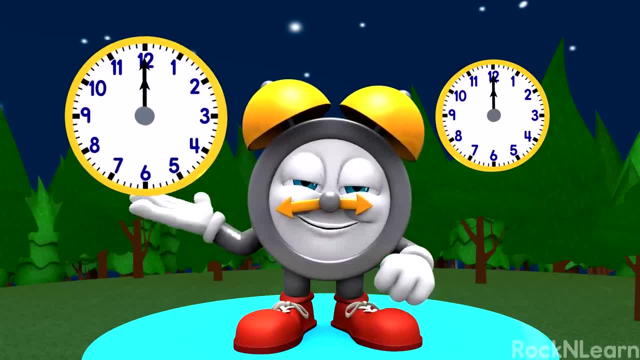 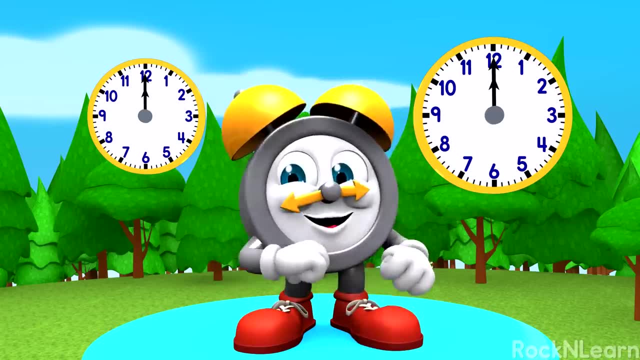 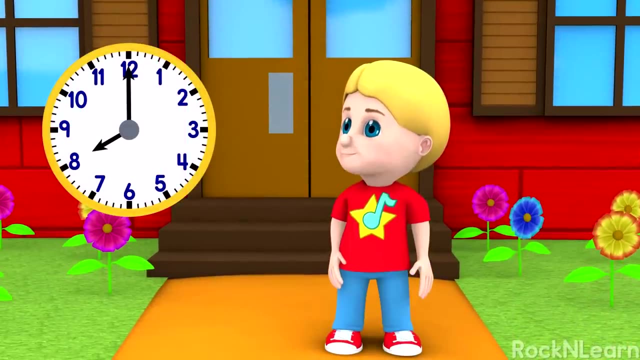 This is twelve am and also twelve midnight. Twelve hours later, it is noon or twelve pm. Let's look at some examples now and join along with them. Eight o'clock am Is the start of my school day. 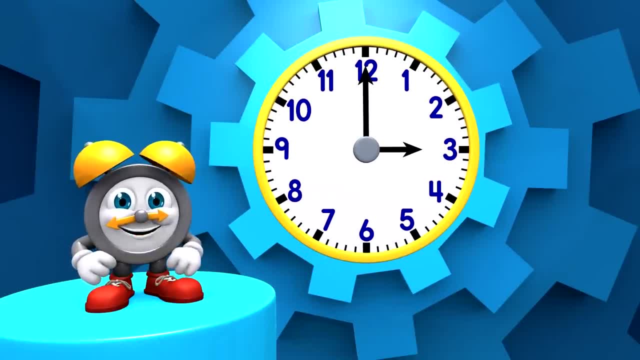 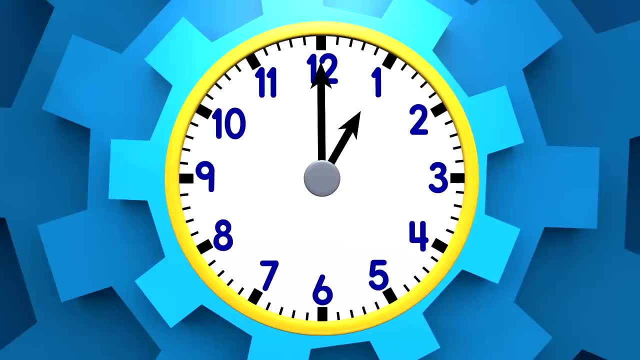 Let's try a few examples. Just take a look at these and say them out loud as quickly as you please. One o'clock, Two o'clock, Three o'clock, Four o'clock, Five o'clock, Six o'clock, Seven o'clock, Eight o'clock, Nine o'clock, Ten o'clock, Eleven o'clock, Twelve o'clock. 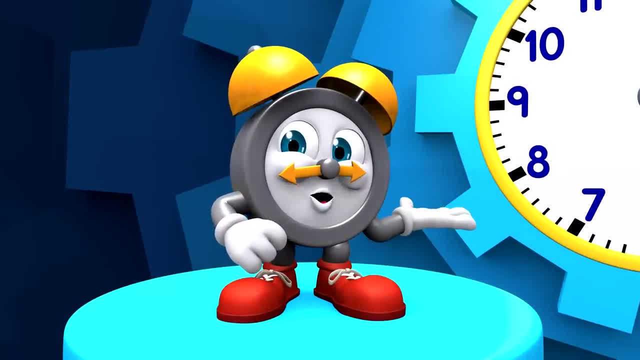 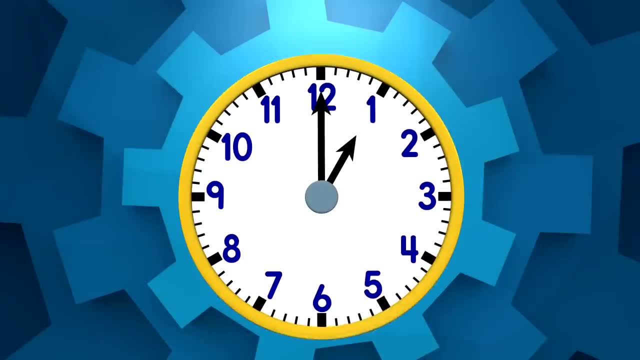 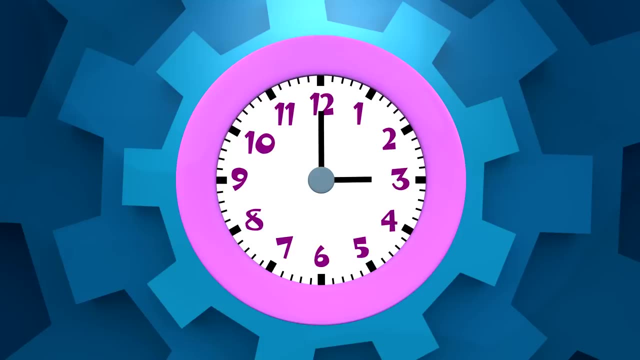 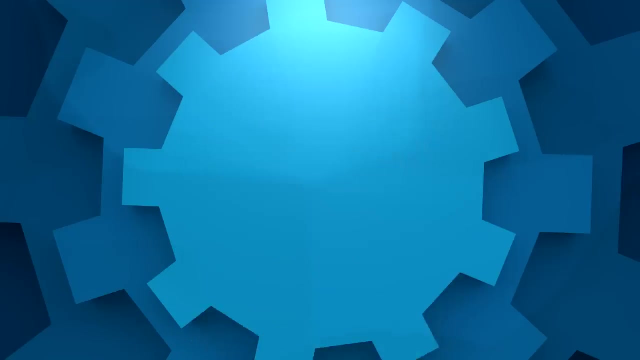 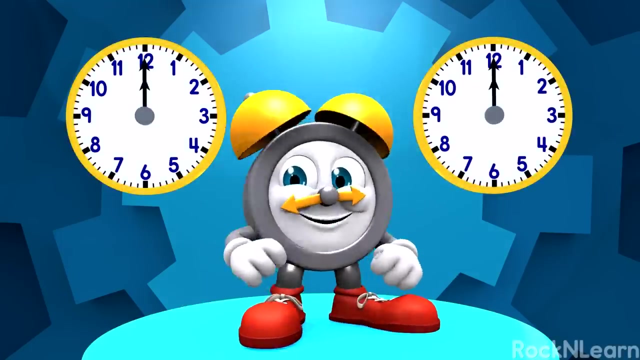 Now let's try some other questions. There are several o'clocks like ones that you might see, So you get some more practice. Say these times with me: One o'clock, Three o'clock, Six o'clock, Eleven o'clock. Some of you have noticed something along the line. 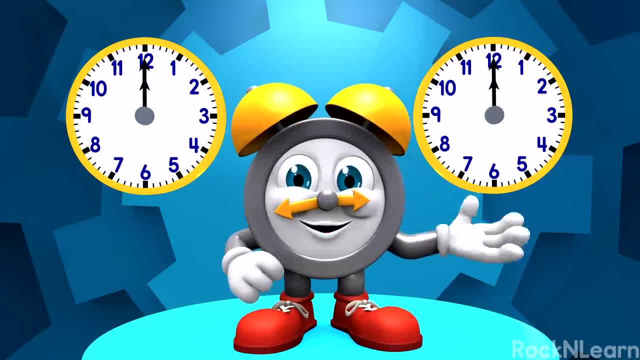 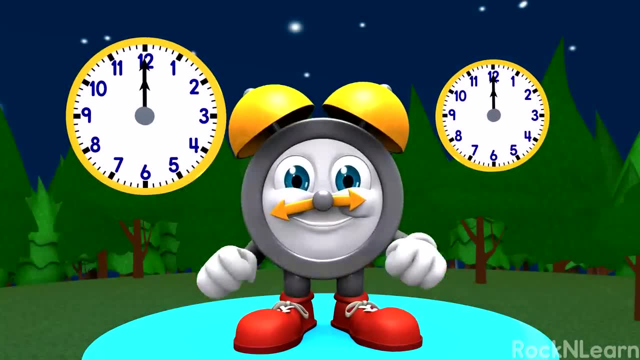 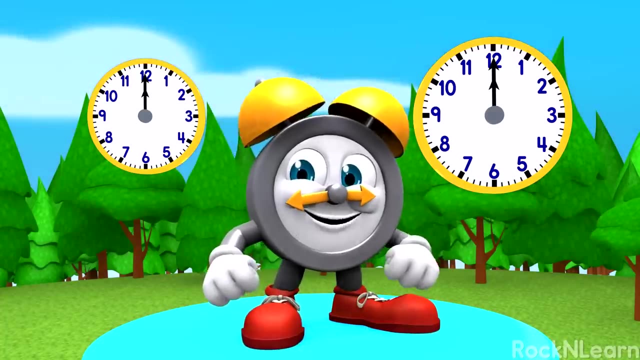 little strange. It seems we have two of each hour in each day. The first, 12 o'clock, comes when it is night. This is 12 am, and also 12 midnight. 12 hours later it is noon or 12 pm. Let's look at. 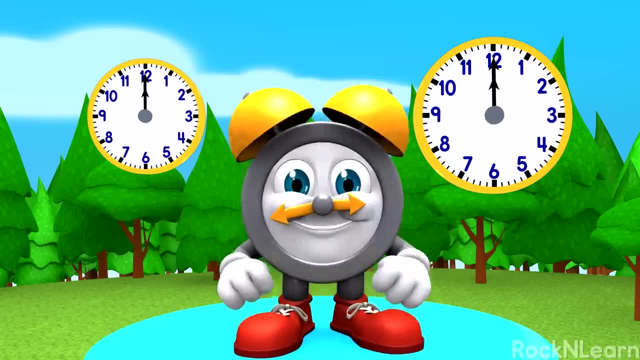 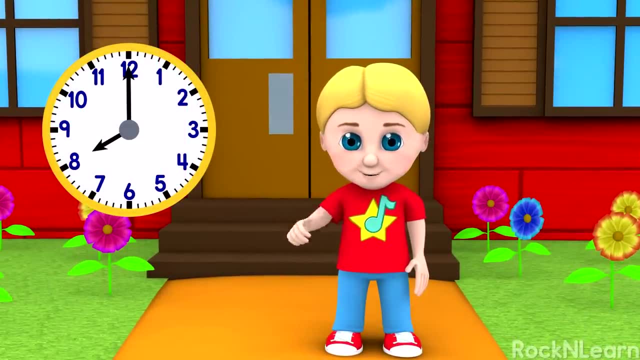 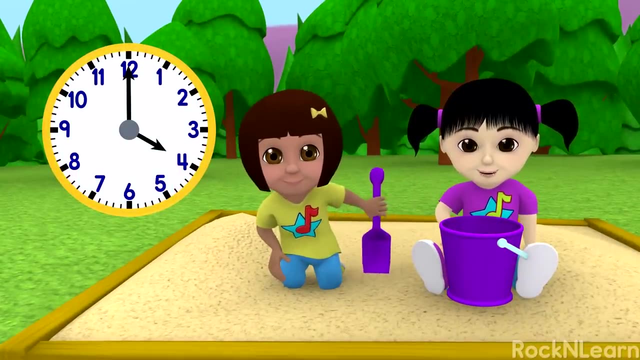 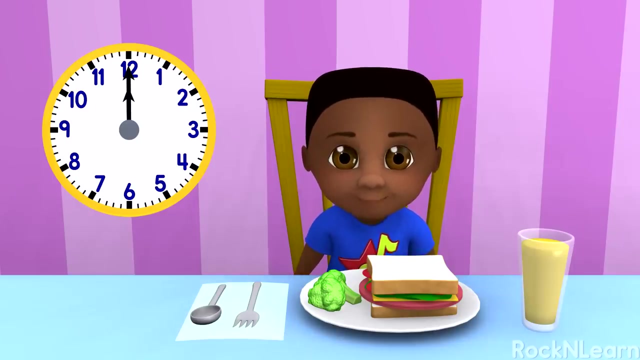 some examples now and join along with them. Eight o'clock am is the start of my school day. Four o'clock pm is the time for friends to play. Twelve o'clock pm is the time to eat some lunch. Seven o'clock pm. 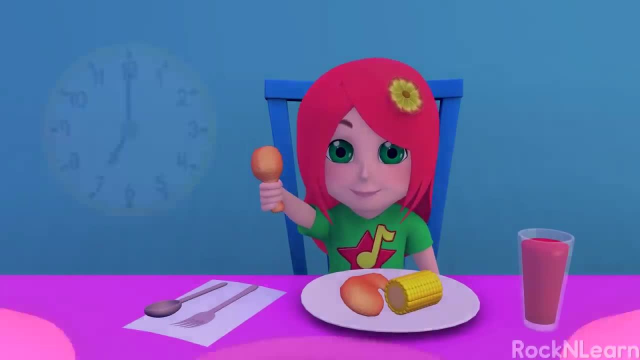 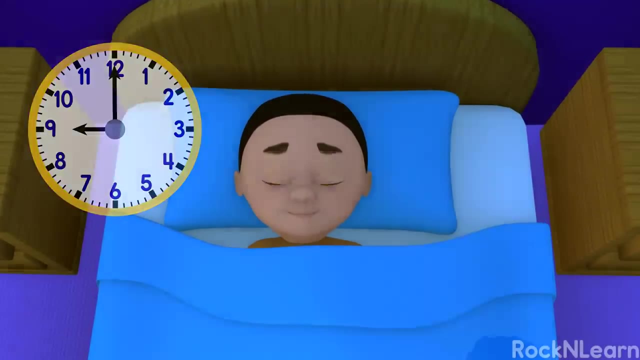 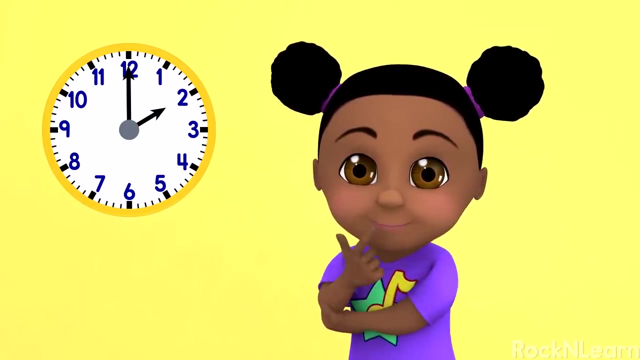 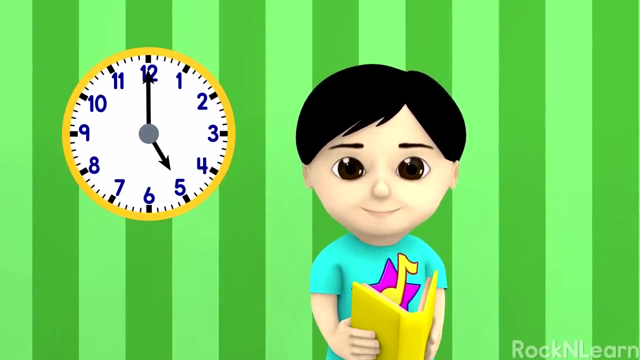 is when my dinner gets munched. Nine o'clock pm is when I need to be in bed. Two o'clock pm is when I think of what my teacher said. Five o'clock pm is when I do homework and chores. Ten o'clock am is when 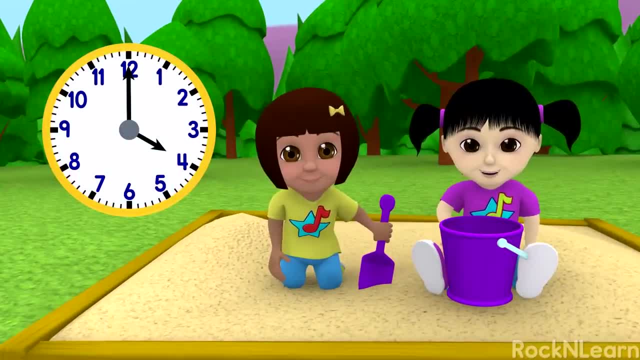 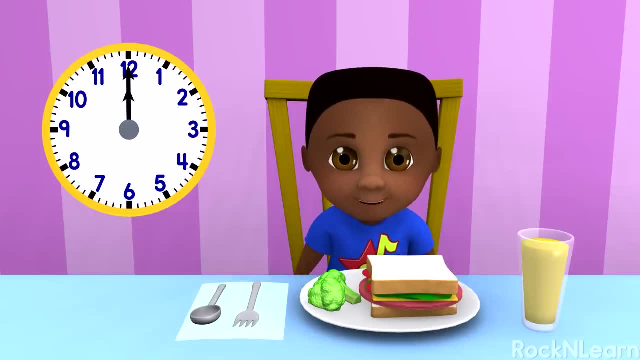 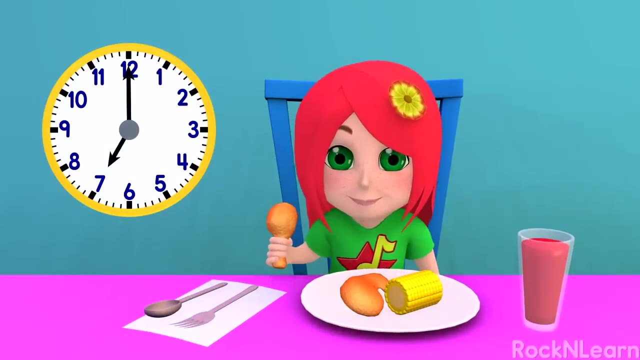 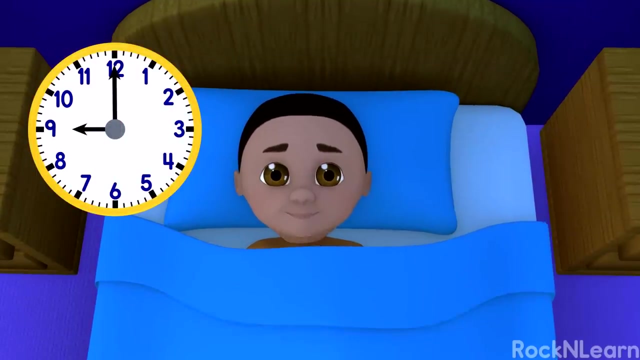 Four o'clock pm Is the time for friends to play. Twelve o'clock pm Is the time to eat some lunch. Seven o'clock pm Is when my dinner gets munched. Nine o'clock pm Is when I need to be in bed. 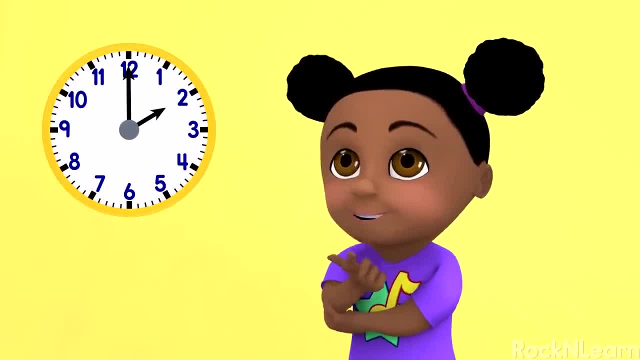 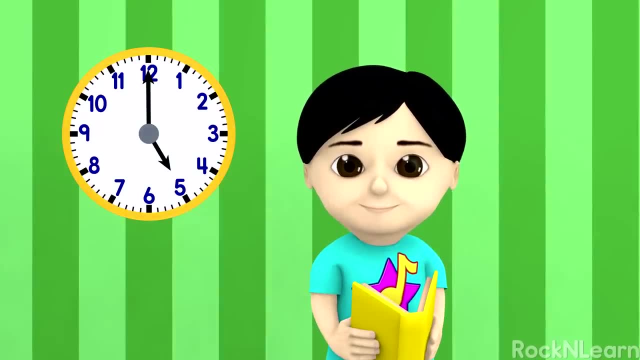 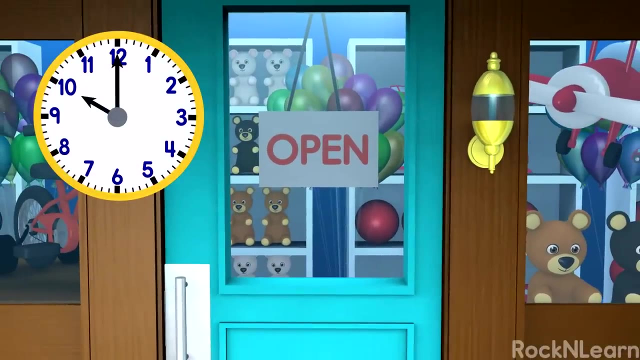 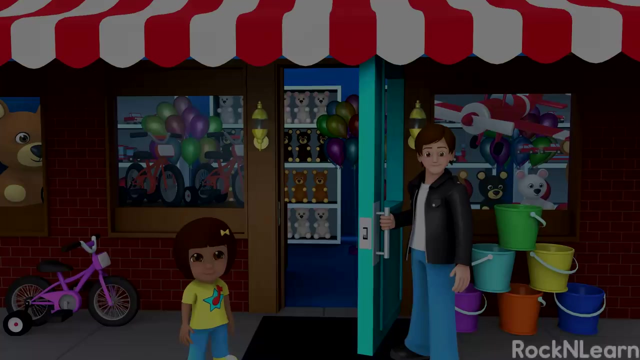 Two o'clock pm Is when I think of what my teacher said. Five o'clock pm Is when I do homework and chores. Ten o'clock am Is when they open most stores. Ten o'clock am Is when I write my homework. 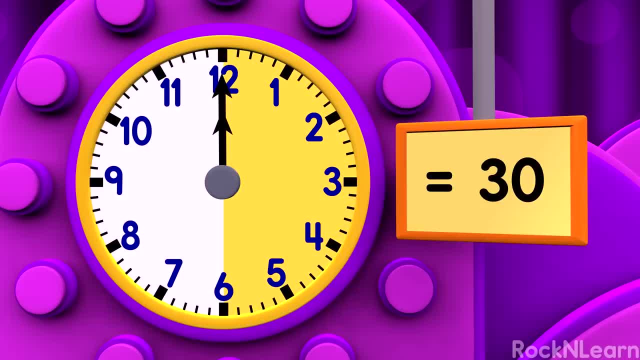 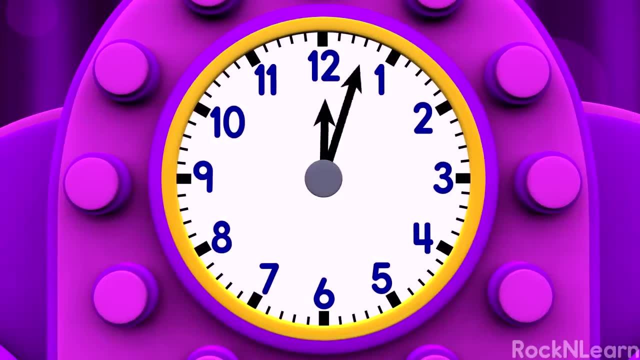 Seven o'clock pm Is when I have to do homework on my own. Twenty o'clock pm Is when I go to the gym. Ten o'clock pm Is when I wake up and see that my teacher is there And that I am not alone. 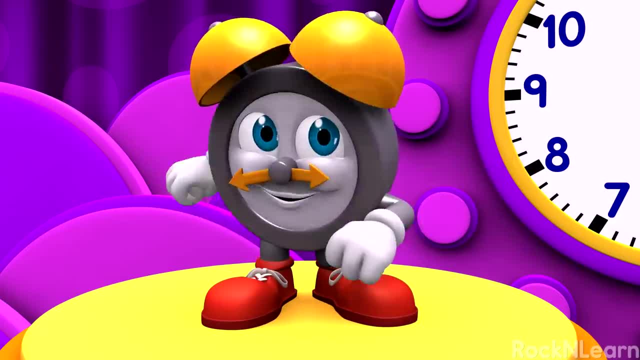 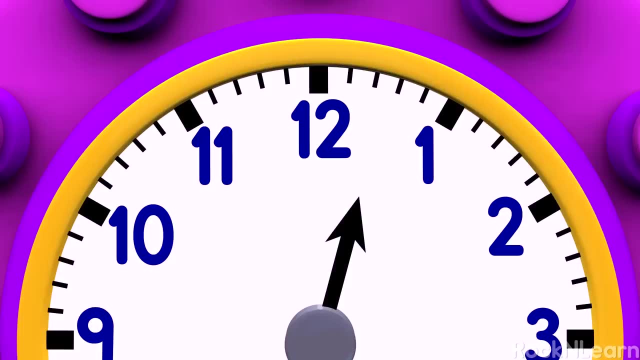 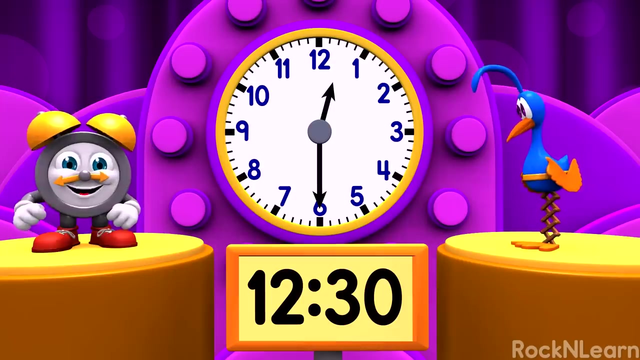 Twelve o'clock pm Is when I am at the gym. It's quite easy. The hour hand will be halfway in between two of the numbers, somewhere around the ring. Whichever of the numbers the hour hands just passed is the one you say out loud, with 30 at the last. 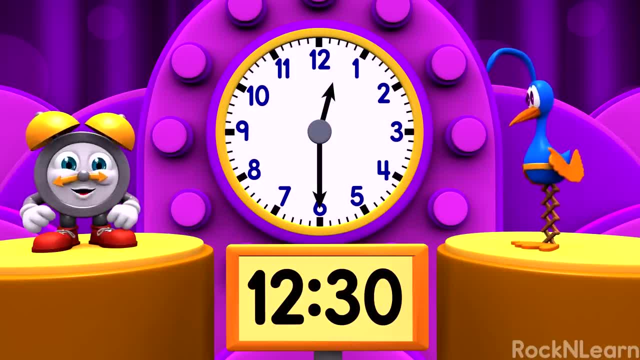 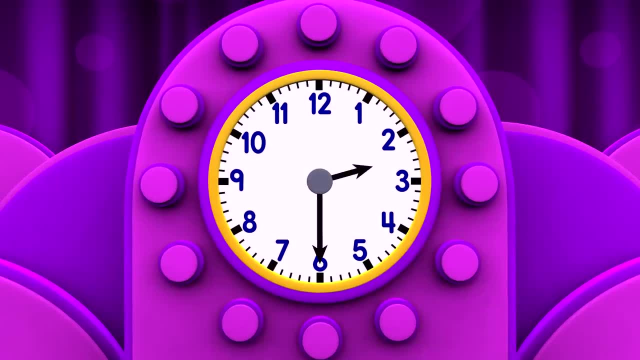 Well then, show us how to do it. Okay, don't get your feathers ruffled. 1.30, 2.30, 3.30, 4.30, 5.30, 6.30, 7.30, 8.30. 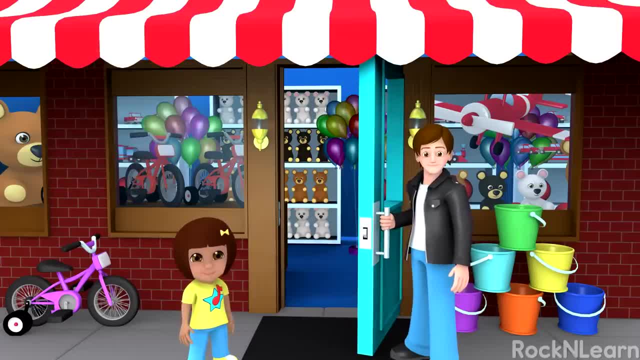 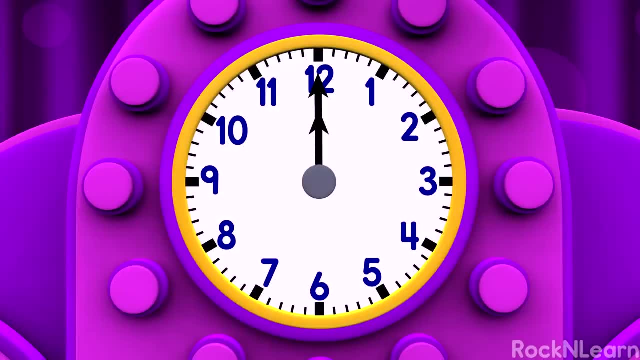 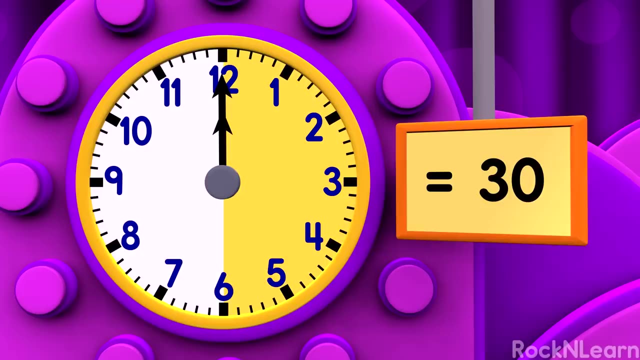 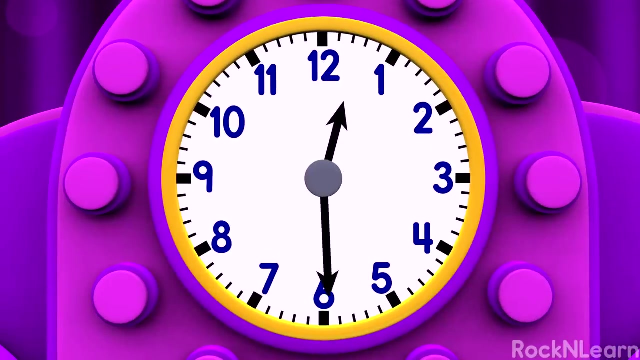 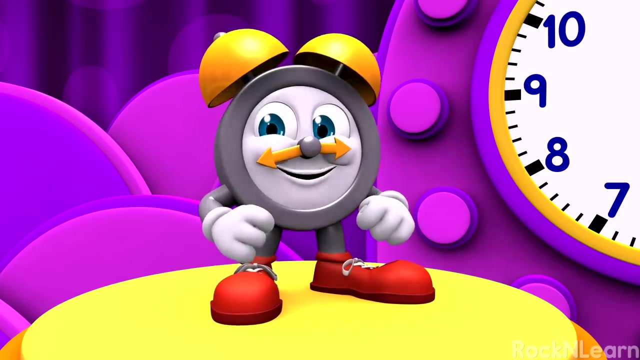 Then they open most doors. Since one whole hour has sixty minutes, half an hour has only thirty minutes in it. If you start on the hour and go halfway around, the minute hand will be on the six hanging upside down. Now you might ask where will the short hand be? 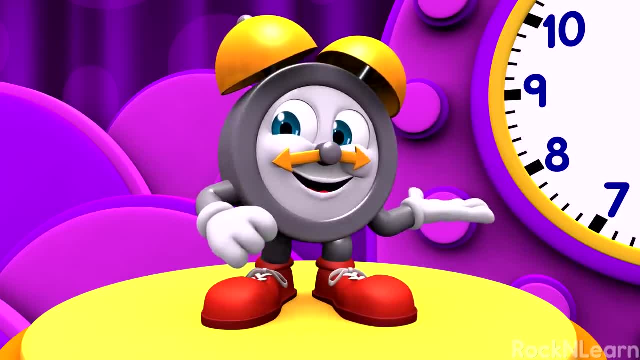 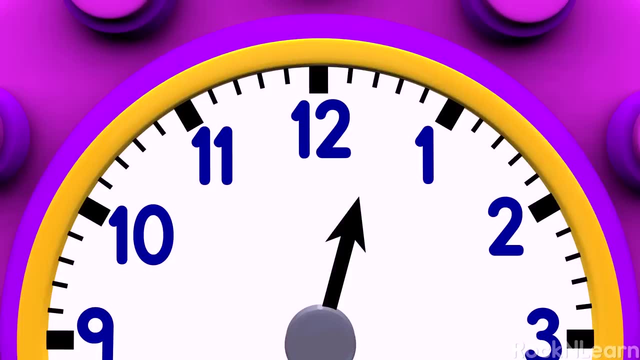 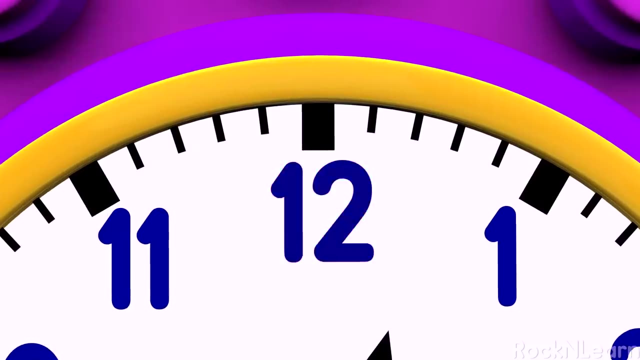 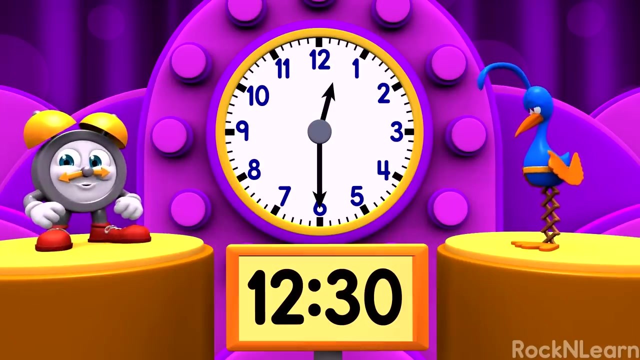 I can tell you now. it's quite easy. The hour hand will be halfway in between two of the numbers, somewhere around the ring. Whichever of the numbers the hour hand's just passed is the one you say out loud With thirty at the last. 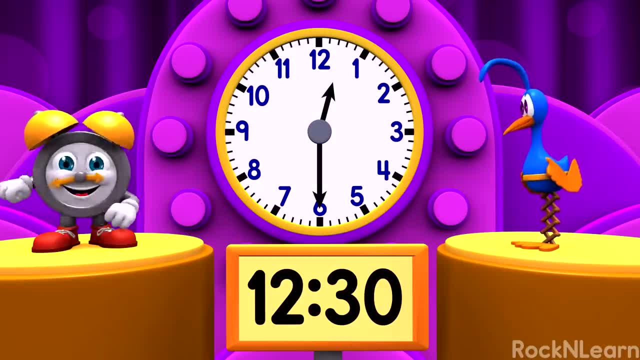 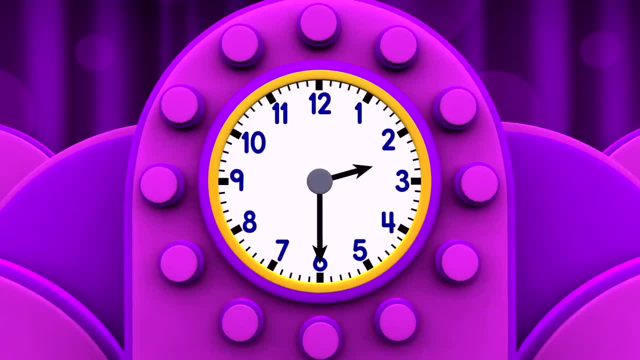 Well then, show us how to do it. Okay, don't get your feathers ruffled. One, thirty Two, thirty Three, thirty Four, thirty Five, thirty Six, thirty Five, thirty Six, thirty Seven, thirty Eight, thirty Nine, thirty. 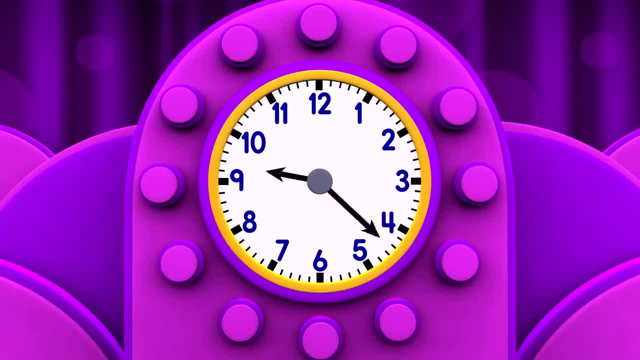 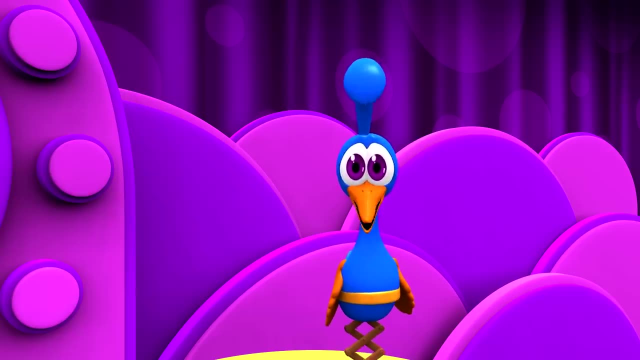 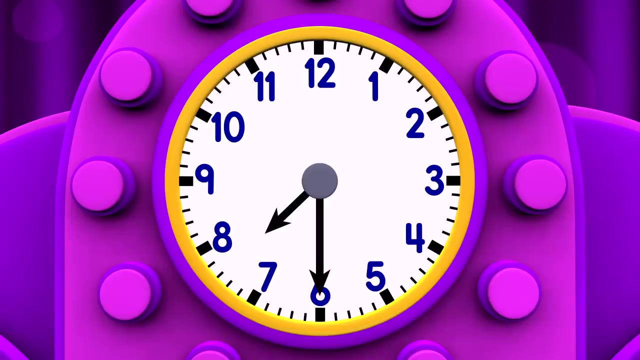 Ten, thirty, Eleven, thirty, Twelve, thirty. Okay, Timothy. so when I hear people say it's half past seven, does that mean that the minute hand is on the six and that it's seven thirty? Wow, Cuckoo. 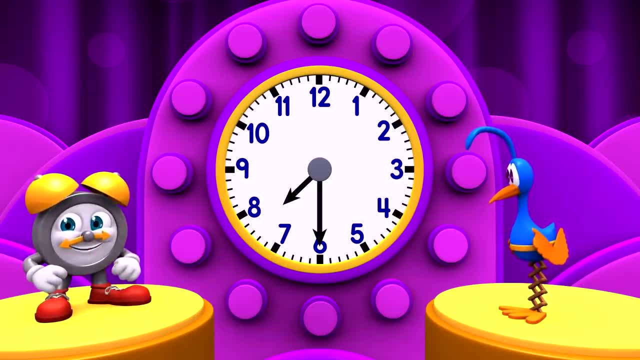 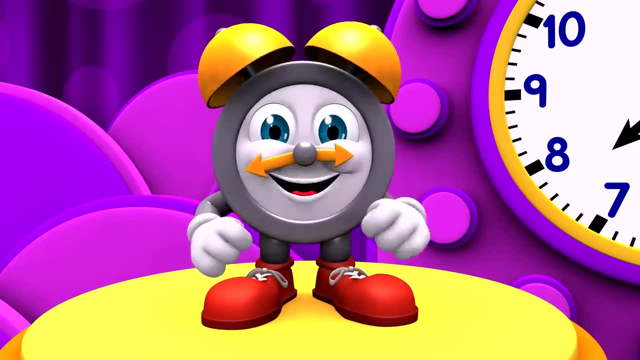 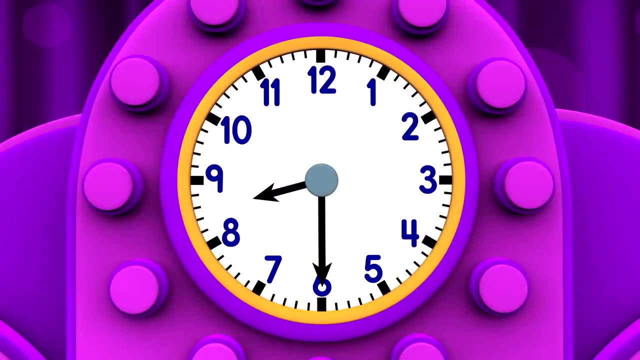 You catch on really fast. They say half past because the hour hand has traveled halfway past the number before it. Let's look at some more clocks. Read the times on these clocks with me: Eight, thirty or half past eight Twelve o'clock. 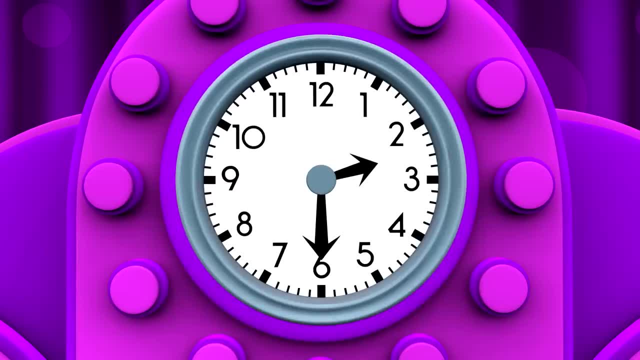 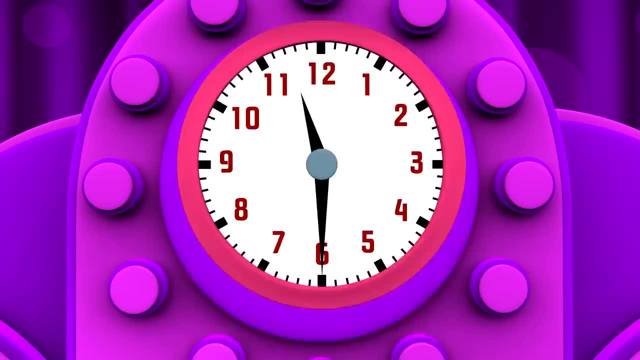 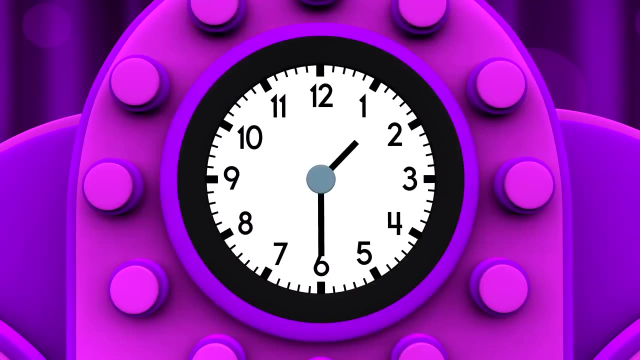 Two, thirty or half past two. Twelve o'clock Two. thirty or half past two. Eleven, thirty or half past ten. Eleven, thirty or half past eleven. Nine o'clock Nine o'clock One, thirty or half past one. 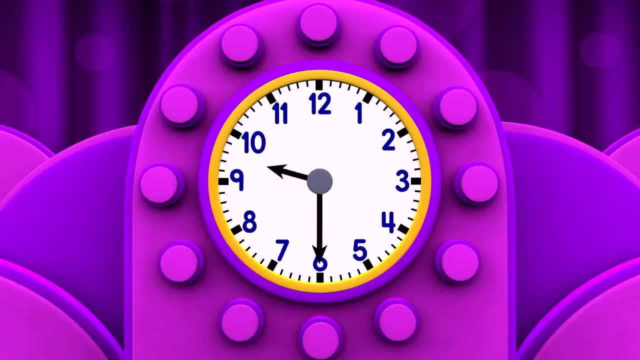 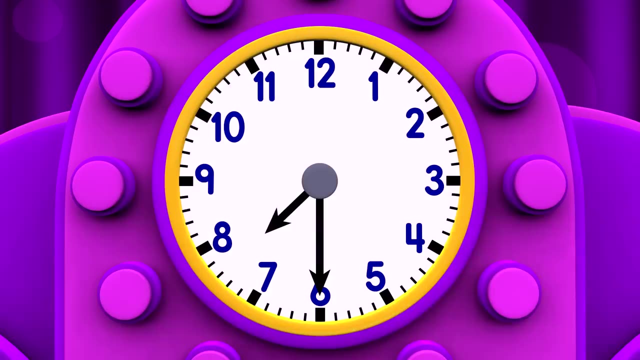 9.30, 10.30, 11.30, 12.30. Okay, Timothy, so when I hear people say it's half past 7,, does that mean that the minute hand is on the 6 and that it's 7.30?? 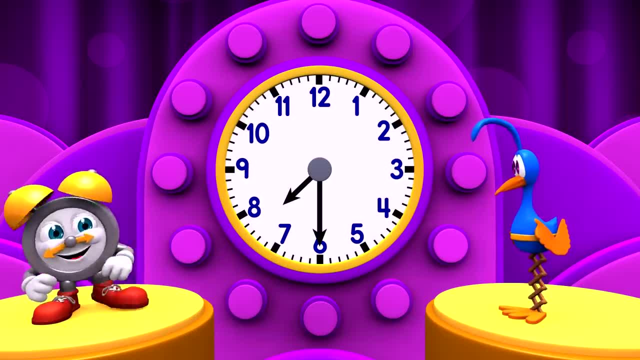 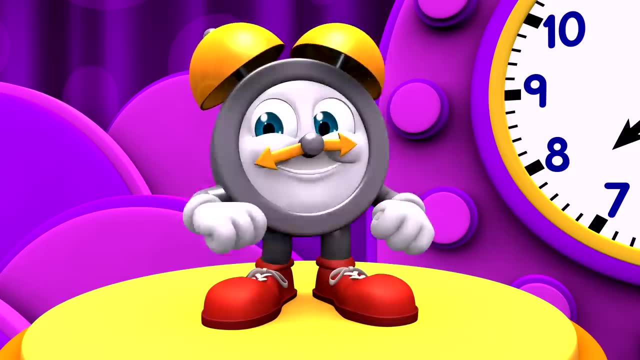 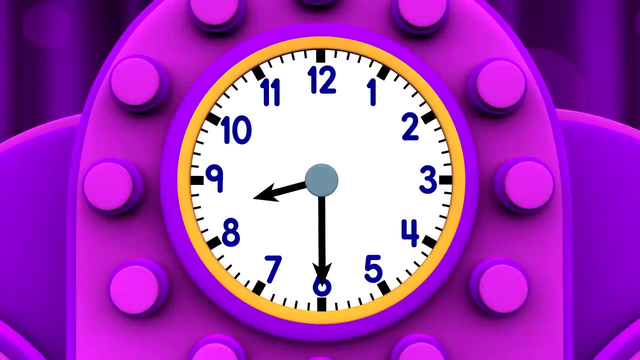 Wow, Cuckoo, you catch on really fast. They say half past because the hour hand has traveled halfway past the number before it. Let's look at some more Four clocks. Read the times on these clocks with me: 8.30 or half past 8.. 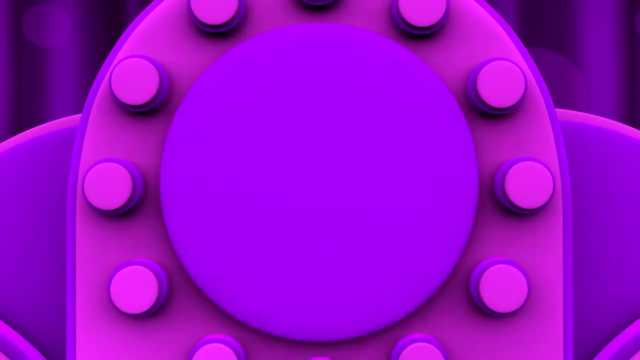 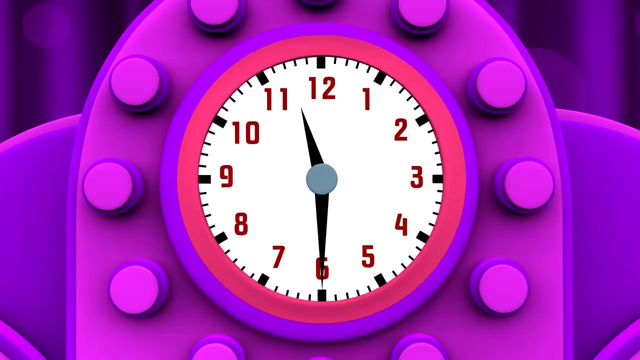 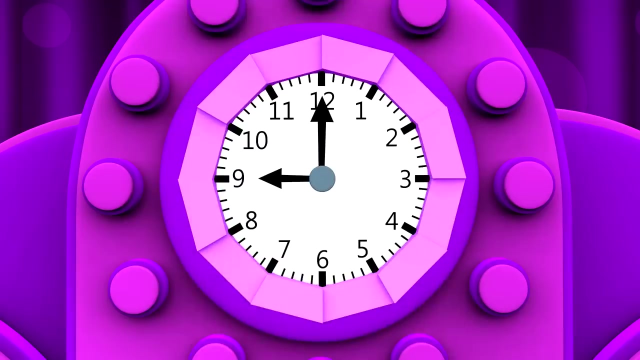 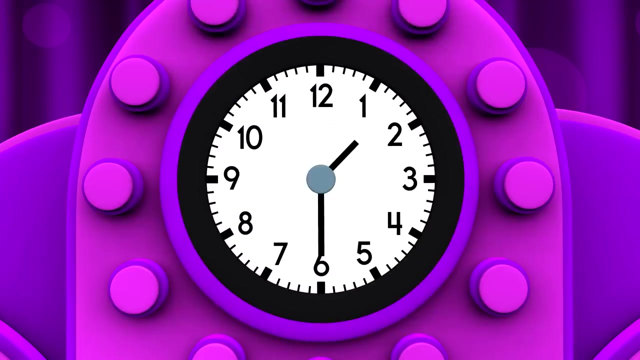 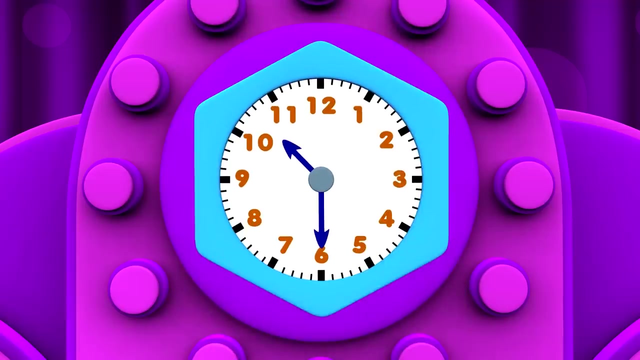 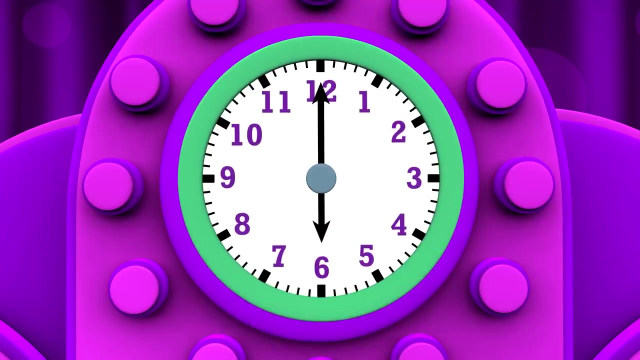 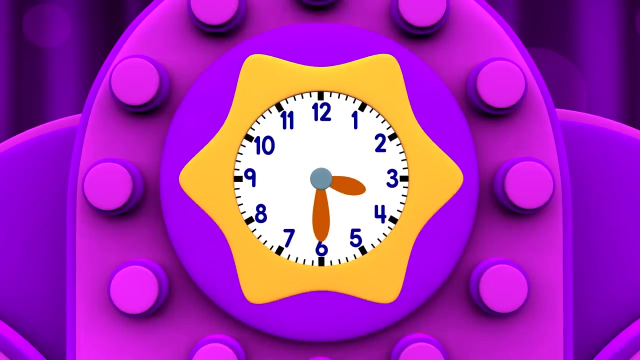 12 o'clock. 2.30 or half past 2.. 11.30 or half past 11. 9 o'clock. 10.30 or half past 10.. 3.30 or half past 3. 9 o'clock. 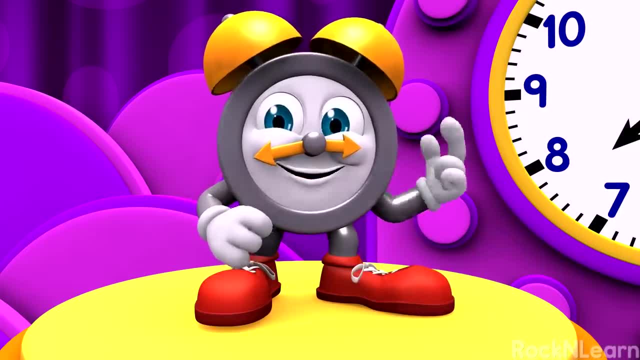 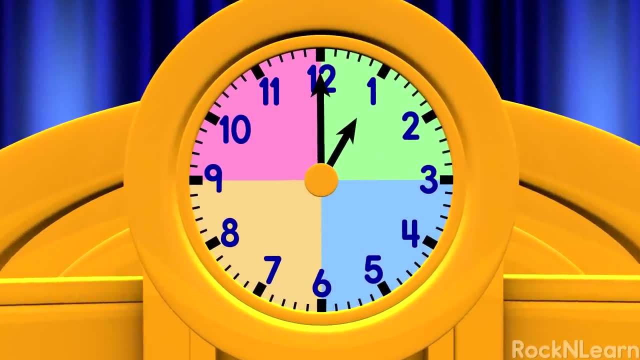 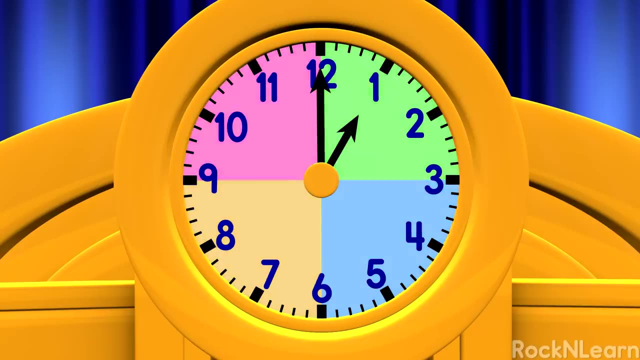 10.30 or half past 10.. adas't my number: 3.30 or half past 10.. using your brain power telling time to the half hour, this clock face has been divided into four, that's four equal sections. now let me tell you more. if the 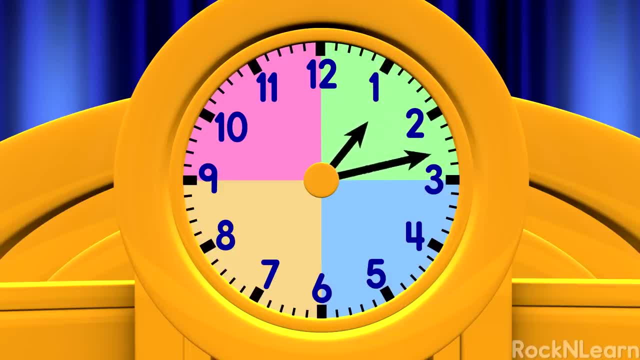 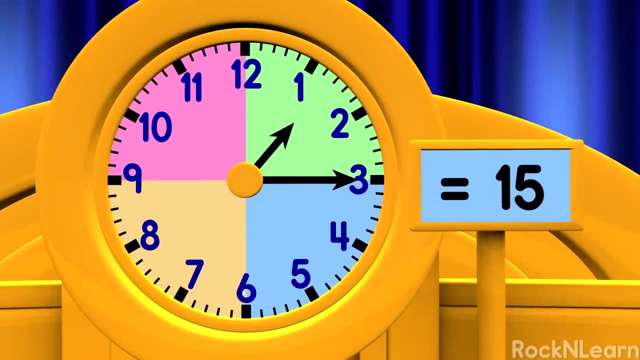 minutes hand has gone just a quarter of the way. it's a quarter past the hour. a quarter past is what you say, at a quarter past. the minute hand is on the three and the number of the minutes past the hour is 15. the hour hand will be 1. 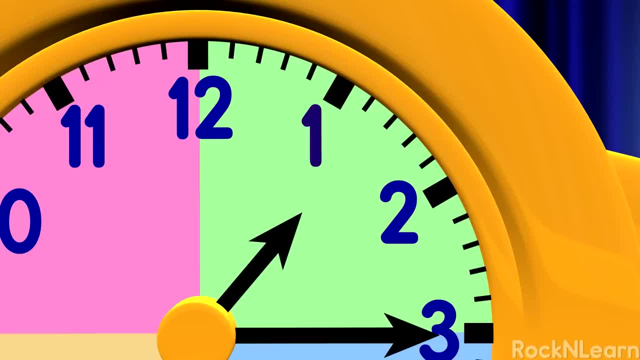 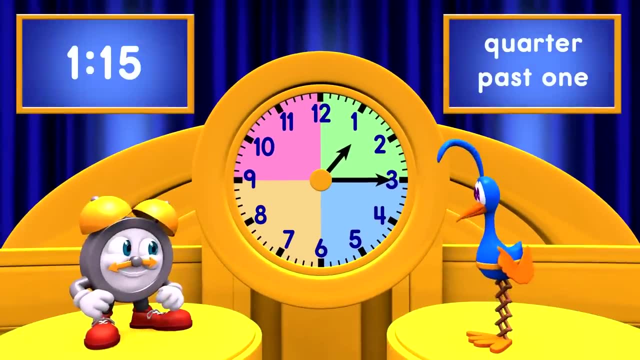 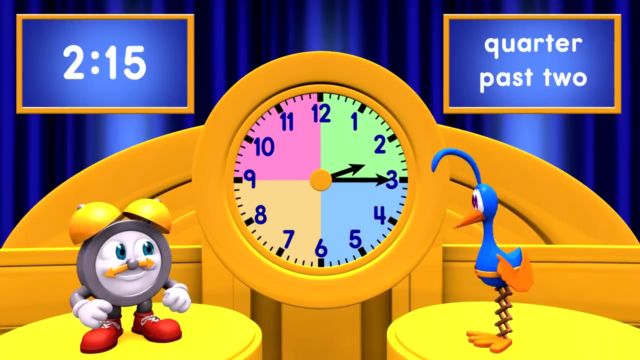 fourth, of the way, past one of the numbers. this numbers what you'll say: one, 15 or a quarter past one. we can say it either way. telling time can sure be fun. to 15 or a quarter past 2. we're learning to tell time, it's. 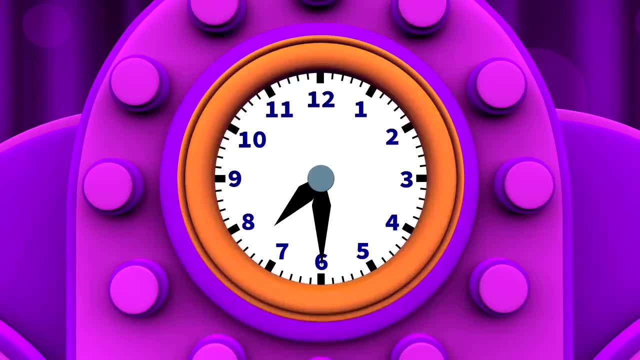 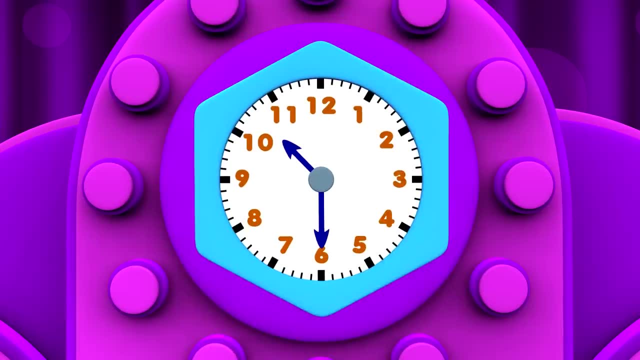 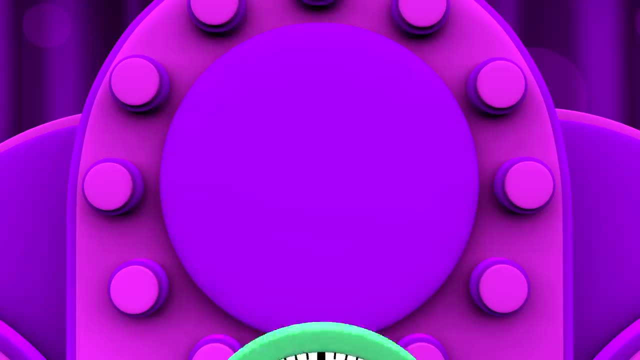 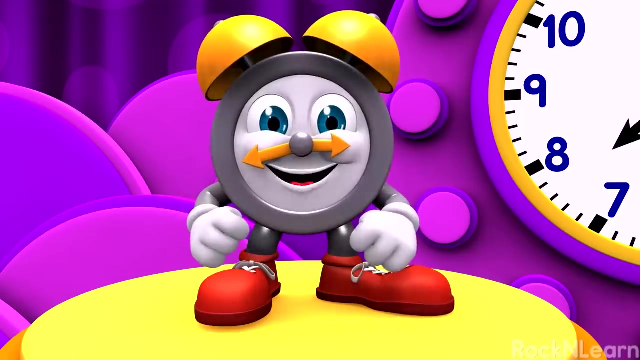 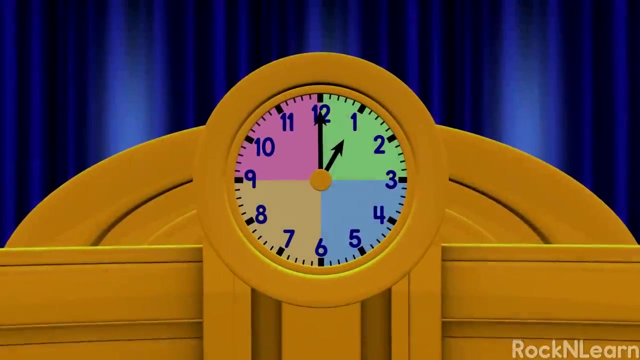 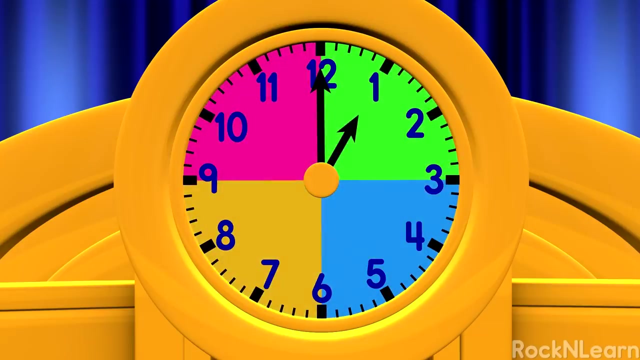 The first time. Seven thirty or half past seven, Ten thirty or half past ten, Six o'clock, 3.30, or half past three. Now you're using your brain power telling time to the half hour. This clock face has been divided into four. 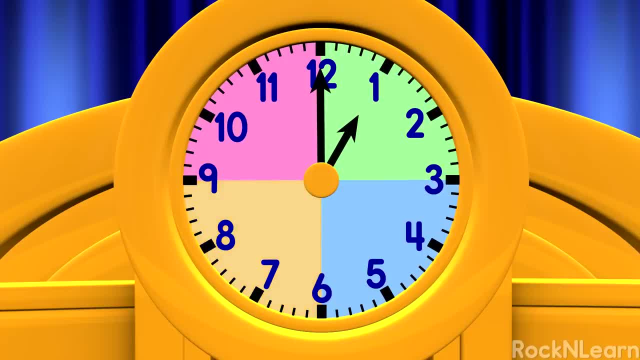 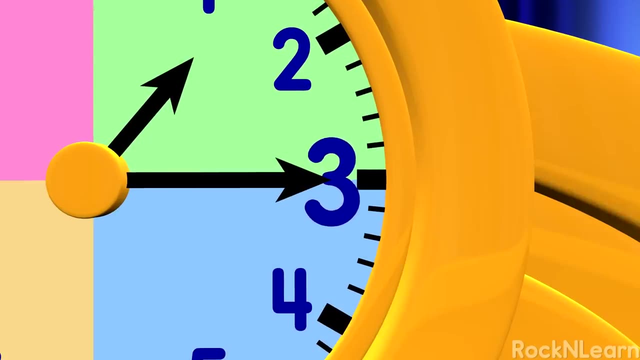 That's four equal sections. Now let me tell you more. If the minute hand has gone just a quarter of the way, it's a quarter past the hour. A quarter past is what you say At a quarter past. the minute hand is on the three and the number of the minutes past the hour is 15.. 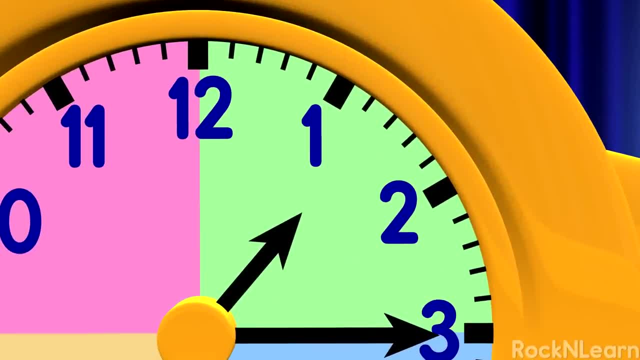 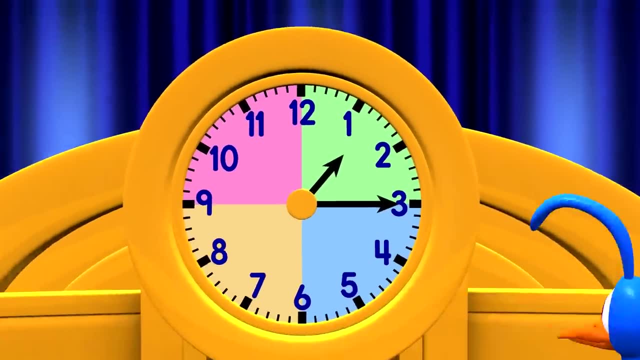 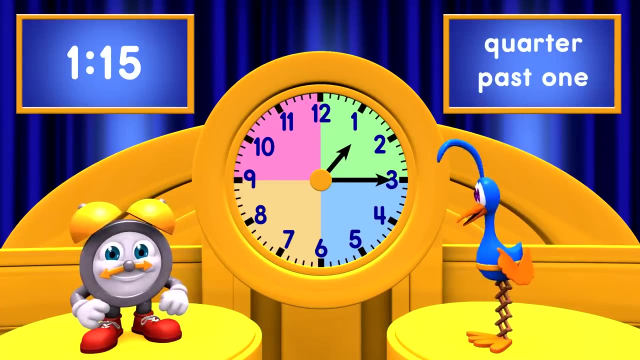 The hour hand will be one-fourth of the way past one of the numbers. This number's what you'll say: One-fifteen or a quarter past one, We can say it either way. Telling time can sure be fun. 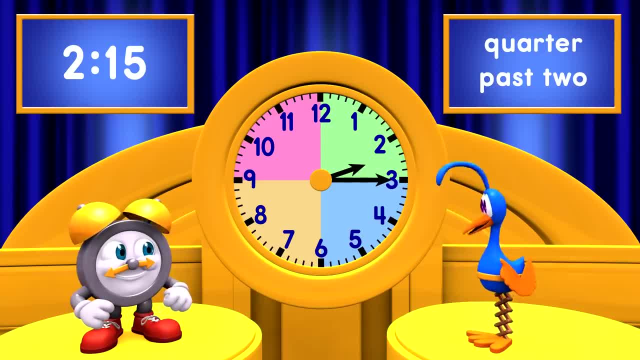 Two-fifteen or a quarter past two. We're learning to tell time, It's easy with you. Oh, thank you, Cuckoo. Three-fifteen or a quarter past three. Three-fifteen or a quarter past three. 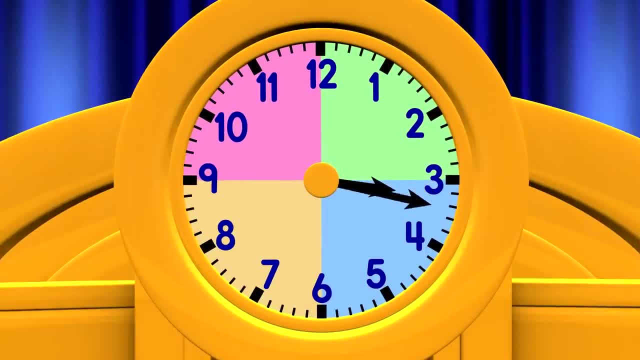 I think I've got it now Sounds good to me. Now, when the minute hand has moved another quarter of the way, it's half past the hour. Oh, we've learned that. Okay, Four-thirty or half past four. 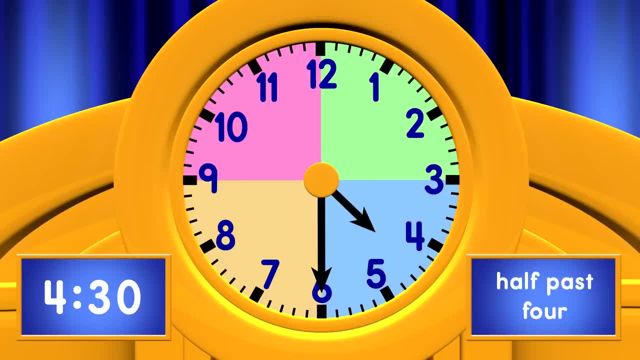 Four-thirty or half past four. I remember this. Let's do a couple more. Let's do a couple more. Five-thirty or half past four. Five-thirty or half past four. Five-thirty or half past five. 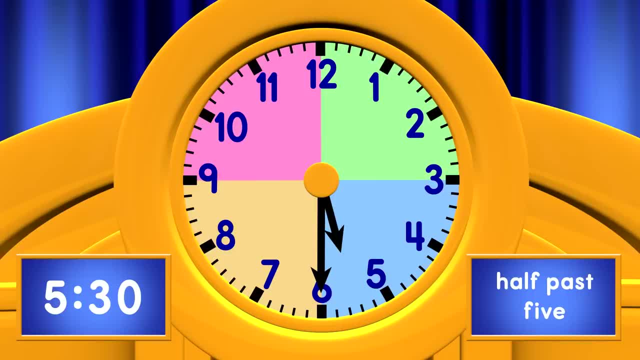 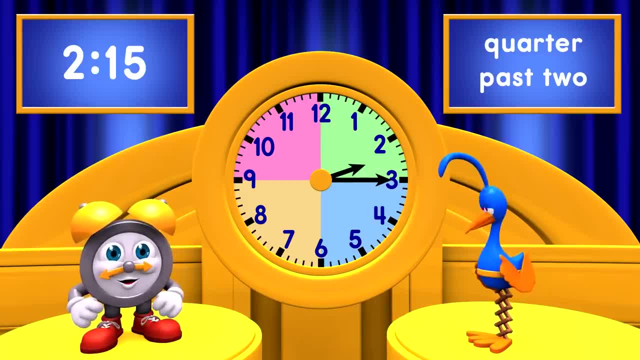 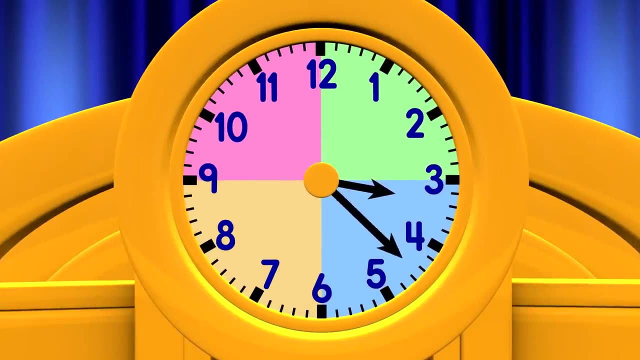 easy with you. oh, thank you, cuckoo. 15 or a quarter past 3 sounds good to me. now, when the minutes hand has moved another quarter of the way, it's half past the hour. oh, we've learned that. okay, 430 or half past 4. I remember this. let's do a couple. 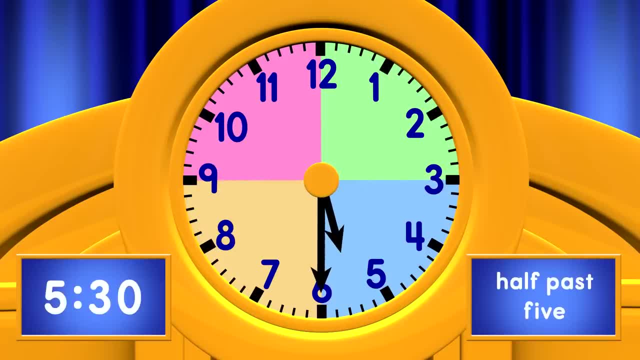 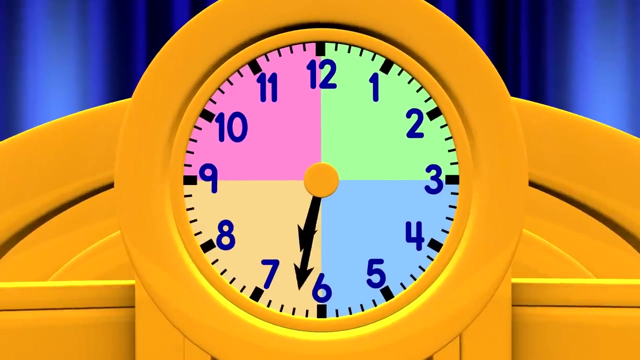 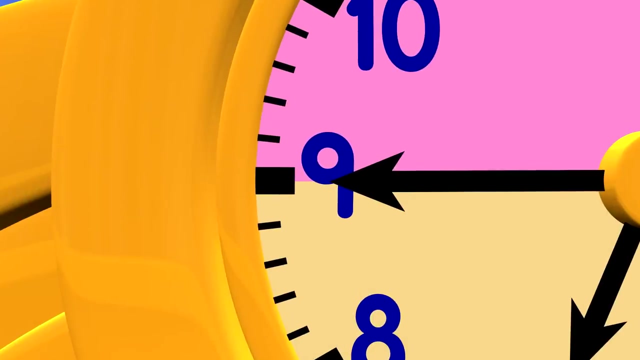 more. 530 or half past 5. I think you've really got it. yeah, give me 5 OME. let's learn something new. okay, do 630. or half past 6. let's learn something new. okay, I'll teach you some more tricks. let's keep on moving another quarter of an hour, so it's just a quarter till the very next hour. the minutes hand will be pointing to the 9. the minutes that have passed equal 45. the hour hand has point clear. 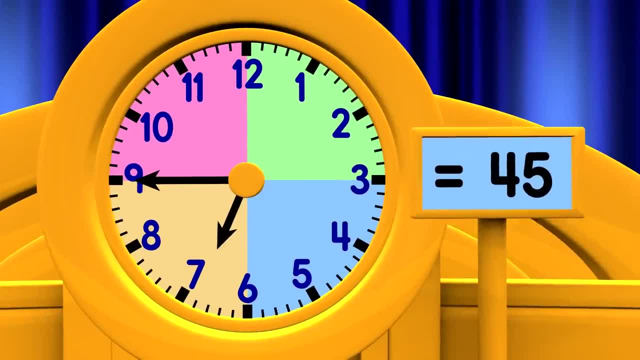 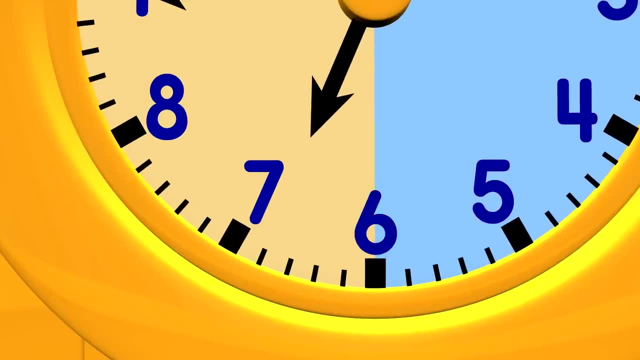 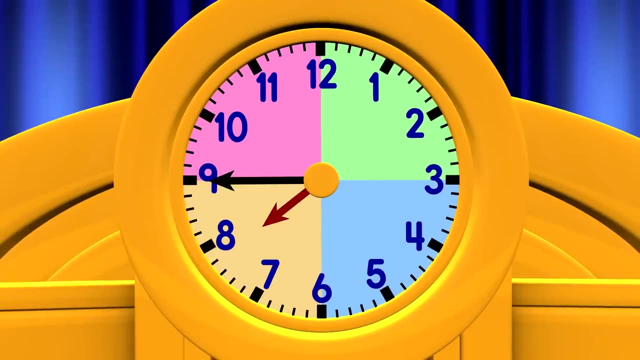 cloudy sky, sky as past the hour, three quarters of the way. so look back to the number that you are going to say. take a look at this one. the hour hand is almost at the eight, so we go back to the seven to get the hour straight. now the minute hand is on the nine. 45 minutes have passed, so it's 7: 45. 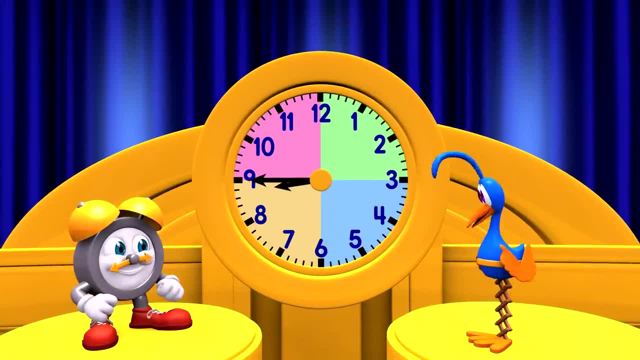 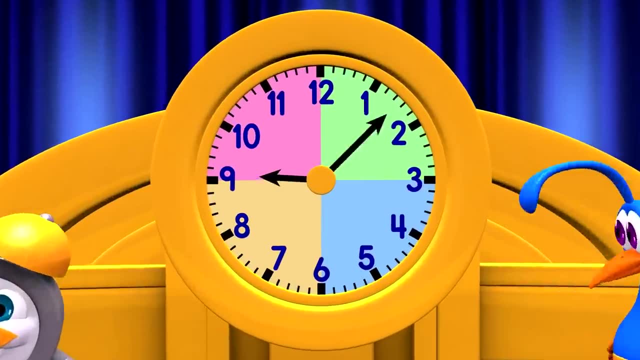 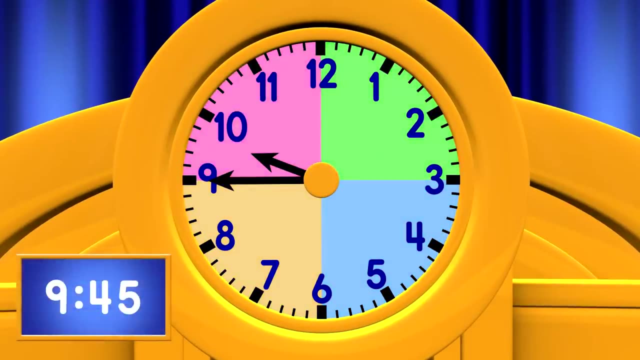 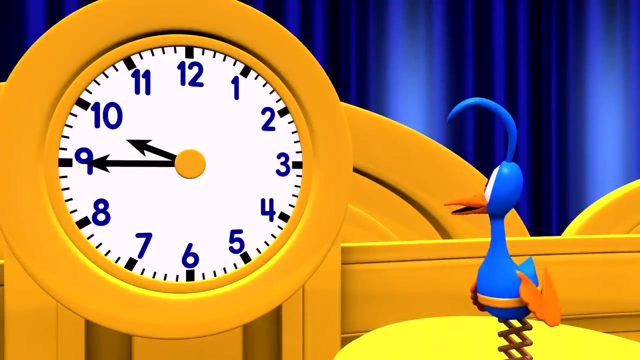 let me see the hour hand is almost to the nine, so i go back to the eight. it's 8: 45.. and this one is 9: 45. that's right, hey, timothy time. this was the time on the clock when someone told me. 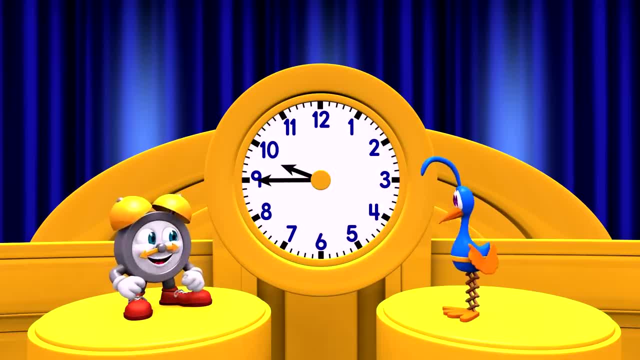 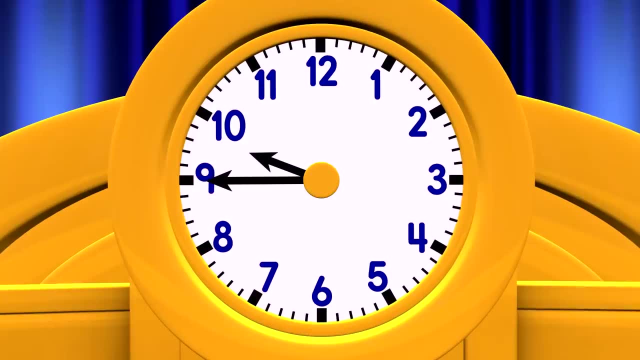 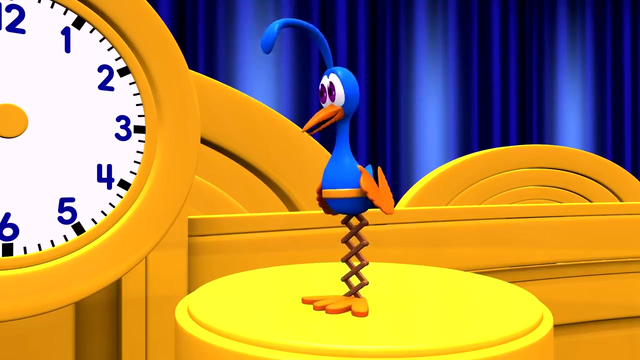 it was a quarter till ten. well, cuckoo, that's another way of looking at this time. instead of going back to the hour that's behind and adding 45 minutes, you look up ahead to the next hour number and say quarter two instead. can i do some by myself? so i'm sure i've got this right. sure, cuckoo, you're in the time spotlight. 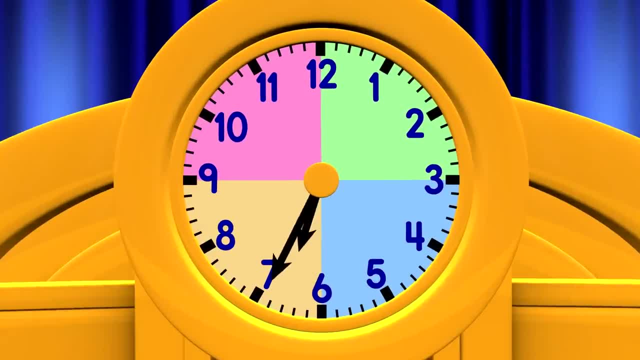 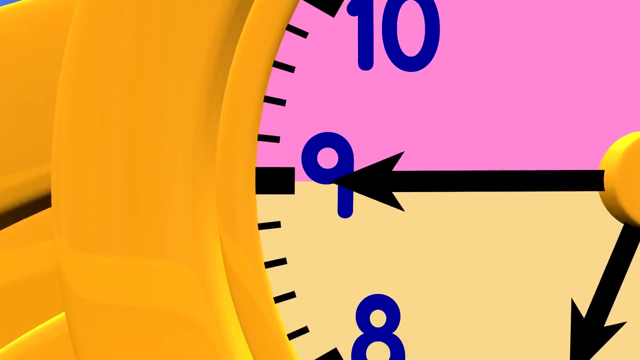 Okay, I'll teach you some more tricks. Let's keep on moving another quarter of an hour, So it's just a quarter till the very next hour. The minute hand will be. The minute hand will be to the 9. the minutes that have passed equal 45. the hour hand has passed the. 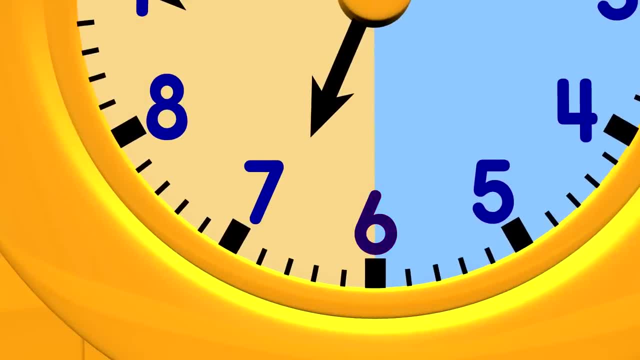 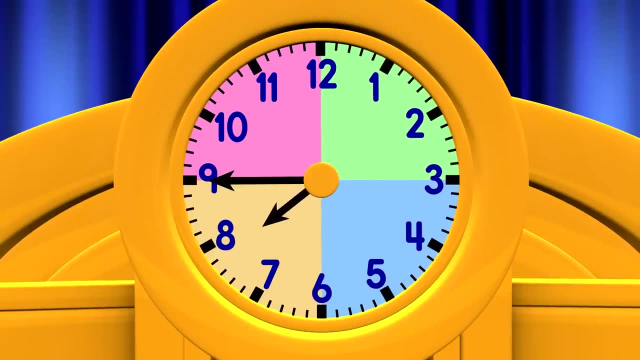 hour 3 quarters of the way. so look back to the number that you are going to say. take a look at this one. the hour hand is almost at the 8, so we go back to the 7 to get the hour straight. now the minute hand is on the 9. 45 minutes have passed. 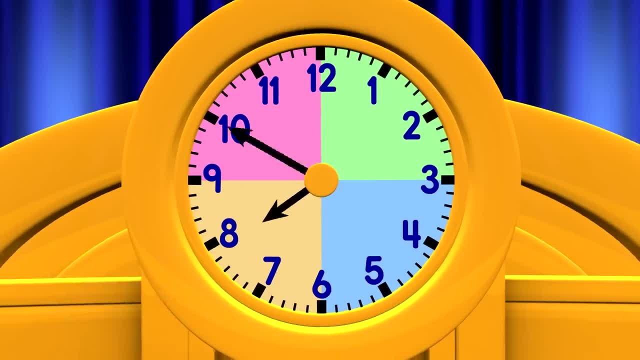 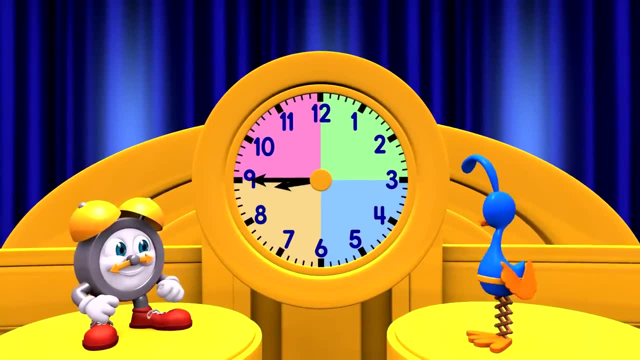 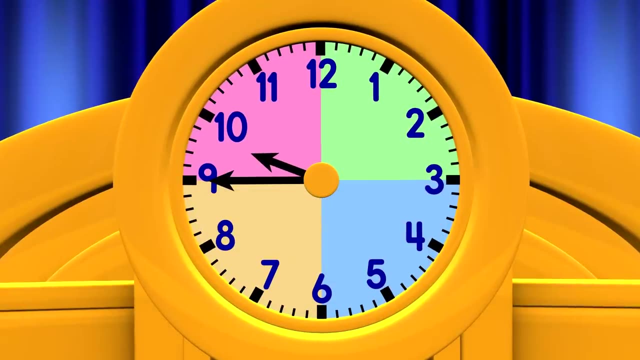 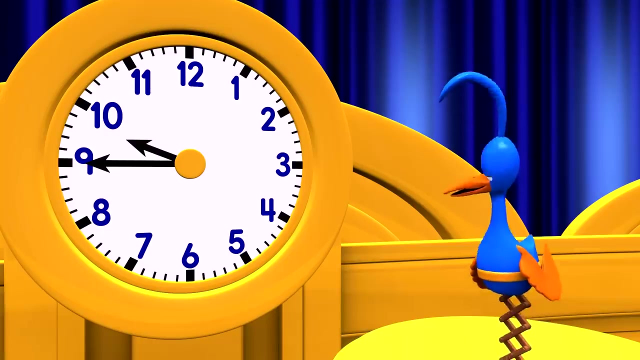 so it's 745. let me see, the hour hand is almost to the 9, so I go back to the 8, and this one is 945. that's right, hey, Timothy time. this was the time on the clock when someone told me it was a quarter to 10. well, cuckoo, that's another way of looking at. 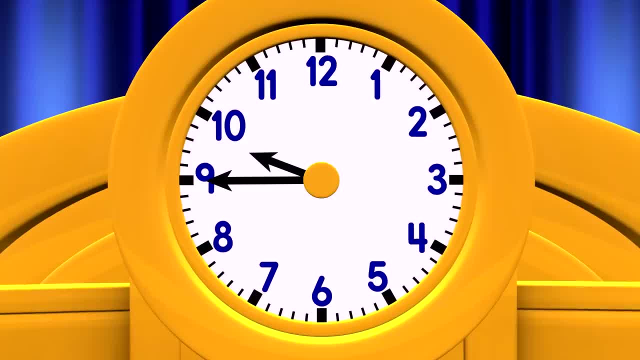 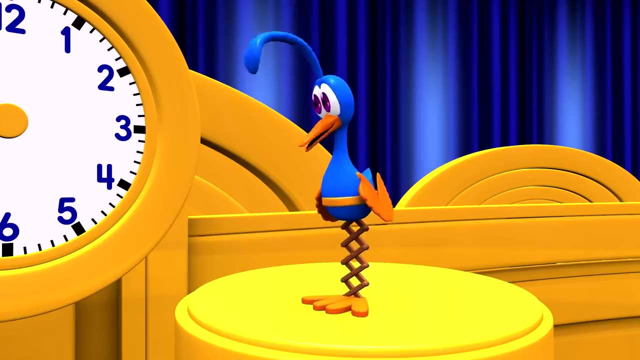 this time, instead of going back to the hour that's behind and adding 45 minutes, you look up ahead to the next hour number and say quarter 10 to instead. can I do some by myself? so I'm sure I've got this right, sure, cuckoo. 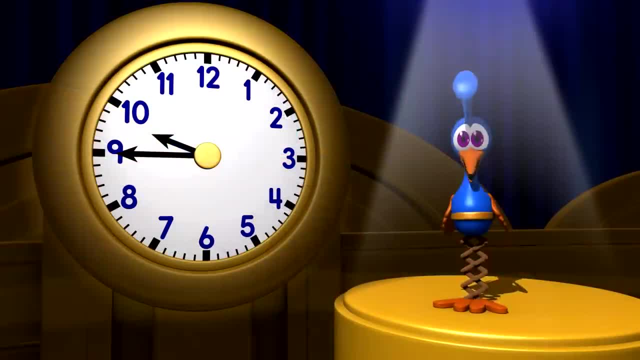 you're in the time spotlight. okay, if I want to look at the hour that's already passed, this is 10: 45. but if I want to look at the hour that is coming, this is a quarter till 11, and this time can be either 1245 or a quarter till one. 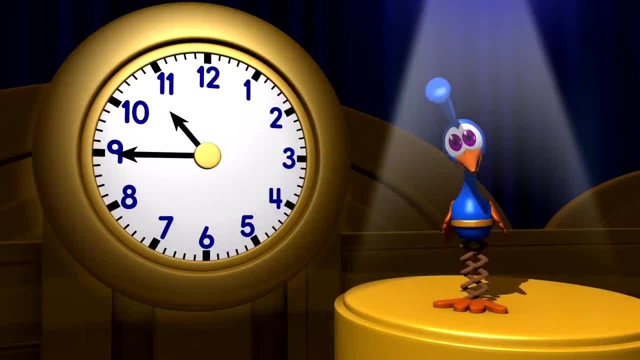 okay, if i want to look at the hour that's already passed, this is 10: 45.. but if i want to look at the hour that is coming, this is a quarter till 11.. and this time can be either 12: 45 or a quarter till one. 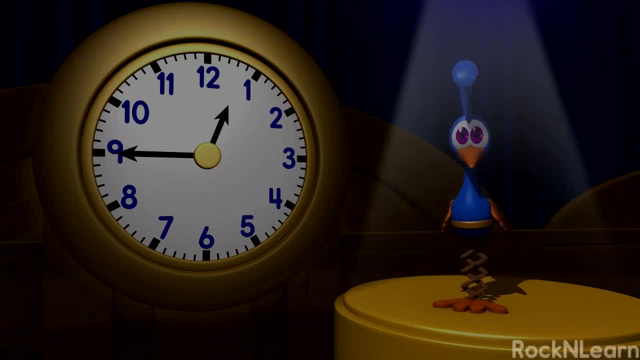 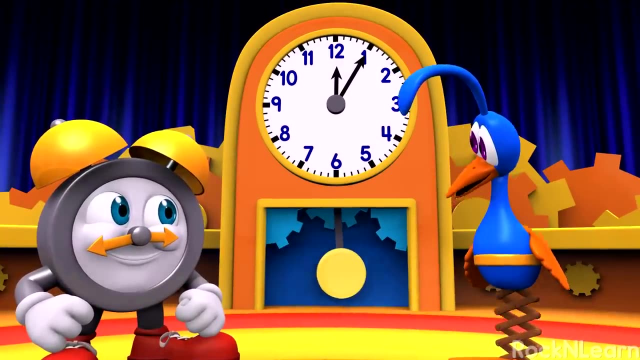 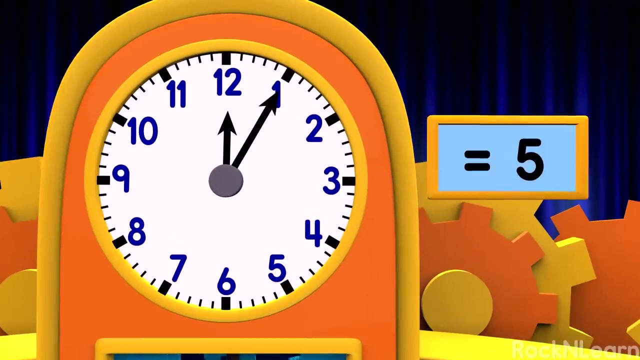 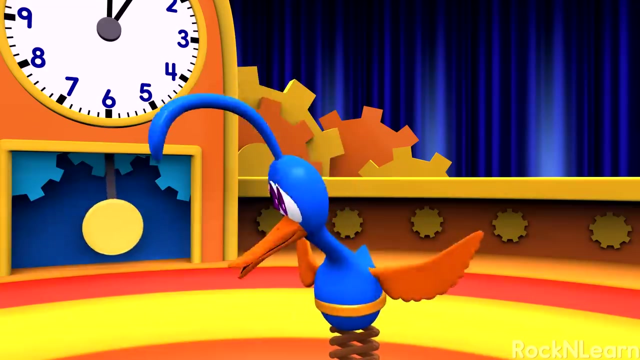 thank you. thank you, hey, timothy time. what happens if the minute hand is on one of the other numbers? well, cuckoo. every time the minute hand is on a number, five minutes have passed. do you know how to count by fives all the way to 60? cuckoo, cuckoo. yeah, and i know why we have to count by fives up to 60.. 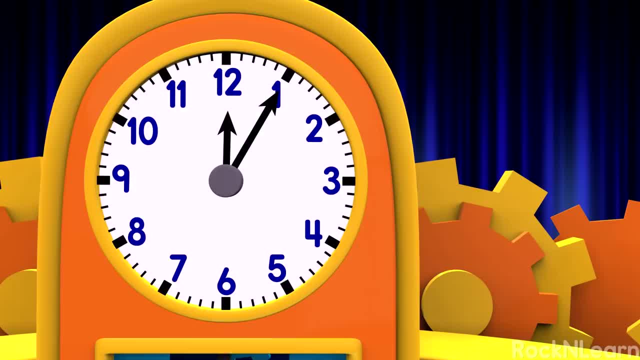 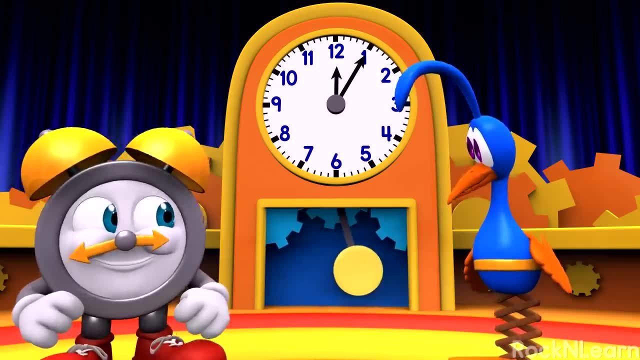 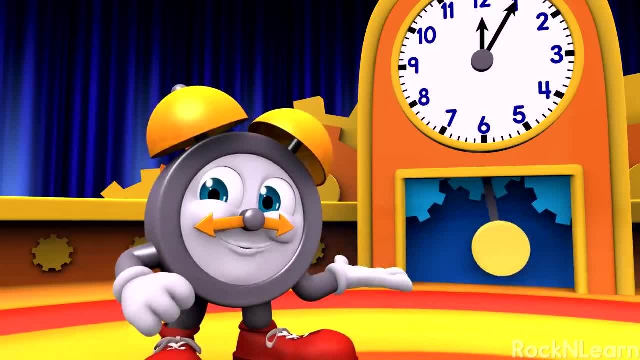 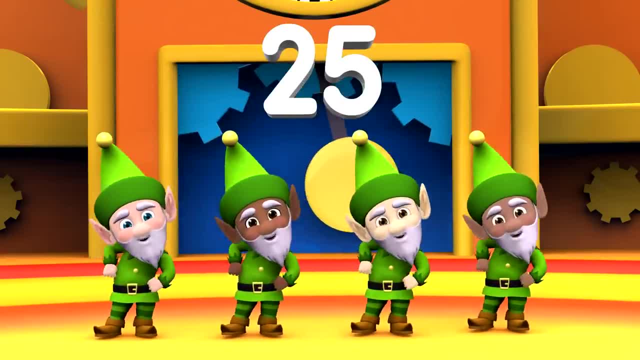 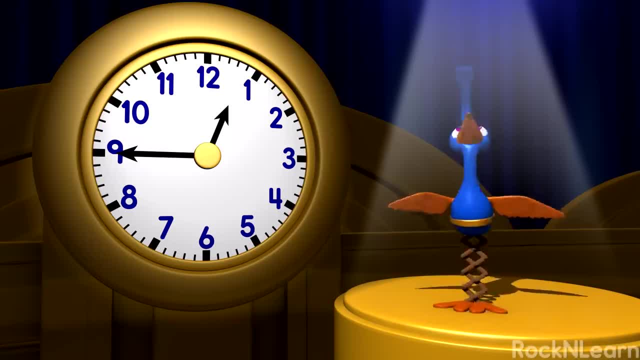 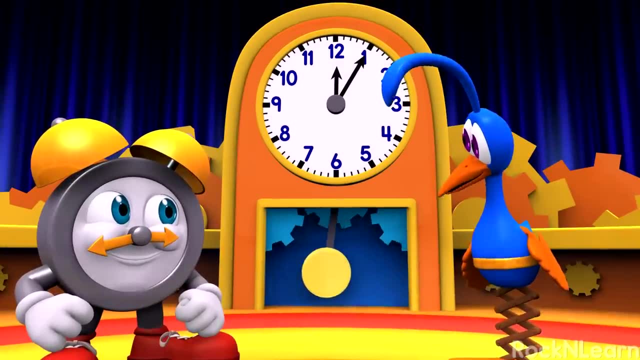 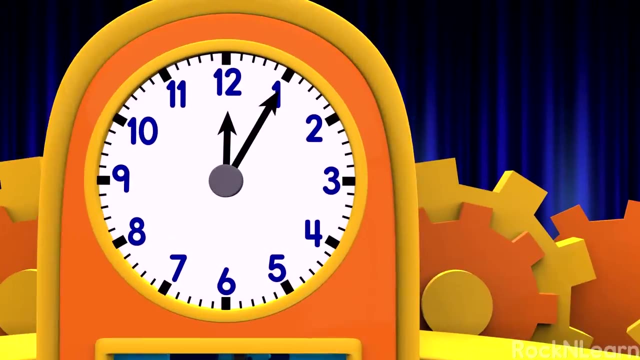 thank you. thank you, hey, Timothy time. what happens if the minute hand is on one of the other numbers? well, cuckoo. every time the minute hand is on a number, five minutes have passed. do you know how to count by two or three minutes, by fives, all the way to sixty. Cuckoo, Cuckoo. yeah, And I know why we have to count by fives. 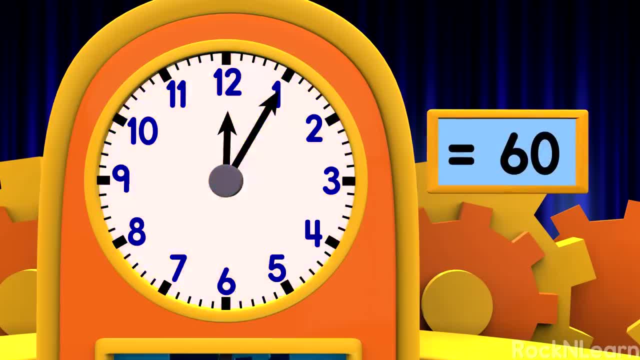 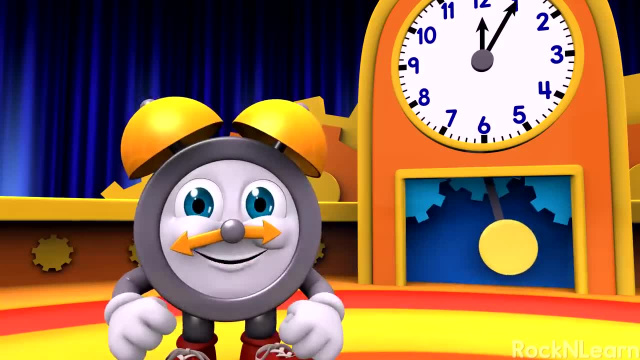 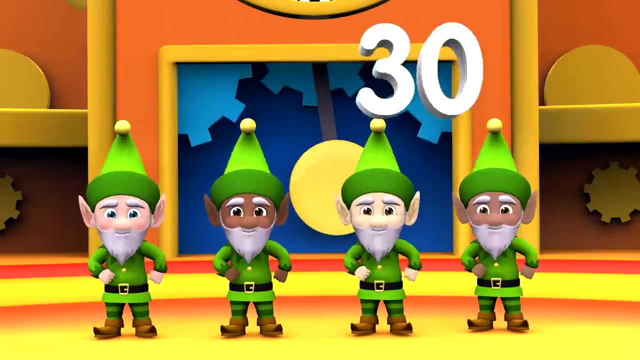 up to sixty. It's because there are sixty minutes in each hour. Can we practice a few times together with some music? Sure, we can, and my little friends will help. Five, ten, fifteen, twenty, twenty-five, thirty, thirty-five, forty, forty-five, fifty, fifty-five, sixty. 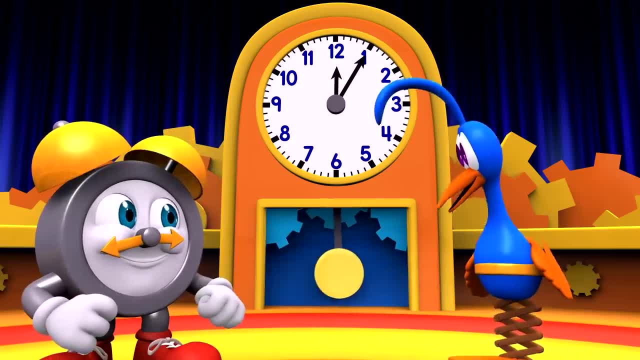 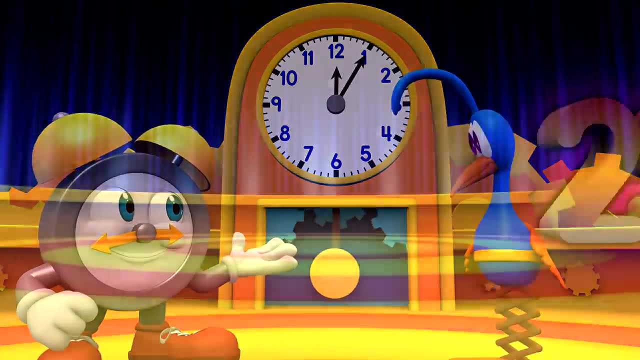 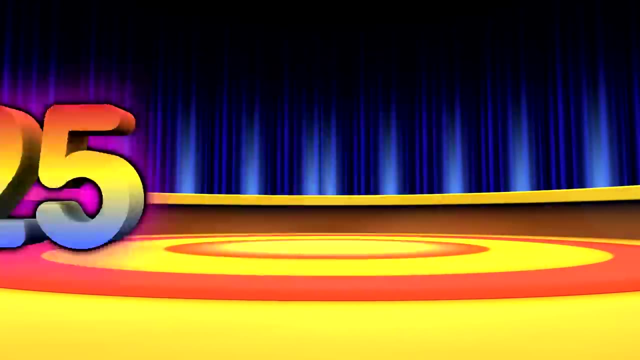 That's right, Let's do it again, Okay, but could we do it without the elves? Sure thing, Cuckoo. How's this? Five, ten, fifteen, twenty, twenty-five, thirty, thirty-five, forty, forty-five, fifty, thirty-five, sixty. One more time. 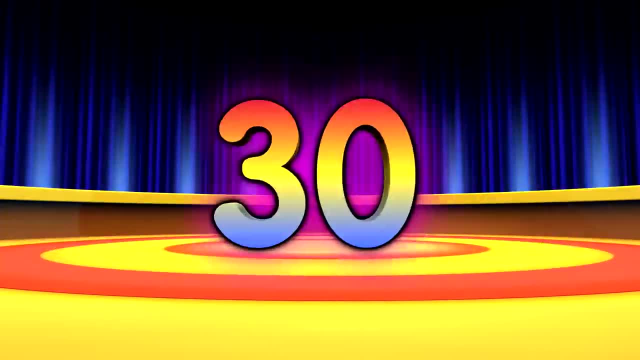 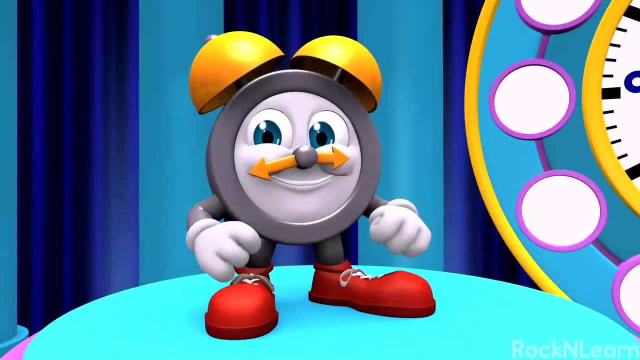 Three, five, ten, fifteen, twenty, twenty-five, thirty, thirty-five, forty, forty-five, fifty, fifty-five, sixty. That was fun. Now let's see how we can use counting by fives to help us tell time to. 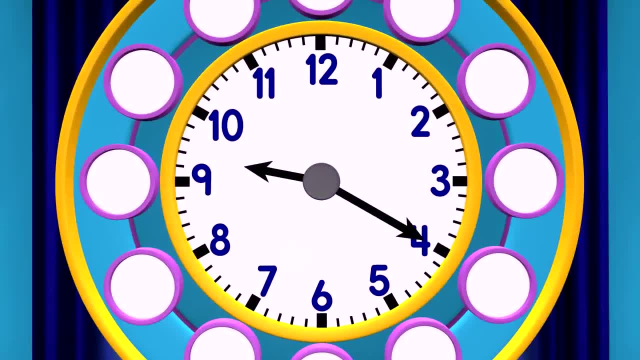 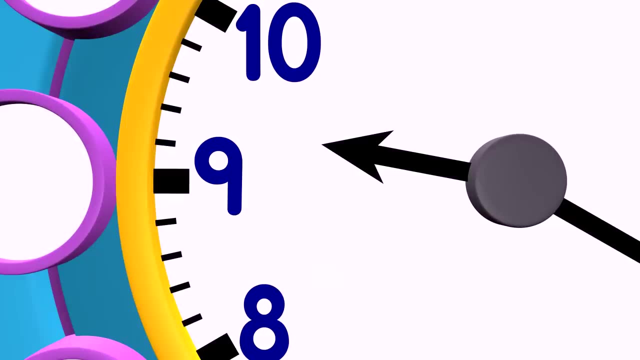 five minutes. Each number on the clock shows five more minutes past, So if you count by fives, you'll learn this really fast. Look at the hour hand. What number has it passed? That will be the hour, Wasn't that? 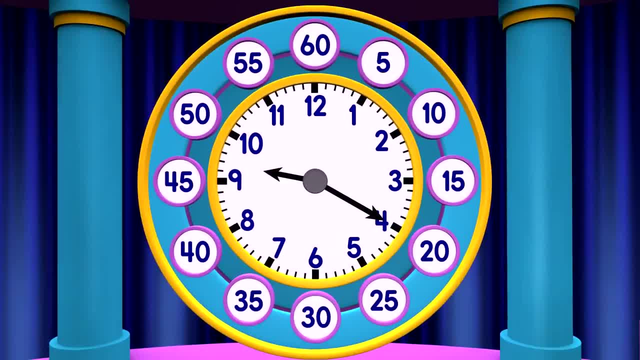 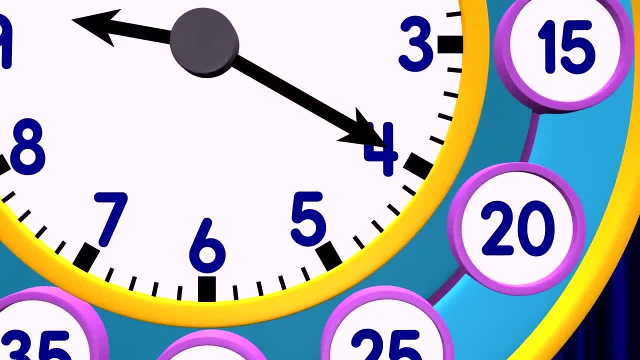 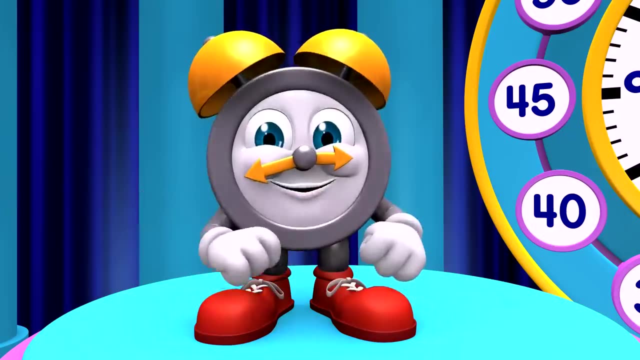 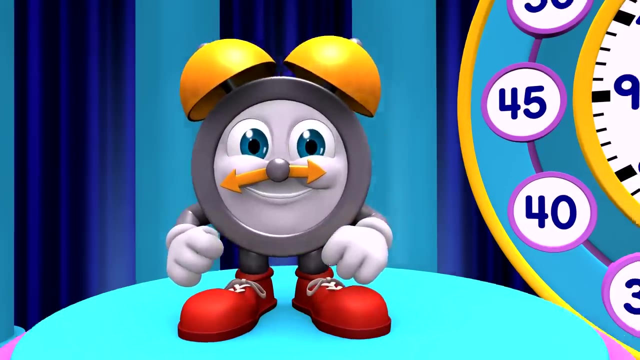 a blast. Now count by fives, starting from the one till you reach the minute hand, and then you will be done. Just say the hour now and say the minutes, then The ones you counted up by fives. let practice now begin. 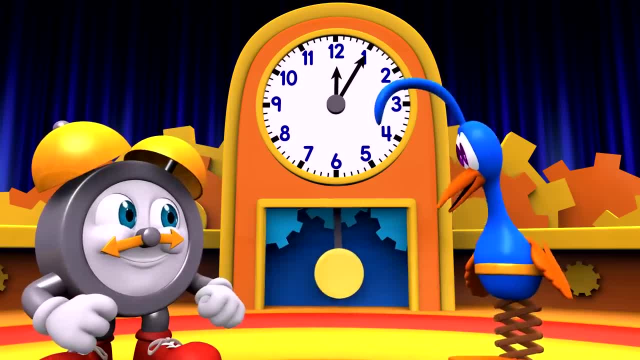 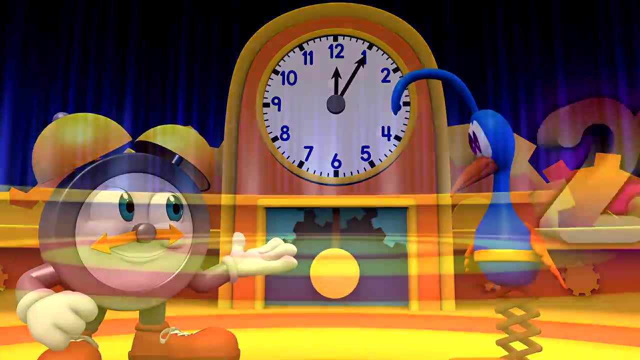 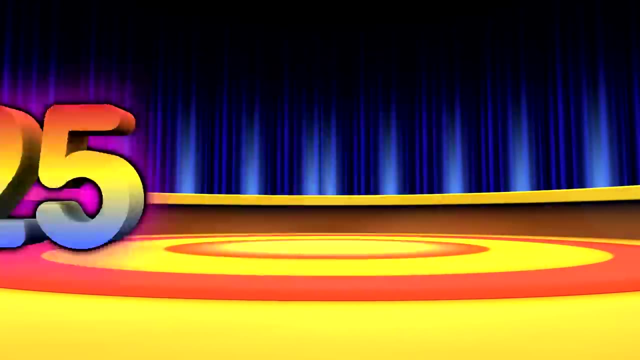 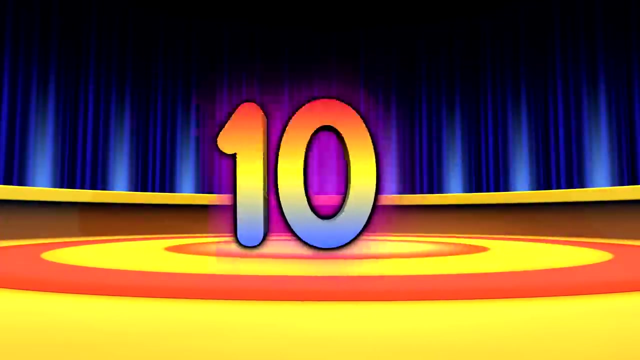 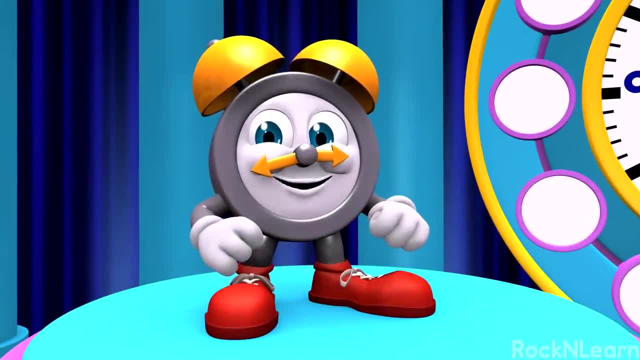 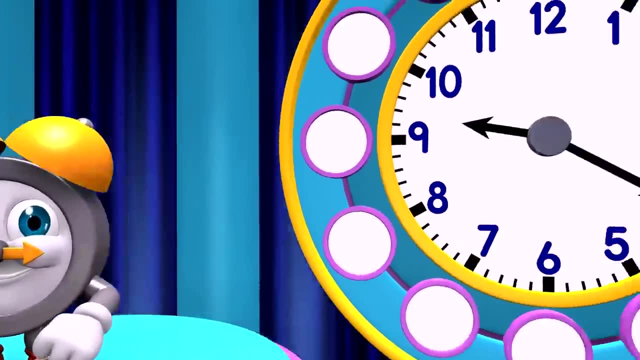 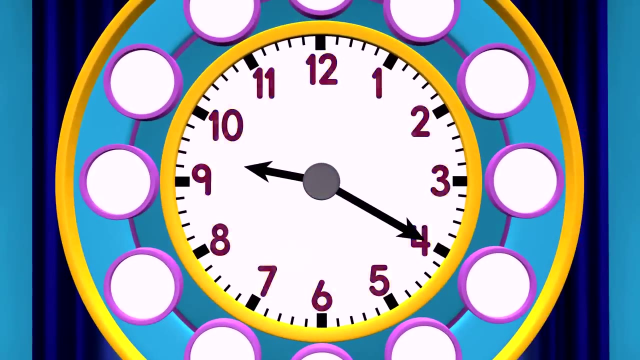 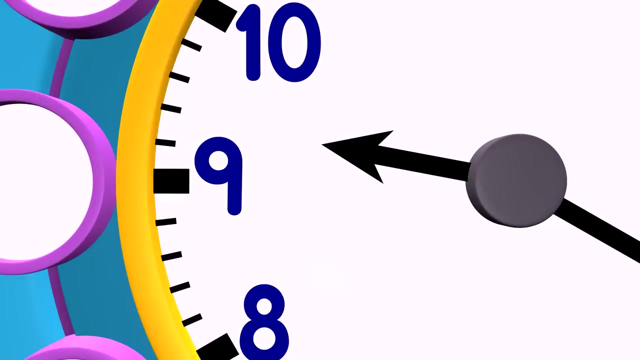 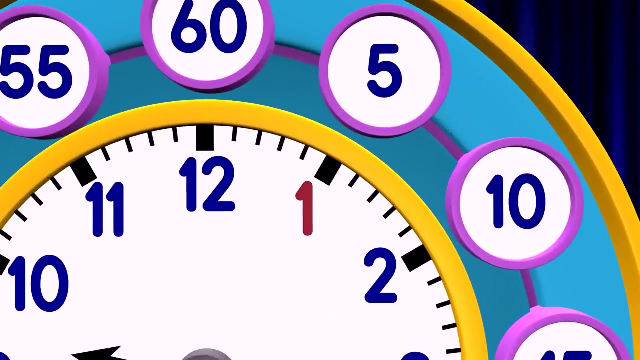 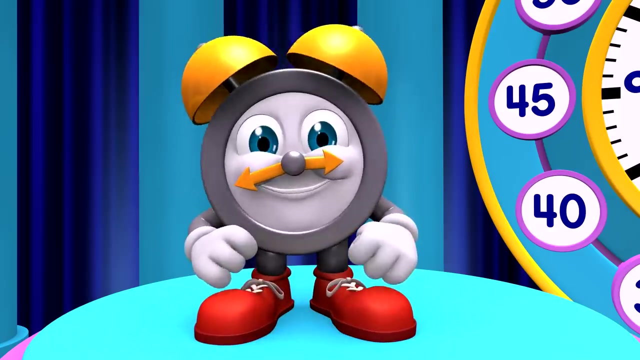 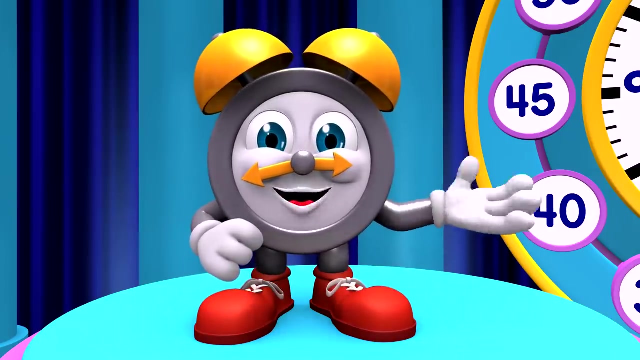 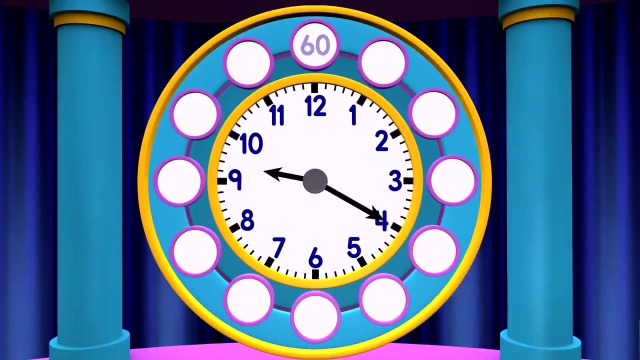 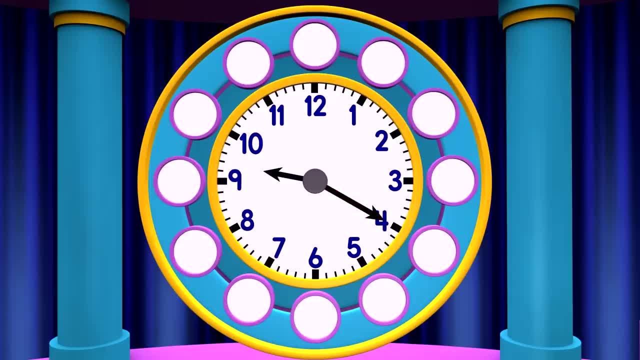 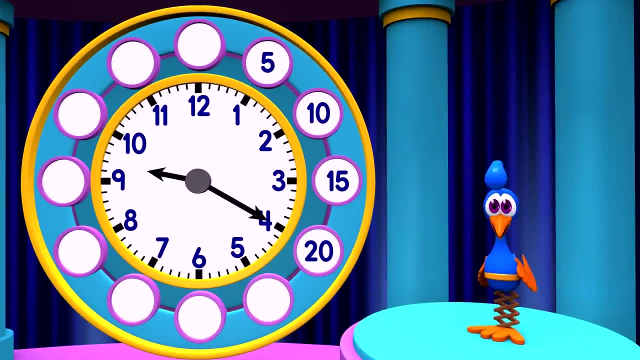 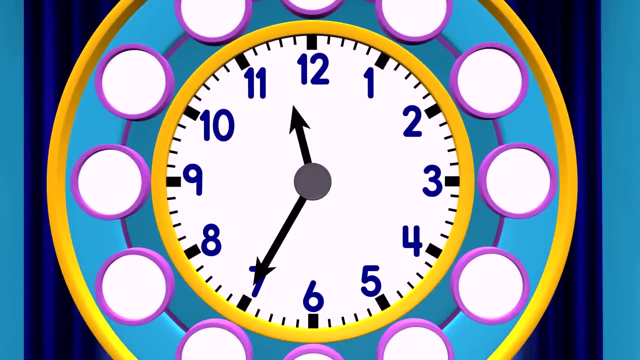 It's pointing at the four. So we count by fives. four times Five. ten, fifteen, twenty. Aha, It must be nine, twenty. That's right, Cuckoo. Now look at the hour hand. at this one, the hour is 11. and what about the minute hand? it's pointing at the seven. 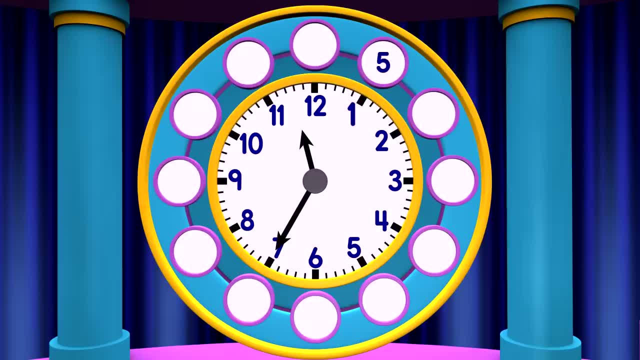 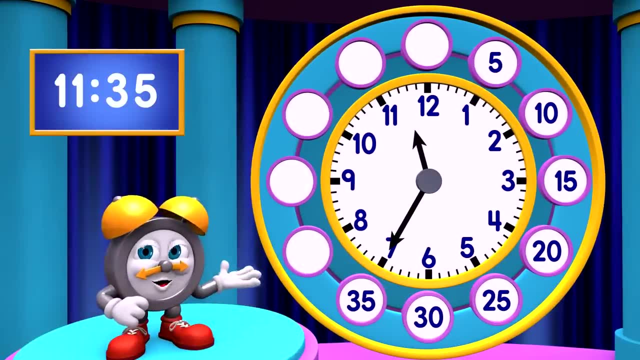 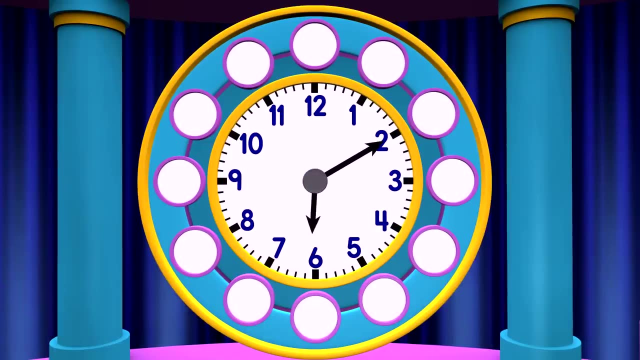 that's right, let's count: 5, 10, 15, 20, 25, 30, 35. it's 11, 35. the hour hand is past the six and the minute hands on the two. what time is it, cuckoo? it's 6, 10. now you've got it. 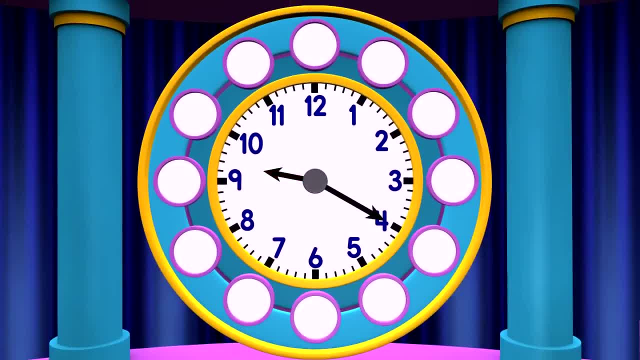 Look at the hour hand. It's a little past nine. Nine is the hour Now. look at the minute hand. It's pointing at the four. So we count by fives. four times Five, ten, fifteen, twenty. Ah ha, It's a minute hand. 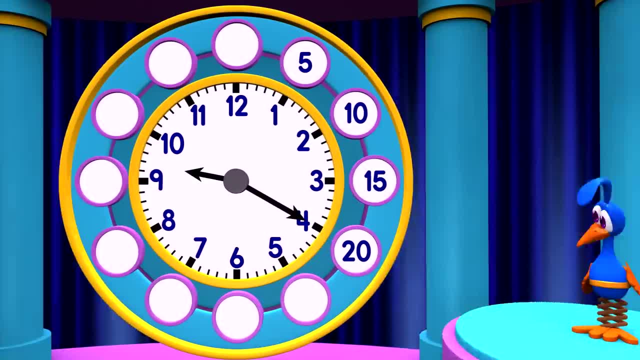 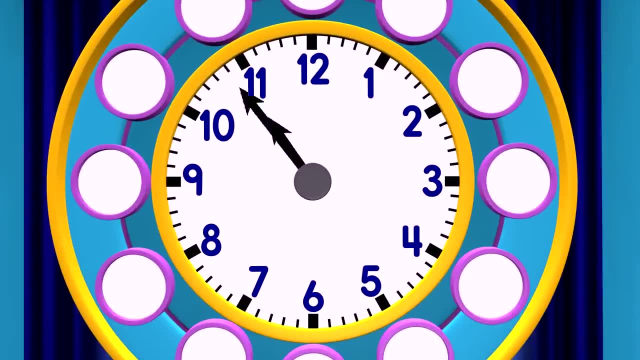 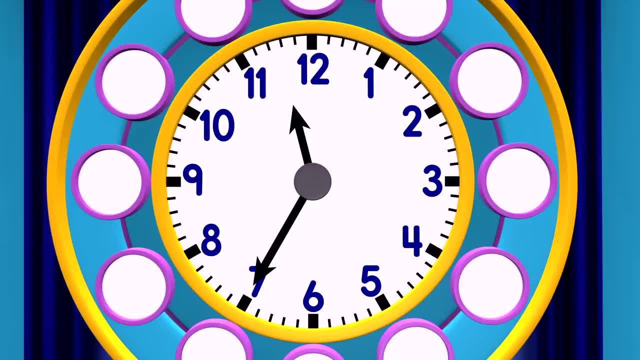 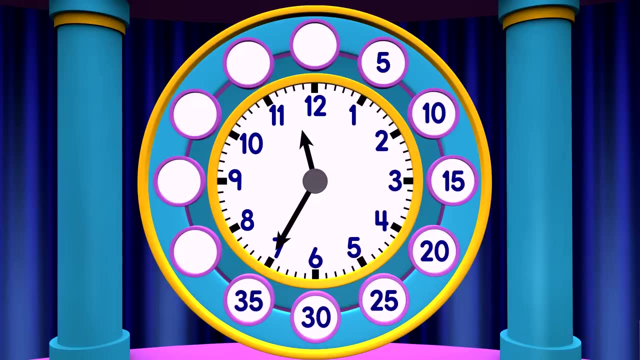 The hour is 11.. And what about the minute hand? It's pointing at the 7.. That's right, Let's count 5, 10,, 15,, 20,, 25,, 30,, 35.. It's 11.35.. 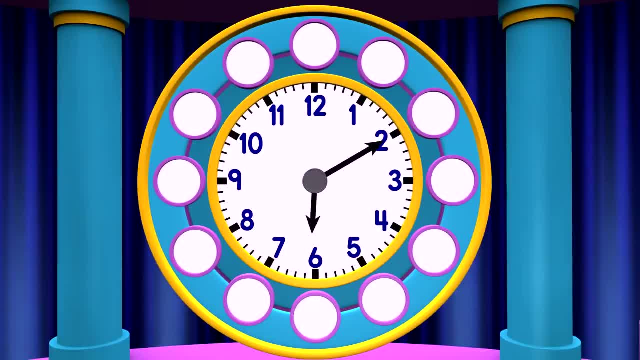 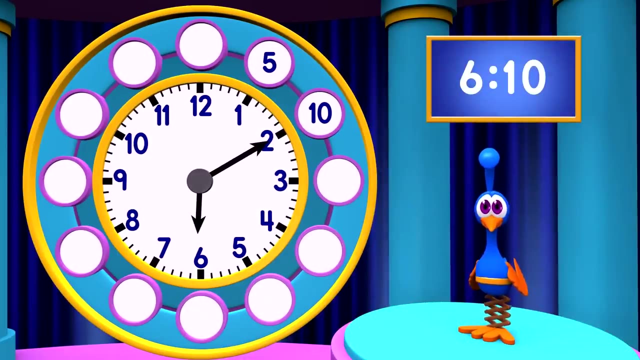 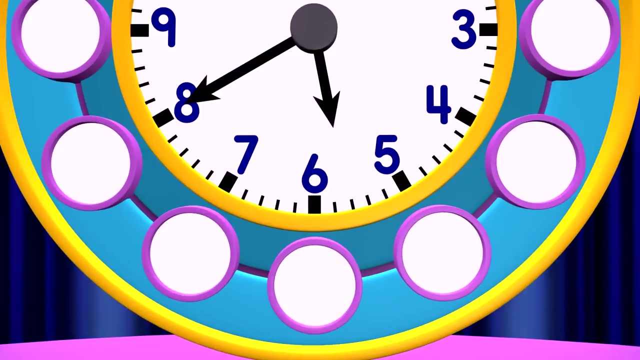 The hour hand is past the 6. And the minute hand's on the 2.. What time is it, Cuckoo? It's 6.10.. Now you've got it, Cuckoo. The little hand is past the 5.. 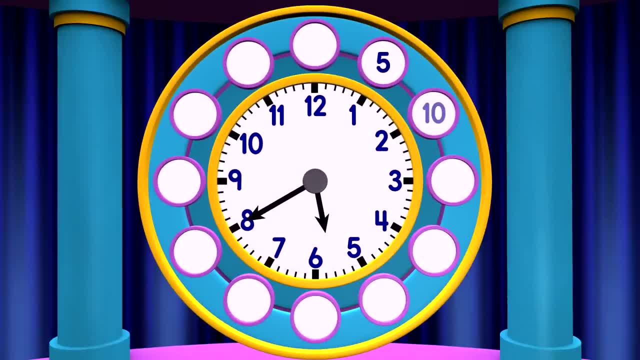 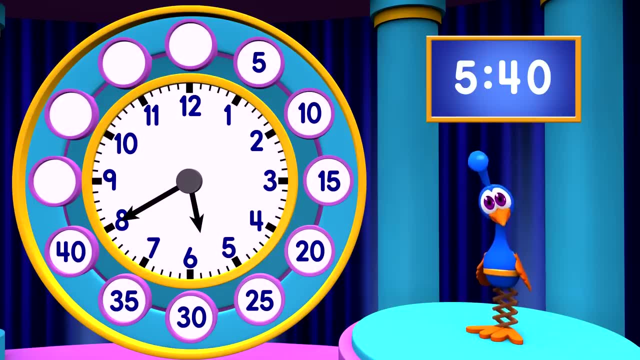 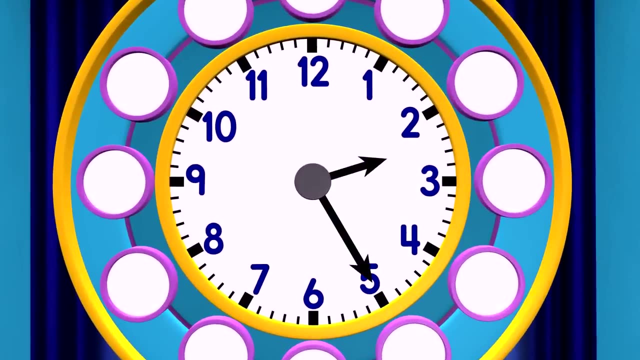 And the big hand's on the 8.. So the time is 5.40.. Very good, You remembered that the minute hand is bigger than the hour hand. Cuckoo, The hour hand is past the 2. And the minute hand's on the 5.. 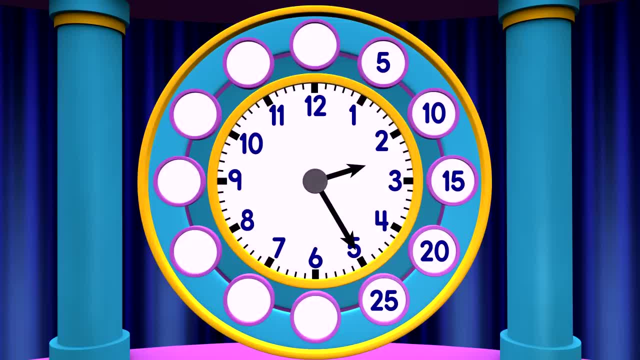 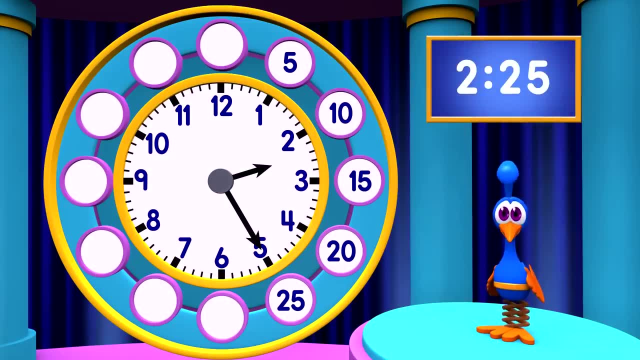 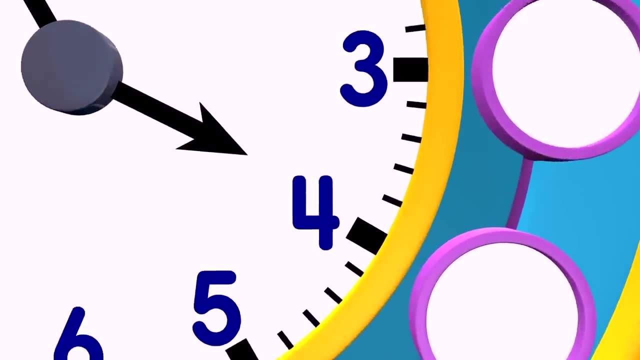 Counting up by 5's, 5 times gives the number 25.. Cuckoo, This clock shows a time of 2.25.. That's correct. What about this one? The hour is almost 4.. But we must use the number that was before. 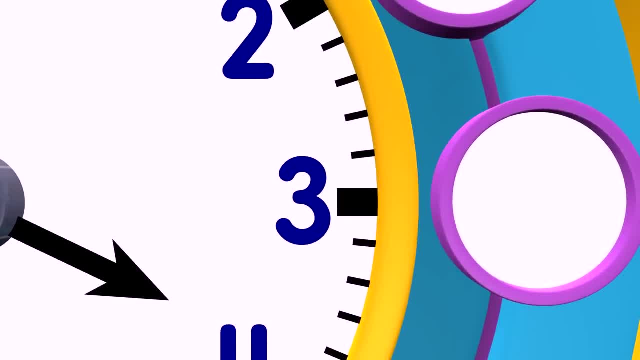 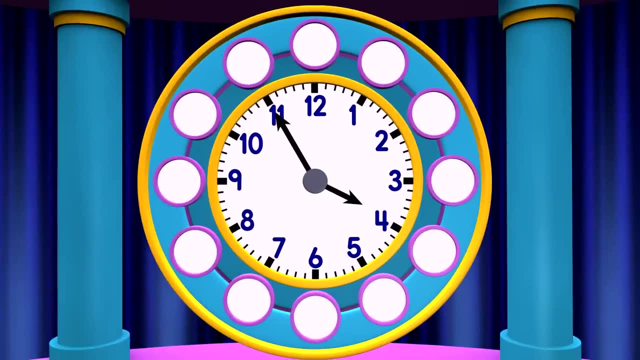 Cuckoo. The hour is 3.. But what about the minutes? 11 times will count by 5.. Might as well begin it. minutes: 11 times will count by 5. might as well begin it. 5, 10, 15, 20, 25, 30, 35, 40. 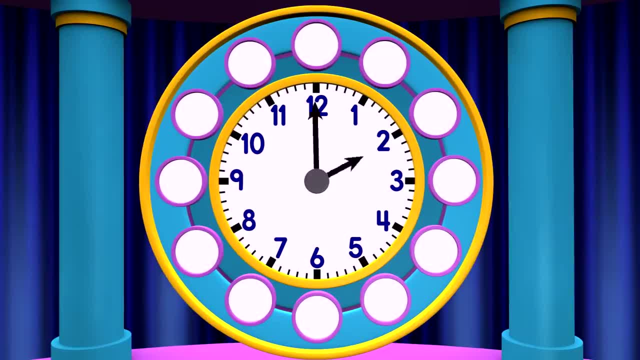 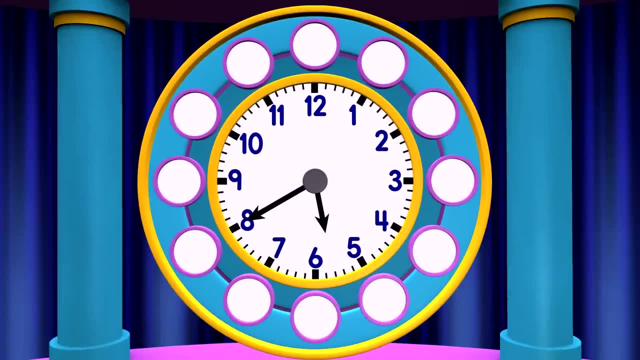 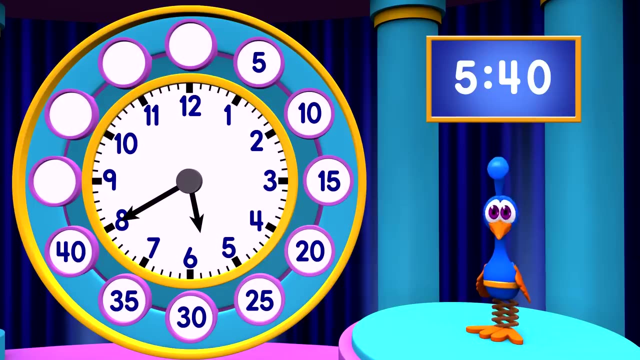 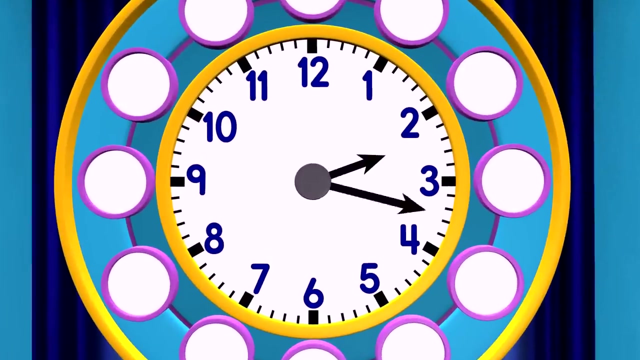 the little hand is past the five and the big hands on the eight, so the time is 5: 40.. very good, you remembered that the minute hand is bigger than the hour hand. the hour hand is past the two and the minute hands on the five. 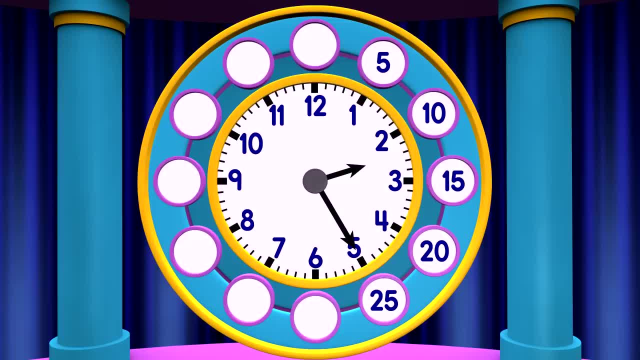 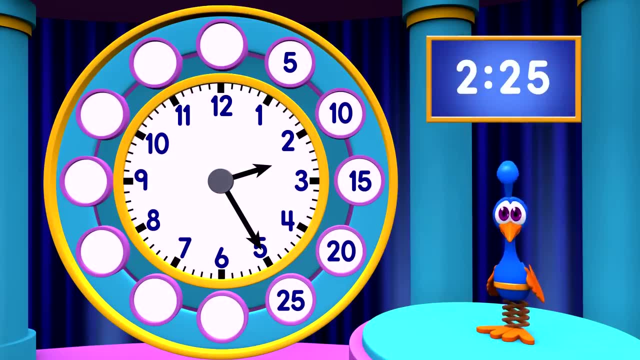 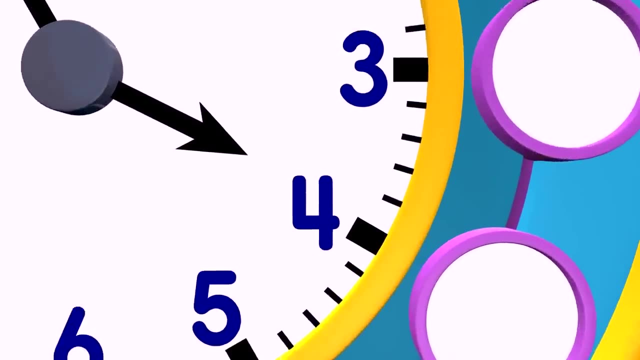 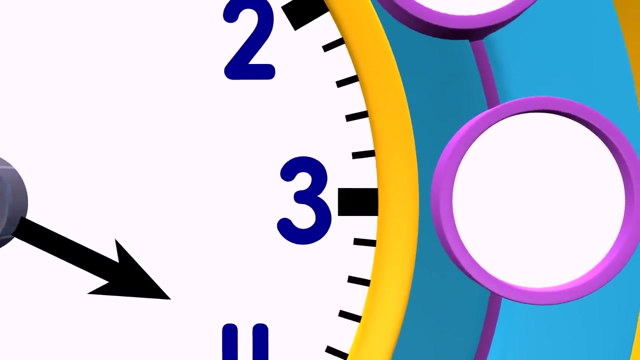 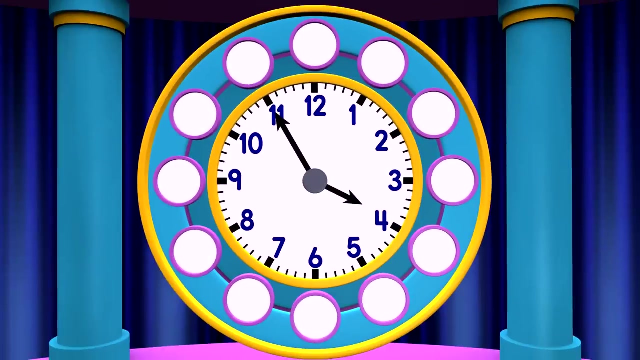 counting up by fives. five times gives the number 25.. this clock shows a time of 2: 25.. what about this one? the hour is almost four, but we must use the number that was before. the hour is three. but what about the minutes? 11 times, we'll count by five. might as well begin it. 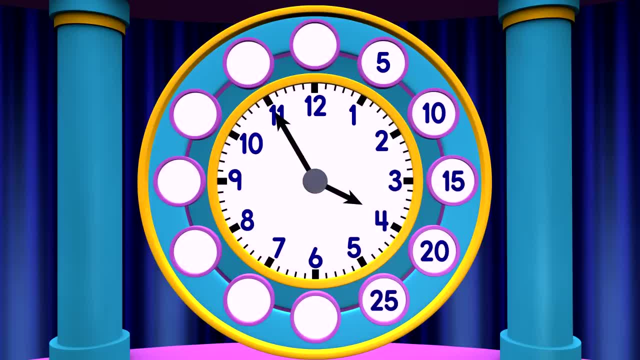 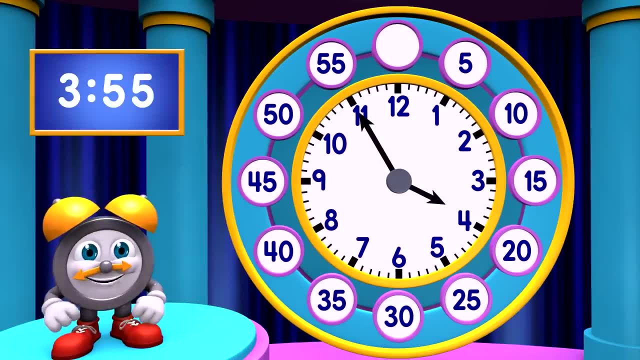 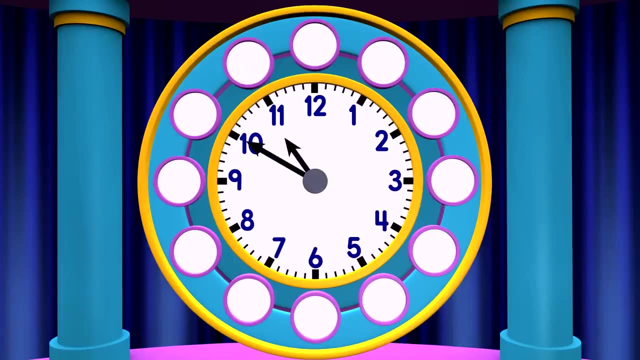 5, 10, 15, 20, 20, 5, 30, 35, 40, 45, 50, 55.. you got it: 3, 55.. what time is it now? the hour hand is almost up to the 11, so the hour must be 10.. 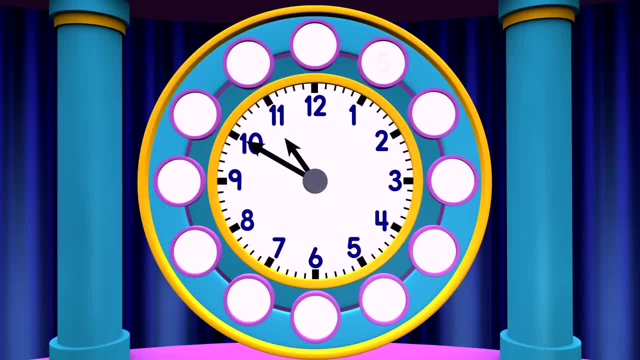 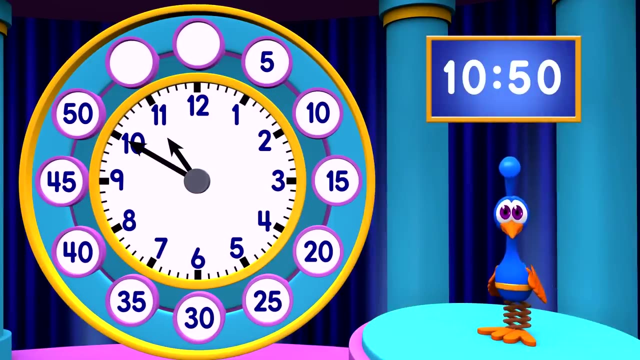 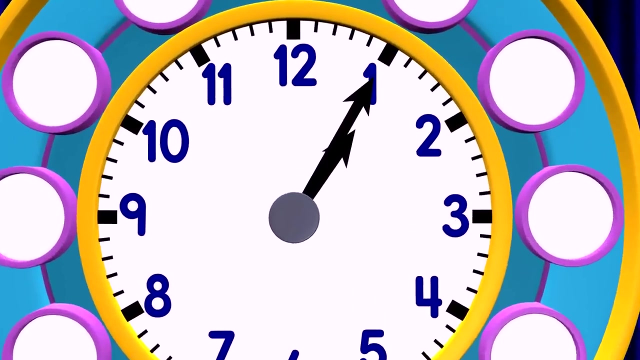 speaking of ten, that's where the minute hand is pointing. Did you count by fives? I sure did, all the way to fifty. Well then it must be ten-fifty, Cuckoo ten-fifty. Oh no, the minute hand and the hour hand are almost the same. 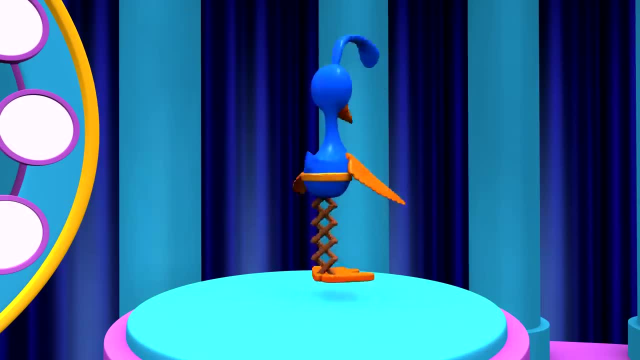 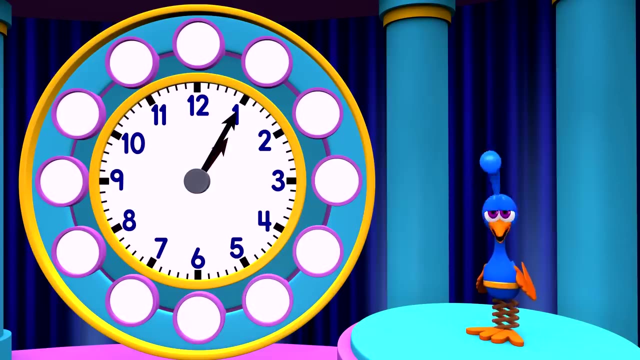 Now what are we gonna do? Cuckoo, cuckoo, cuckoo, cuckoo, cuckoo, cuckoo. Calm down Cuckoo. it's really quite simple. Where's the hour hand? Uh, just barely past the one. 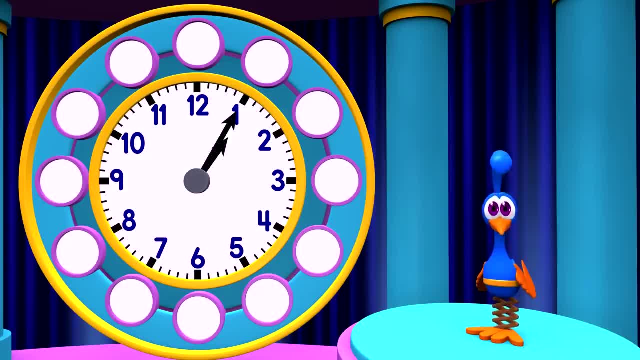 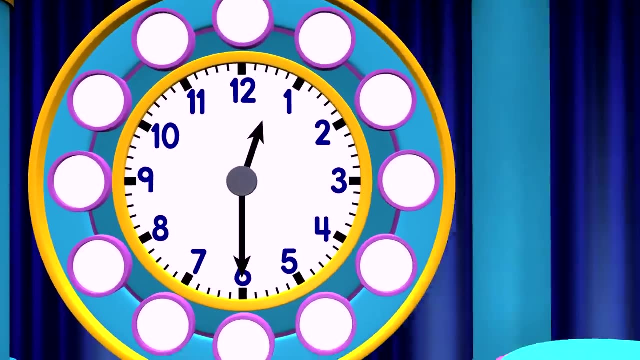 Oh, I see the hour must be one. That's right. and where might the minute hand be? The minute hand is on the one, Easy enough. we don't even have to count. It's one-oh-five. This one is easy. We learned that this time is twelve-thirty. 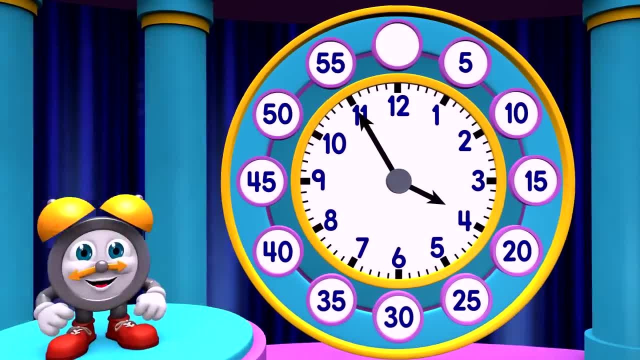 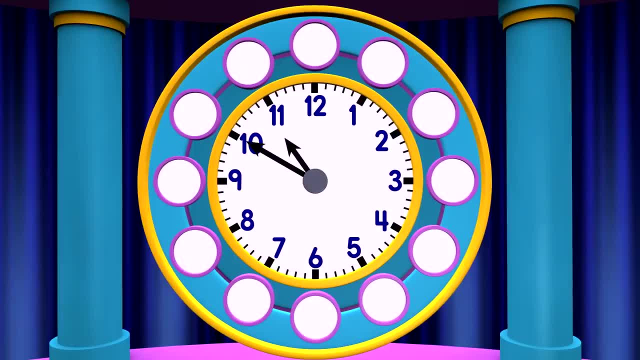 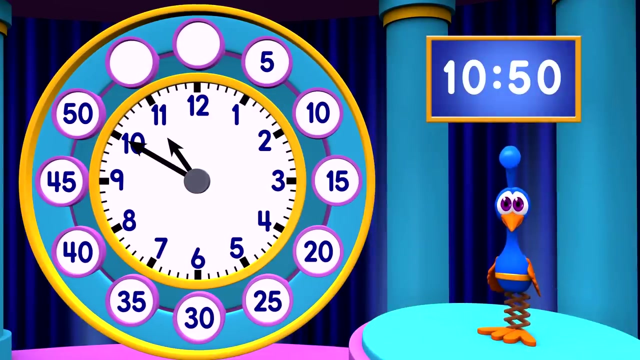 45, 50, 55, you got it 355. what time is it now? the hour hand is almost up to the 11, so the hour must be 10. speaking of 10, that's where the minute hand is pointing. did you count by fives? I sure did, all the way to 50. well then, it must be 1050. 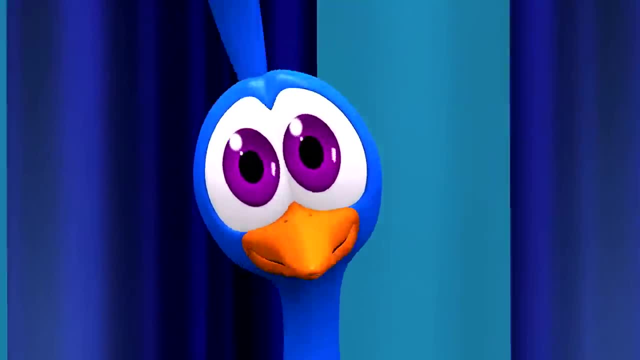 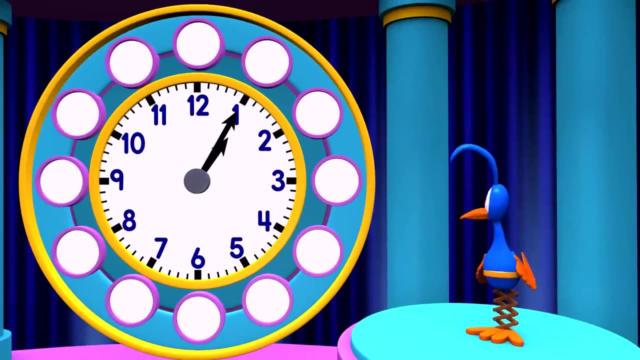 almost the same. now, what are we gonna do? it's really quite simple. where's the hour hand? just barely passed the one. oh, I see the hour must be one, that's right. and where might the minute hands be? the minute hand is on the one, easy enough, we. 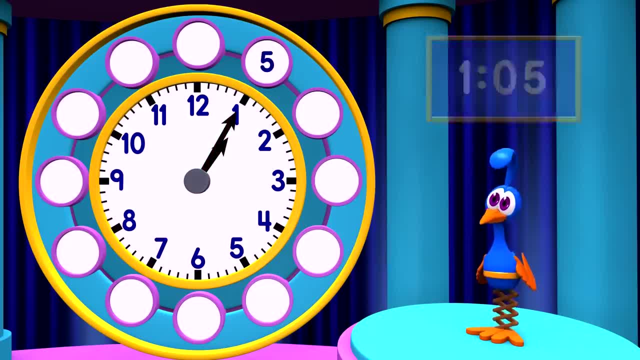 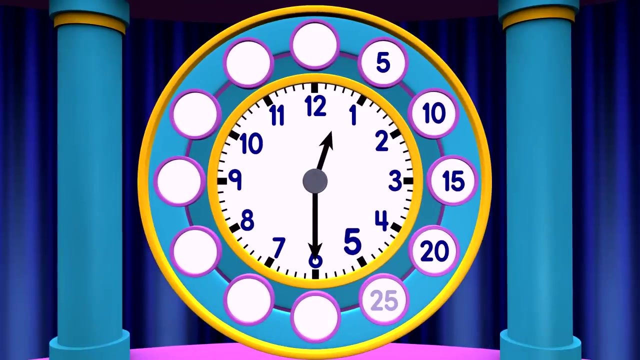 don't even have to count, it's 105. this one is easy. we learned that this time is 12, 30 or half past 12. but what if we count the minutes? will we get the same time? sure we will. cuckoo, let's do it. 5, 10, 15, 20, 25, 30. you can always count by fives to figure out the time. 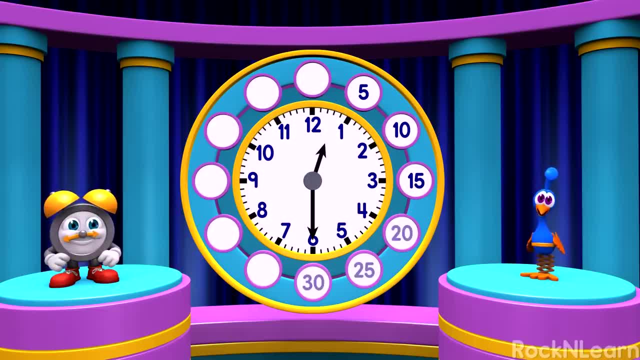 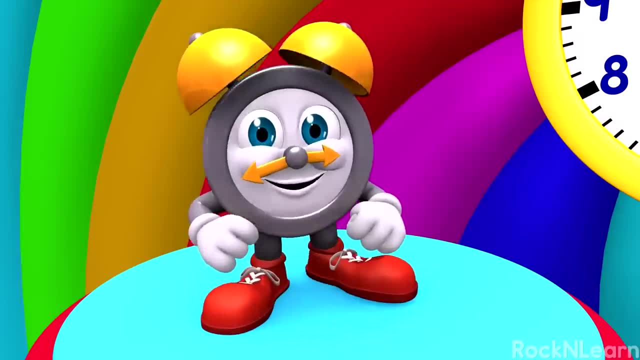 even if it is the quarter hour or half hour. you can always count by fives to figure out the time, even if it is the quarter hour or half hour, even if it is the quarter hour or half hour, let's do a few more so we get it down. if it goes too fast this time, make 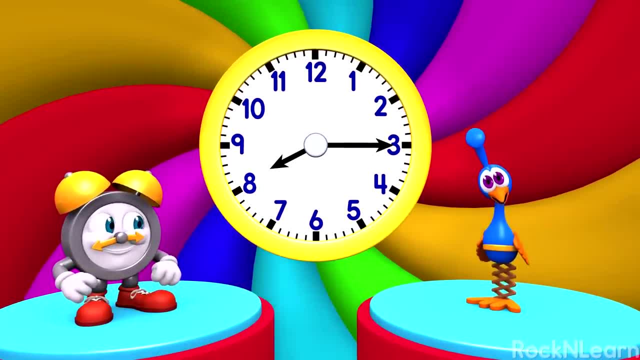 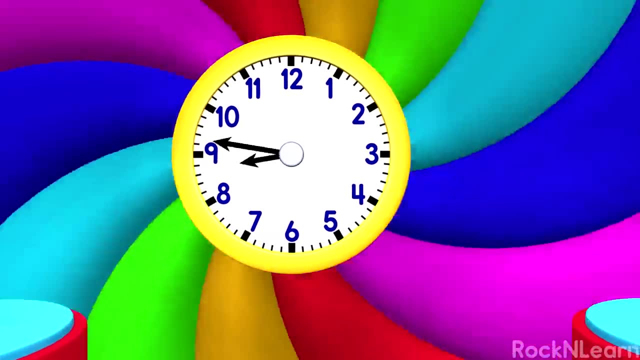 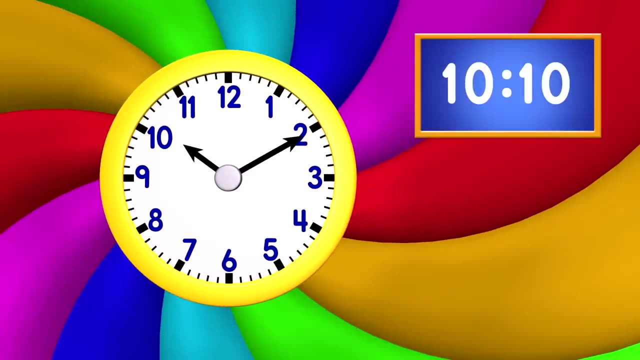 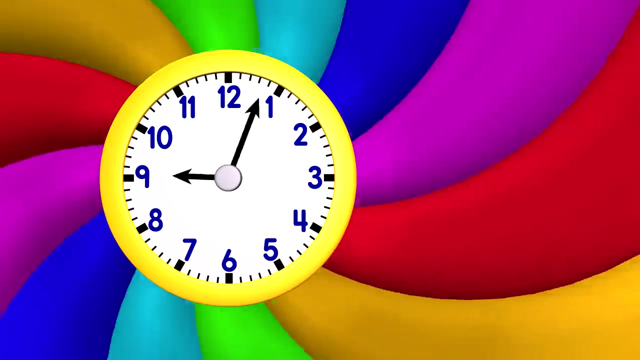 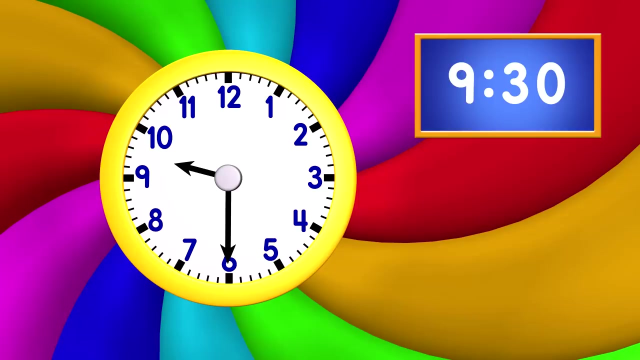 another round. some thinking time. try to save the time before you hear Timothy's voice or mine. some thinking time. try to save the time before you hear Timothy's voice or mine: 10, 10, 10, 10, 135, 930 or half past nine, 930 or half past nine. 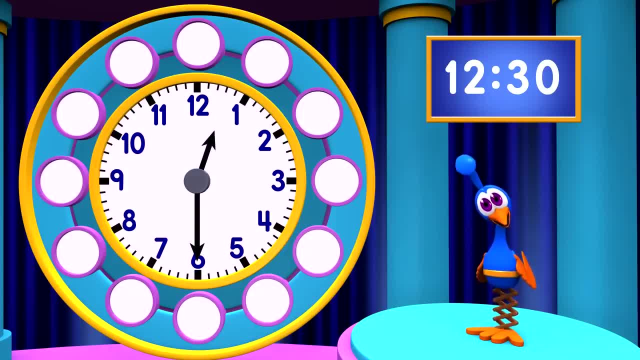 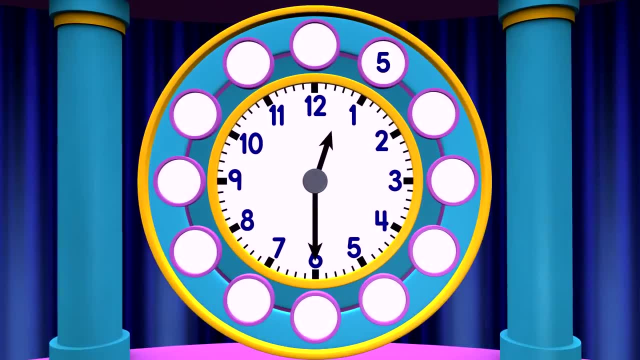 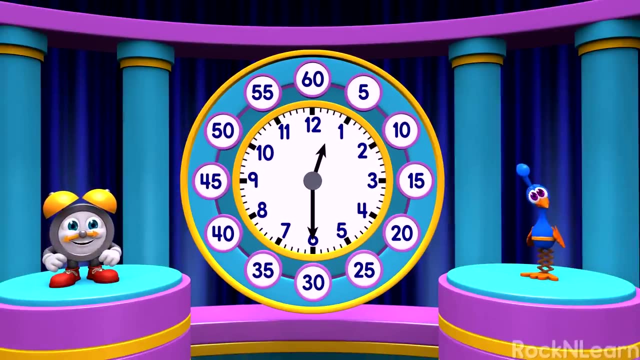 Or half past twelve. But what if we count the minutes? Will we get the same time? Sure, we will. Cuckoo, Let's do it. Five, ten, fifteen, twenty, twenty-five, thirty. You can always count by fives to figure out the time. 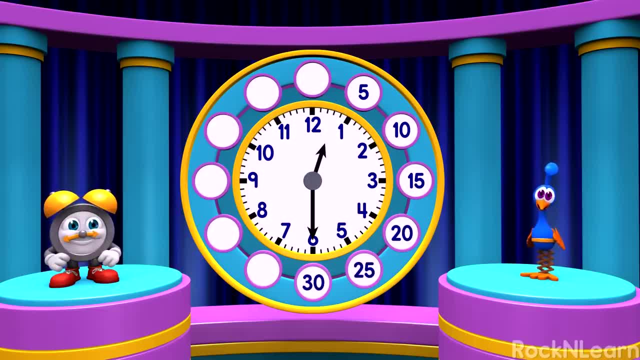 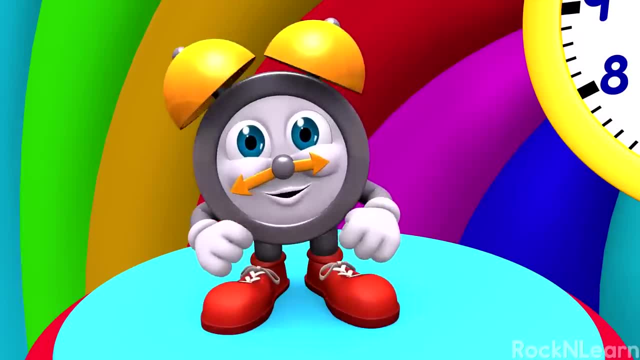 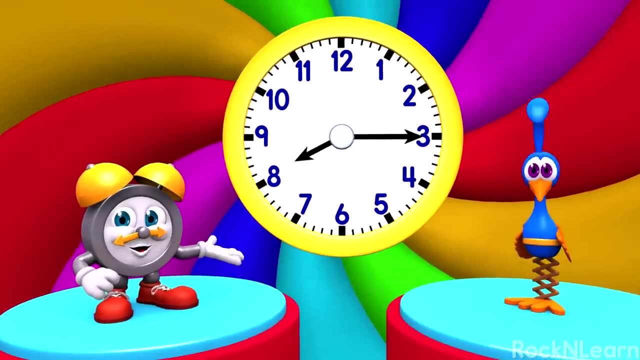 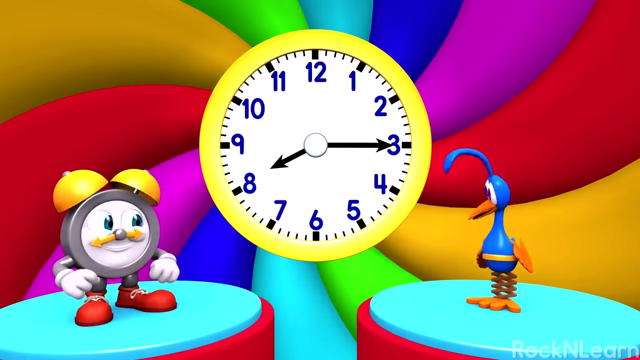 Even if it is the quarter hour or half hour, Let's do a few more so we get it down. If it goes too fast this time, make another round First. we'll look at the clock and give some thinking time. Try to save the time before you hear Timothy's voice or mine. 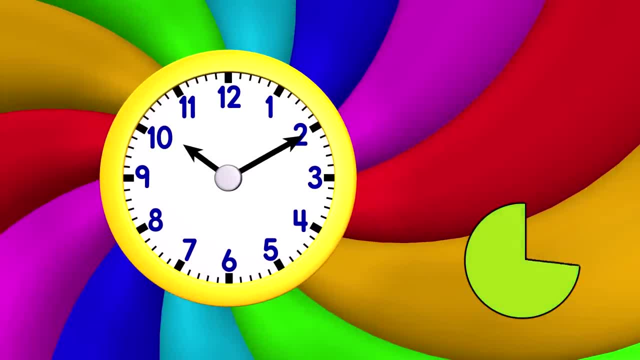 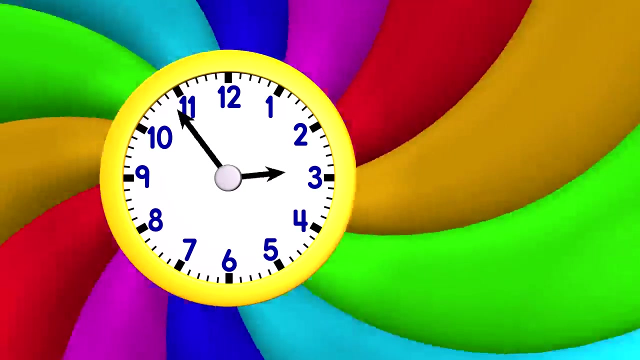 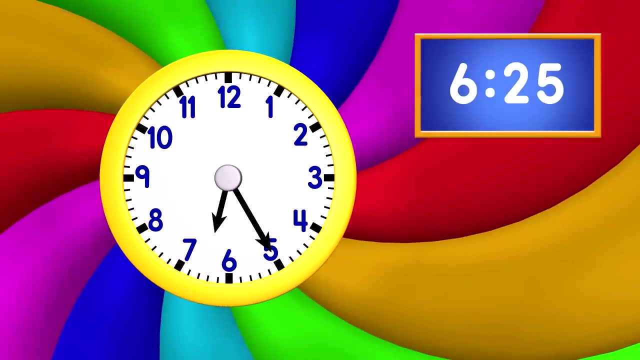 Ten-ten, One-thirty-five, Nine-thirty Or half past nine, Six-twenty-five, One-thirty-five: 2.40, 11.55, 5.05, 3.45 Or a quarter till four. 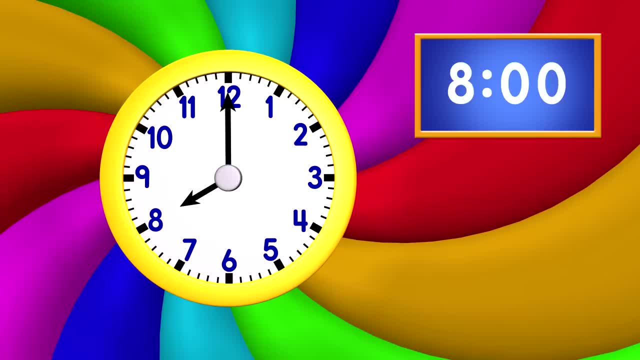 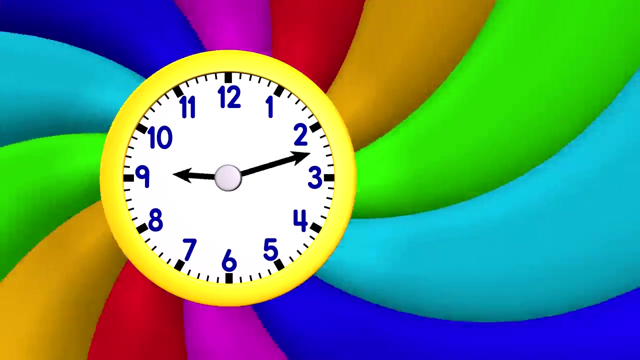 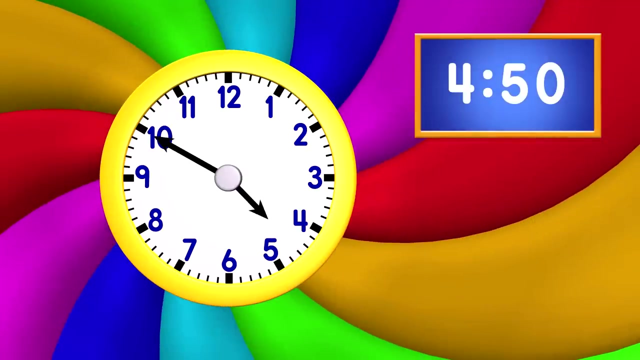 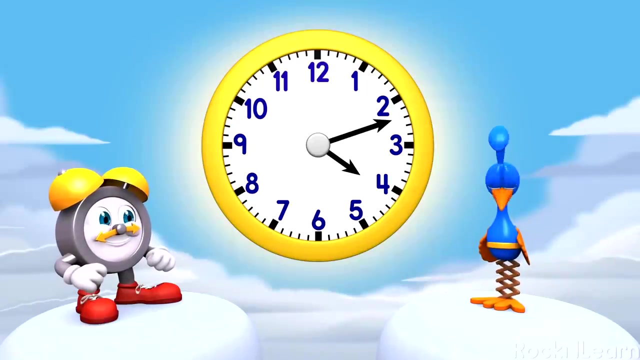 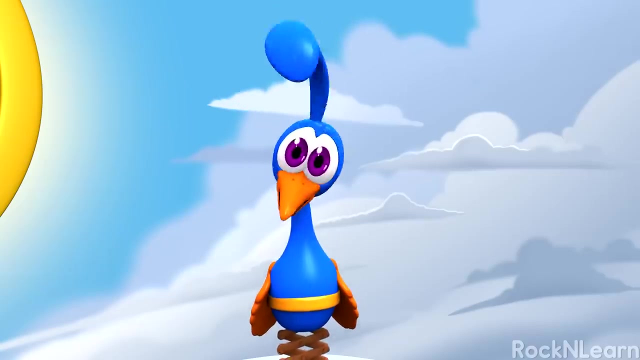 8 o'clock, 12.20, 7.15 Or a quarter past seven, 4.50, Cuckoo, Wow. Telling time is easy as long as the minute hand is on a number, But what do we do when the minute hand is between numbers? 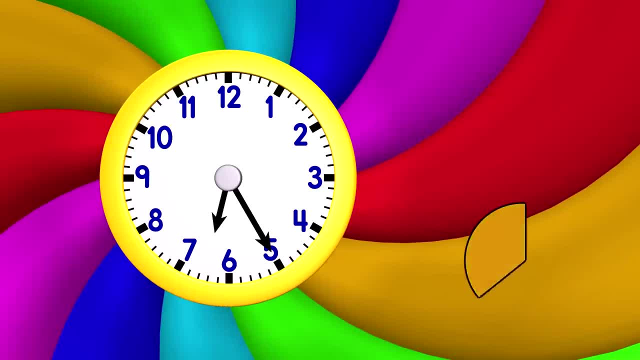 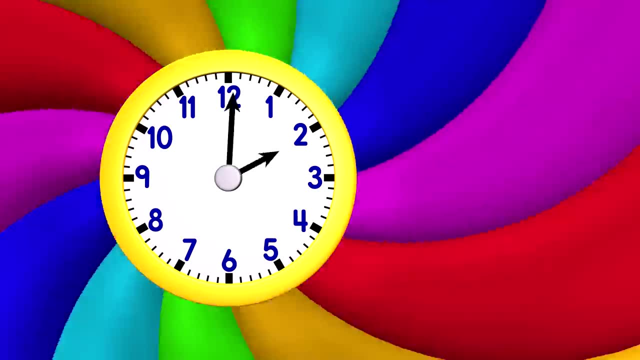 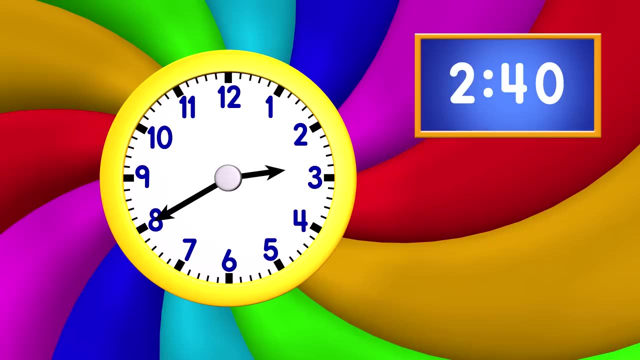 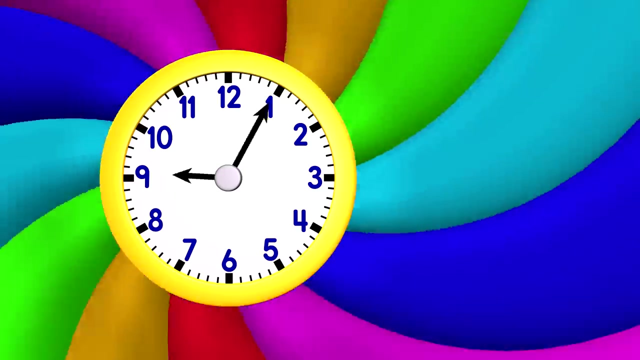 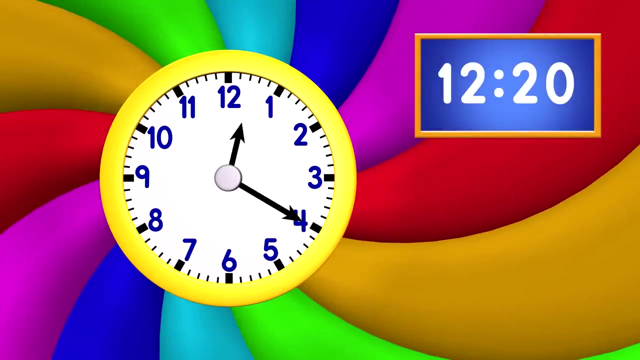 930 or half past nine. 15, 930 or half past nine. jaw jim, jim jimes, jim jimes, Five-oh-five, Three-forty-five Or a quarter till four Eight o'clock, Twelve-twenty, Seven-fifteen Or a quarter past seven. 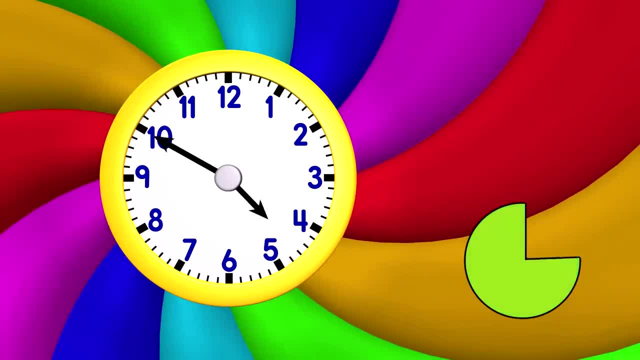 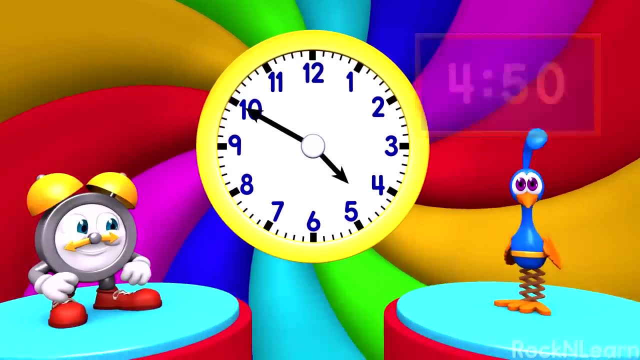 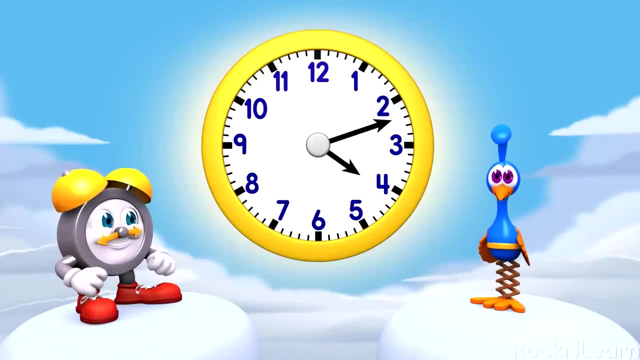 Four-fifty, Cuckoo. Wow. Telling time is easy as long as the minute hand is on a number, But what do we do when the minute hand is between numbers? Well, Cuckoo, do you see the little lines on the outer edge of the clock face? 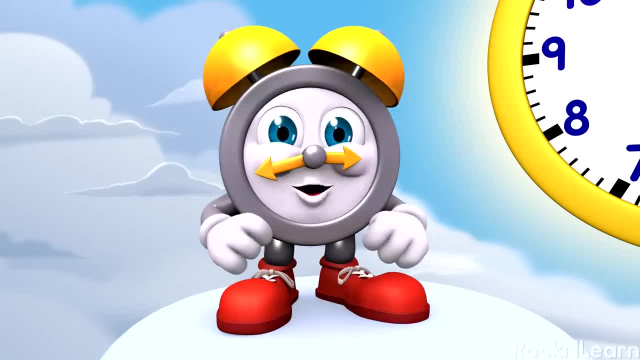 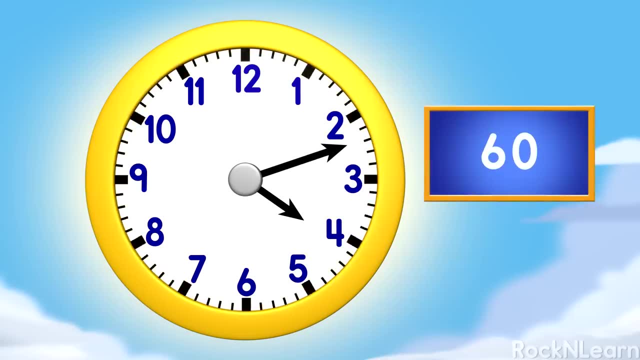 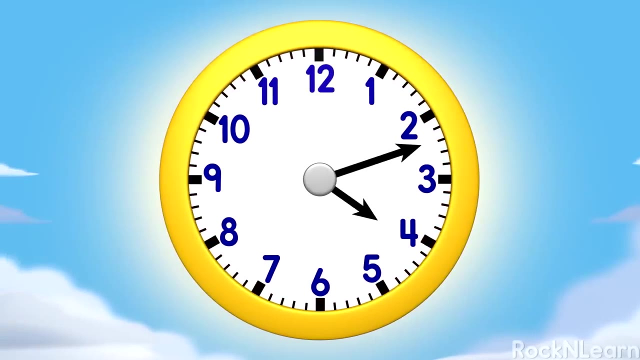 Yeah, I hadn't really noticed them before. Do you know how many little marks are on the clock? Let me guess, Is it sixty? You got it, Cuckoo. That's sixty lines for sixty minutes in an hour. When you tell time to the minute, the hour is fun to find. 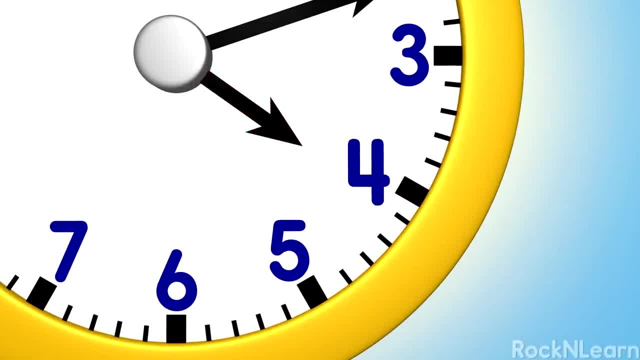 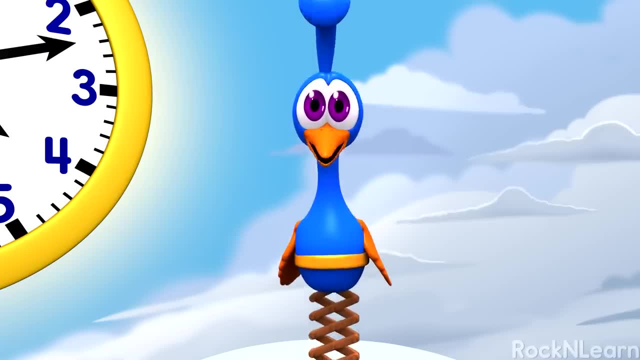 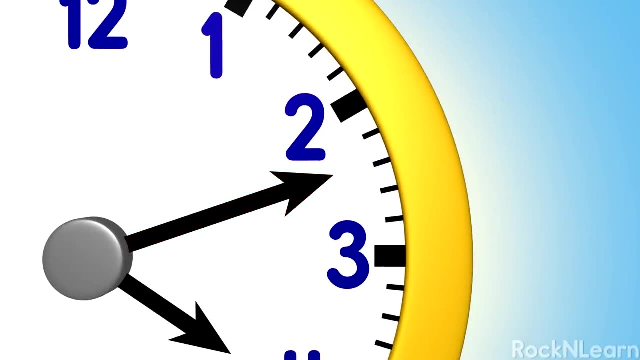 Just look for the hour hand and find the number it's left behind. That gives us the hour. Now we need the minutes, So find the minute hand and count by fives, the way we do. We'll stop On the number before the minute hand, we and you. 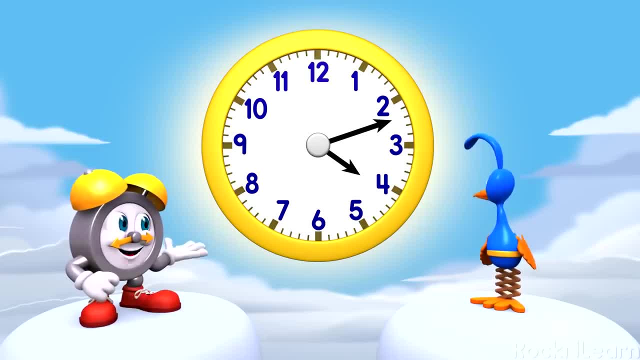 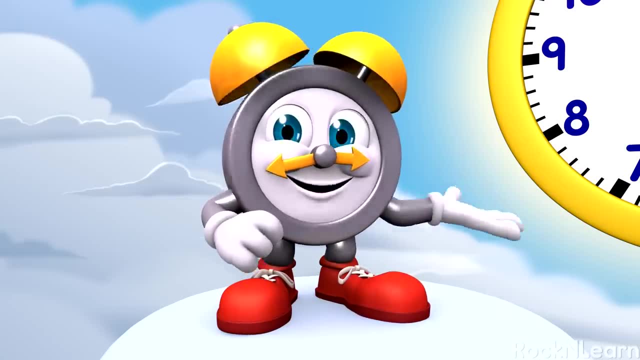 Well, tell time. Well, tell time Now, Cuckoo, do you see the little lines on the outer edge of the clock face? Yeah, I hadn't really noticed them before. Do you know how many little marks are on the clock? 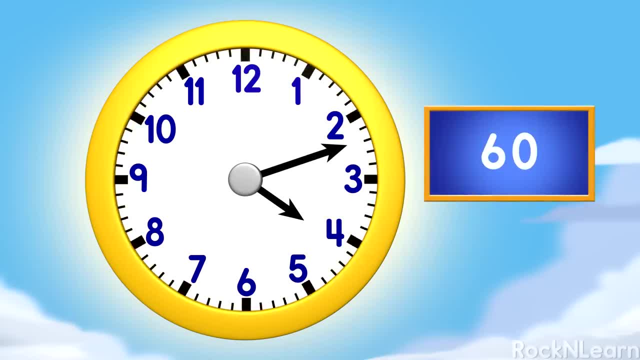 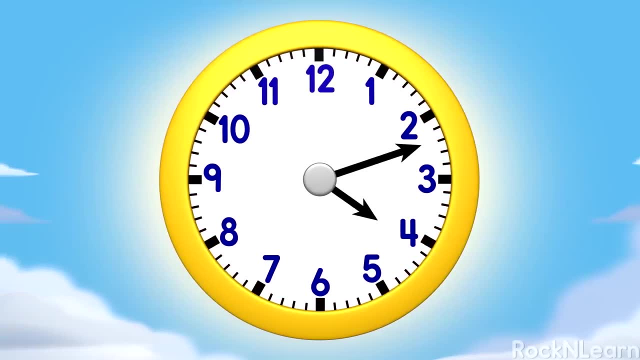 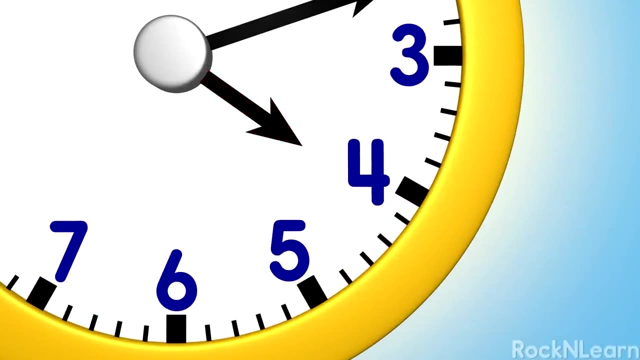 Let me guess, Is it 60?? You got it, Cuckoo. That's 60 lines for 60 minutes in an hour. When you tell time to the minute, the hour is fun to find. Just look for the hour hand and find the number. it's left behind. 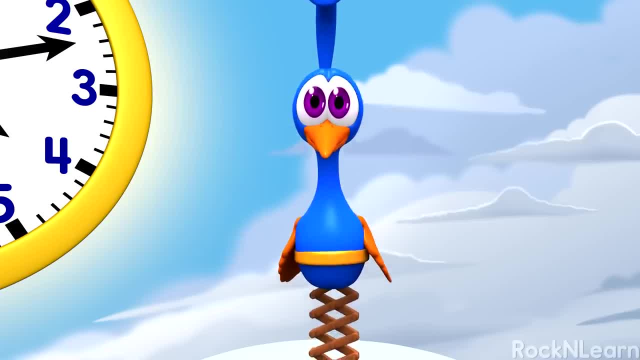 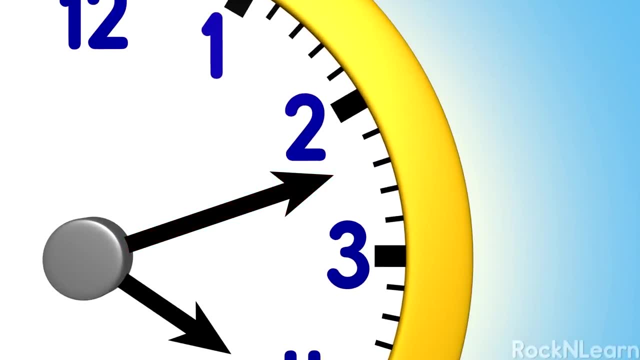 That gives us the hour. Now we need the minutes. So find the minute hand and count by fives, the way we do. We'll stop on the number before the minute hand. we and you Then count up one number for each little line. 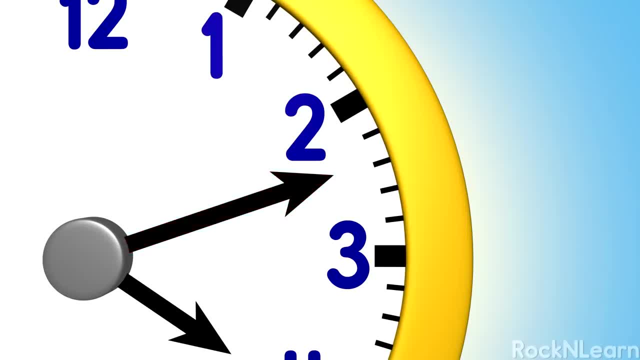 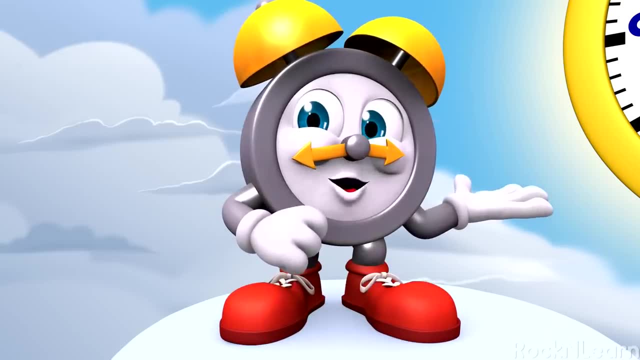 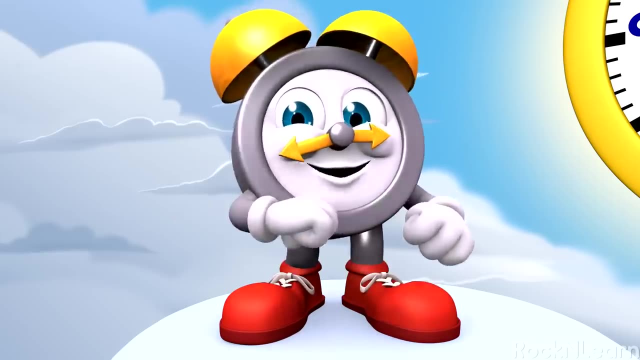 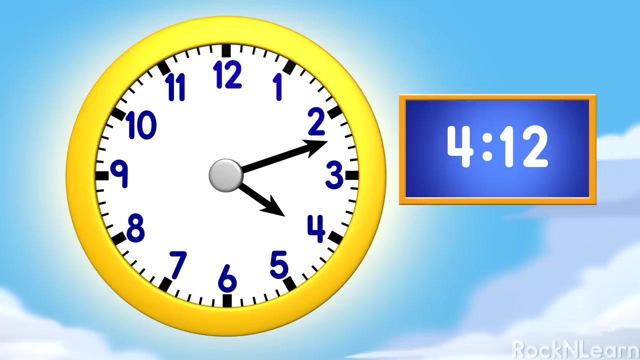 When we reach the minute hand, then the minutes we will find. Put the hour and the minutes together for the time. We'll practice a few here, so you understand my rhyme. This one is for twelve. Find the hour, Count by fives. 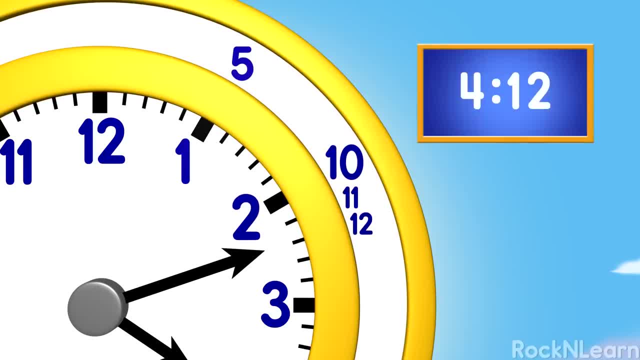 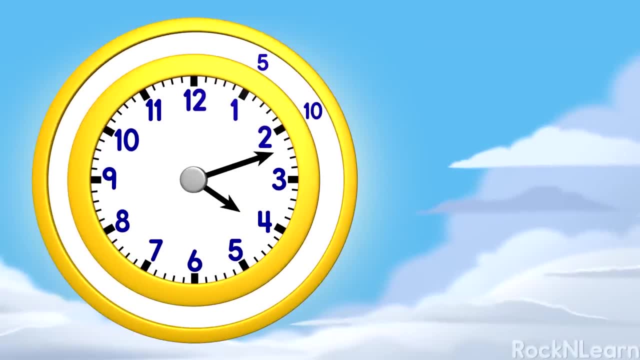 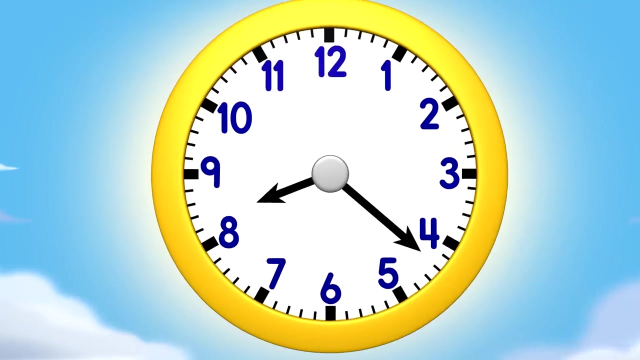 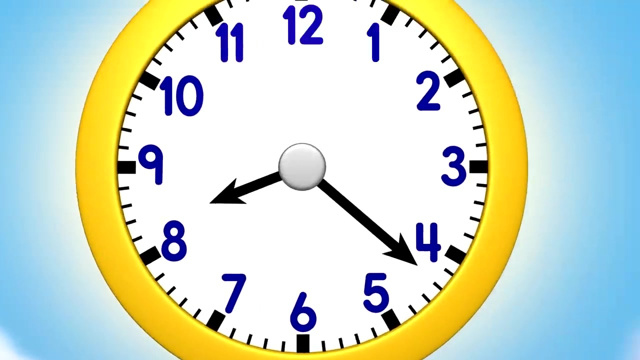 Count the lines to find the time. Find the hour. Count by fives. Count the lines to find the time. Let's do some more: Find the hour. The hour hand's just past the eight. Count by fives. Five, ten, fifteen. 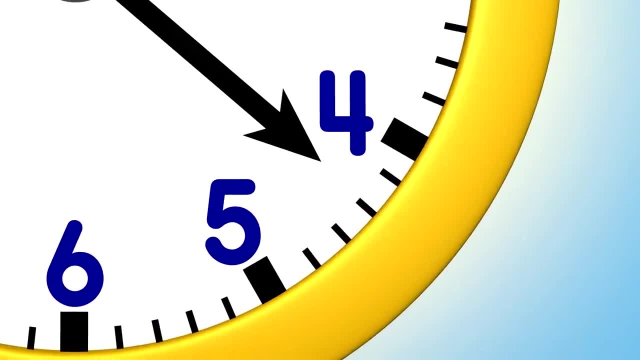 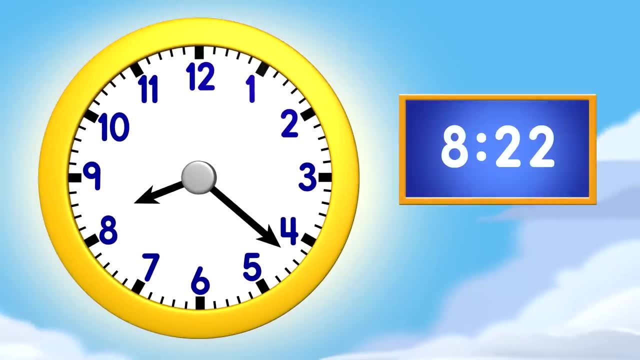 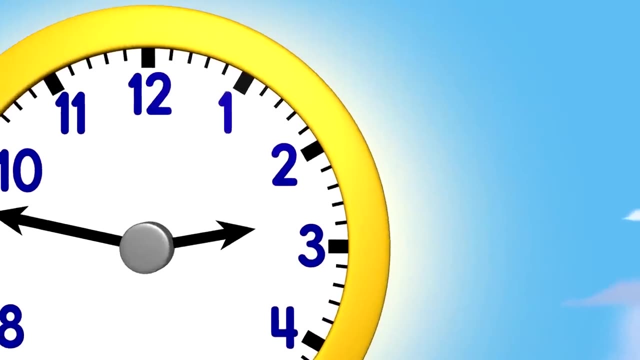 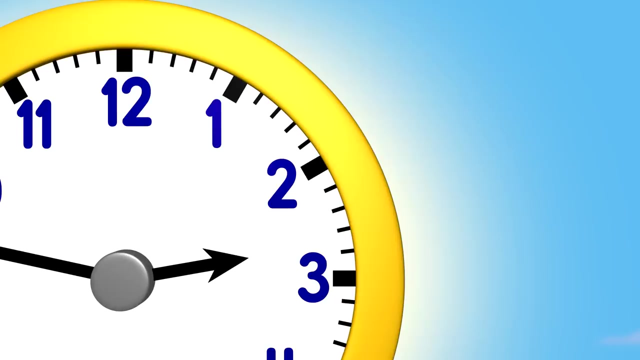 Twenty, Count the lines. Twenty-one, twenty-two, Find the time. Eight-twenty-two, Find the hour. The hour hand's almost to the three. Go back to the two. Count by fives. Here we go. Five, ten, fifteen. 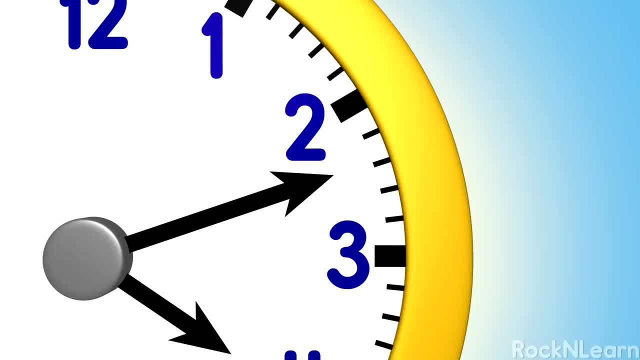 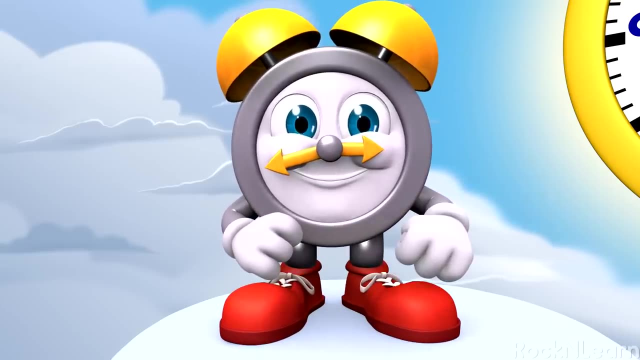 Then count up one number for each little line. When we reach the minute hand, then the minutes we will find. Put the hour and the minutes together. for the time We'll practice a few here, so you understand my rhyme. This one is four-twelve. 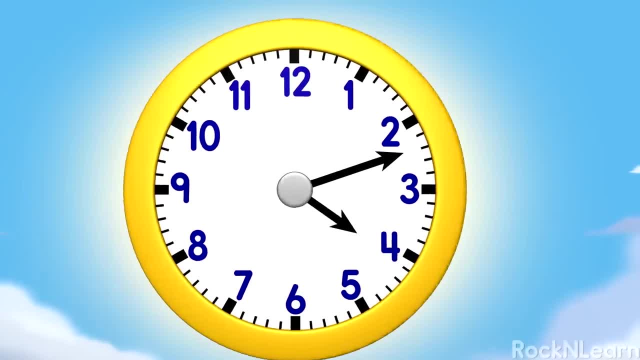 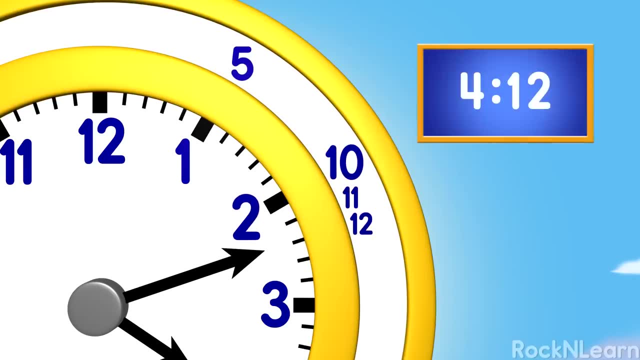 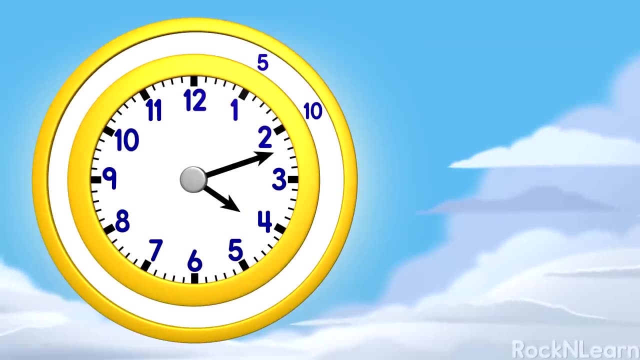 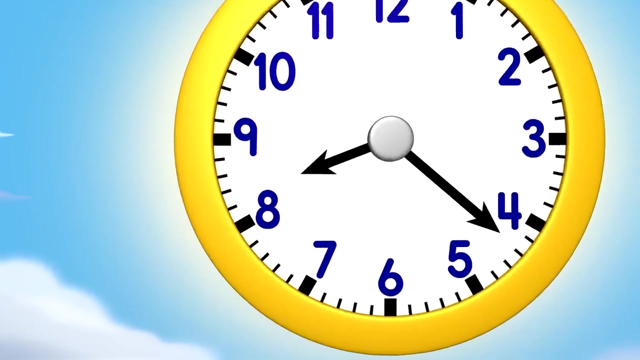 Find the hour: Count by fives. Count the lines to find the time. Find the hour: Count by fives. Count the lines to find the time. Let's do some more. Find the hour. The hour hand's just past the eight. 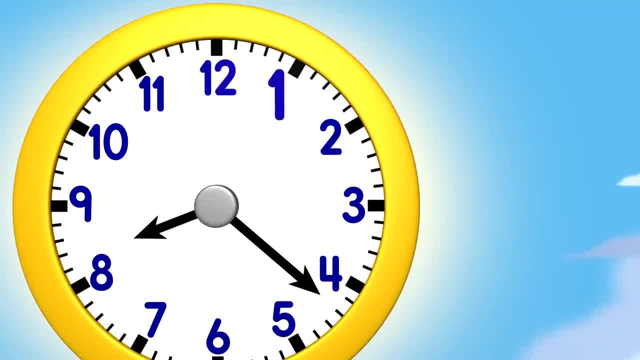 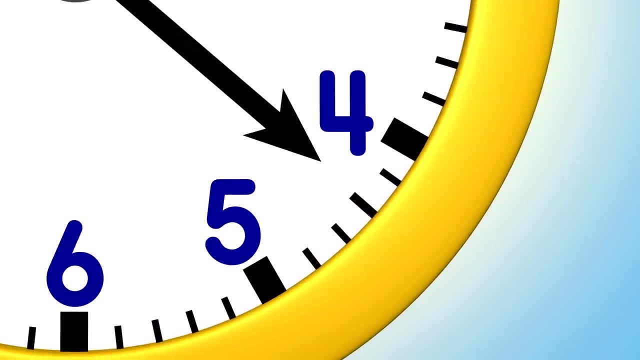 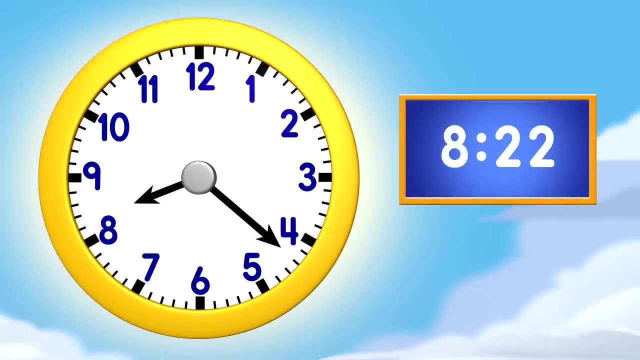 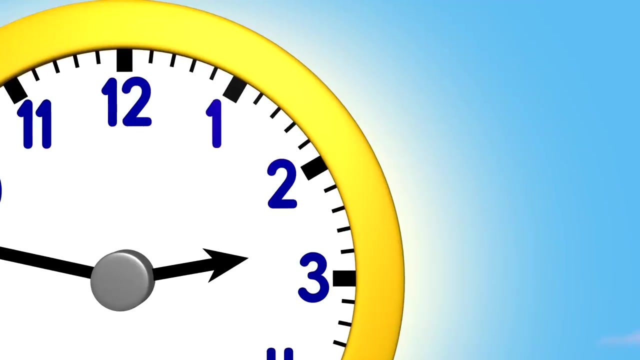 Count by fives. Five, ten, fifteen, twenty. Count the lines. Twenty-one, twenty-two, Find the time. Eight-twenty-two, A hundred-漂亮, Find the hour. The hour hand's almost to the three. 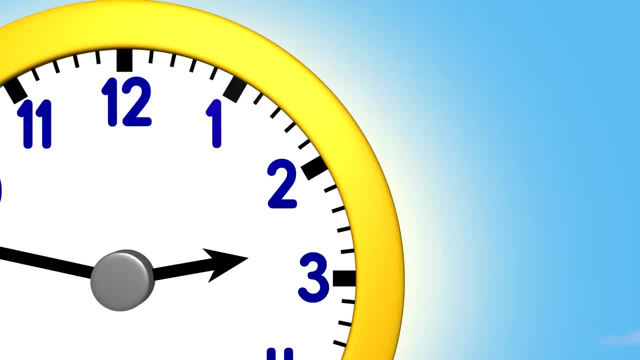 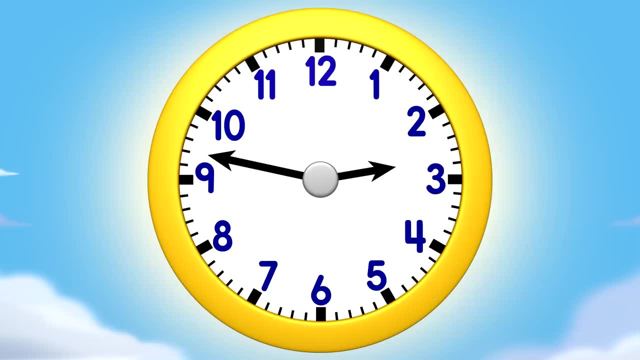 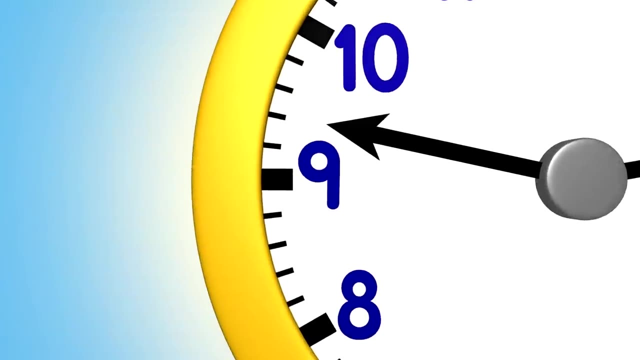 Go back to the two. Count by fives. Here we go. Five, ten, fifteen, twenty, Twenty-five, thirty, Thirty-five, forty, Forty-five. Count the lines Forty-six, forty-seven, Five, ten, fifteen, twenty. 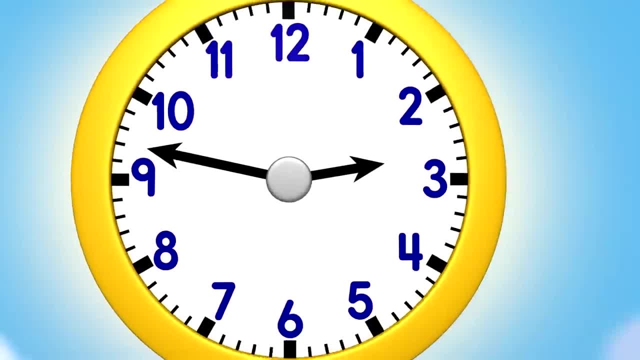 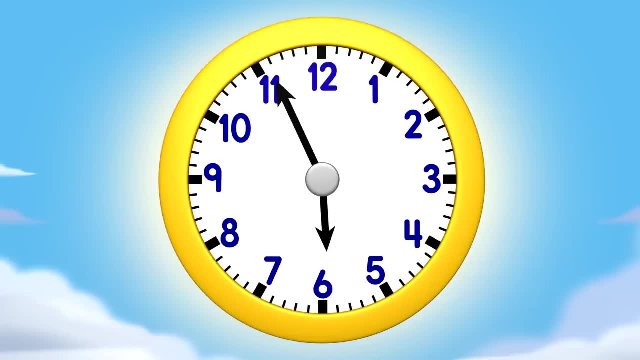 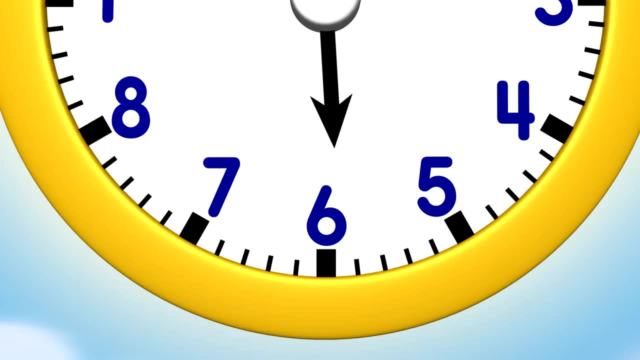 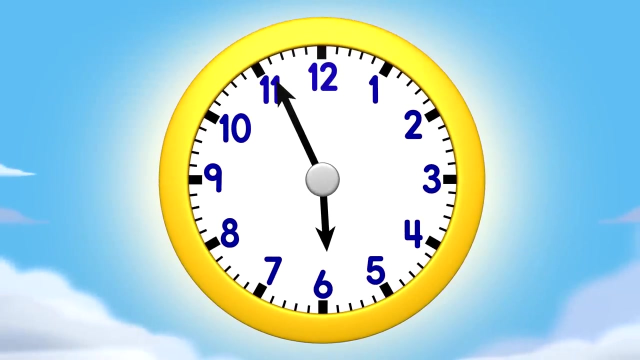 Twenty-five, thirty, thirty-five, forty, forty-five. Count the lines. Find the time. Two, forty-seven. Find the hour. The hour hand's almost at the six. Go back to the five. Count by fives. Five, ten, fifteen, twenty. 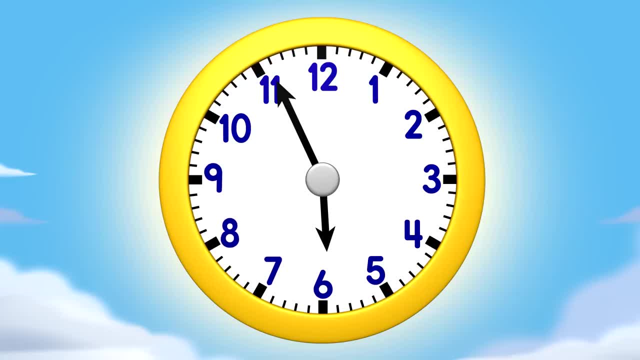 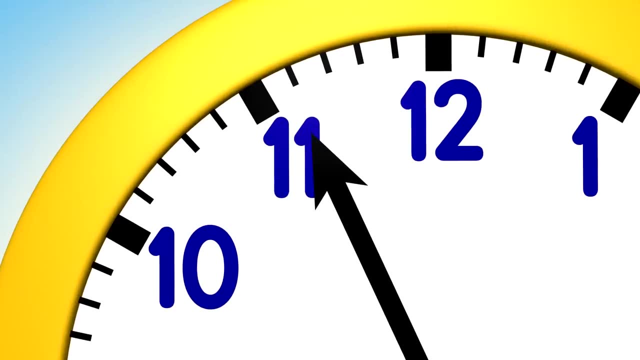 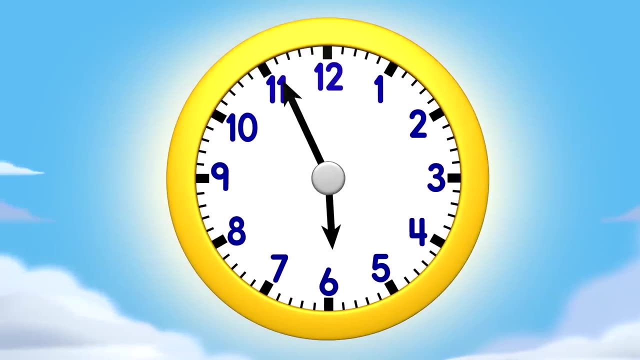 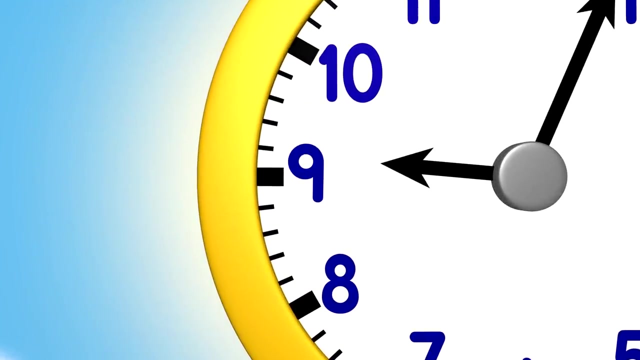 twenty-five, thirty, thirty-five, forty, forty-five, fifty, fifty-five. Count the lines. Fifty-six Find the time. Five. fifty-six Find the hour. The hour hand's just barely past the nine. Count by fives. 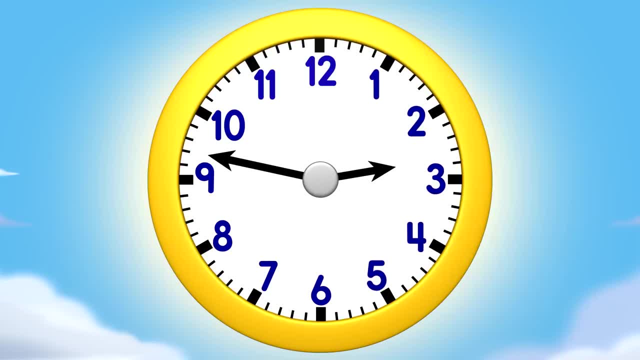 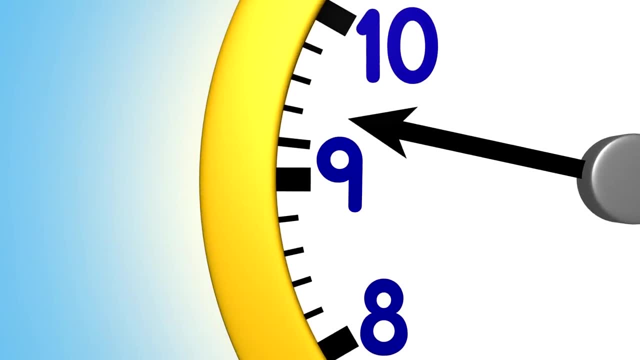 Twenty, Twenty-five, thirty, Thirty-five, forty, Forty-five. Count the lines Forty-six, Forty-seven. Find the time Two, forty-seven, One, two, three, four, five, six, seven, eight, Two, forty-seven. 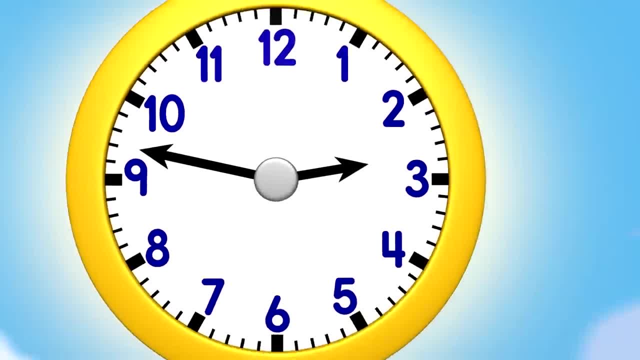 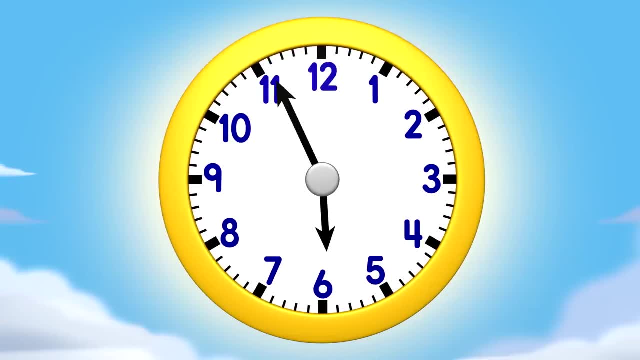 Find the hour. The hour hand's almost at the six. In short, one by four, Two by four, One by five. One by five, Two by six. One by six. Four by five. Two by five, One by six. 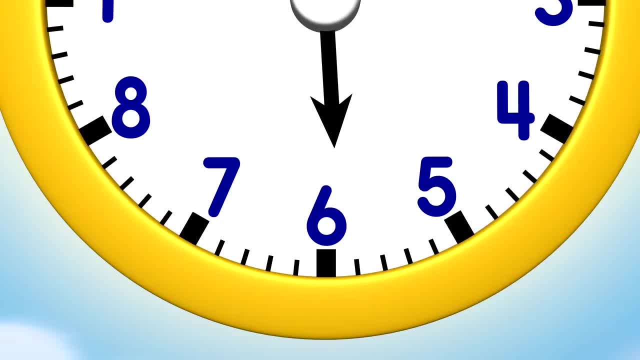 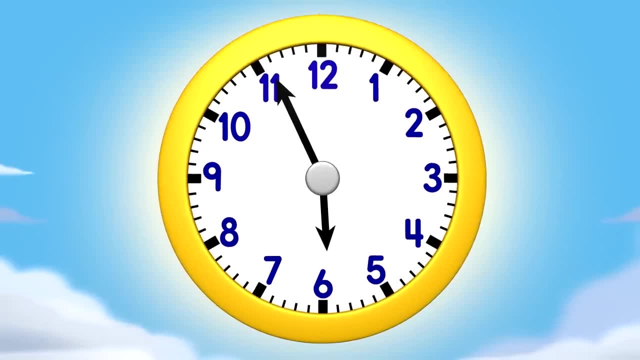 One by seven, One by eight, Two by nine, One by nine, One by twelve, One by twenty. Back to the five. Count by fives. Five, ten, fifteen, twenty, twenty-five, thirty, thirty-five, forty, forty-five, fifty, fifty-five. 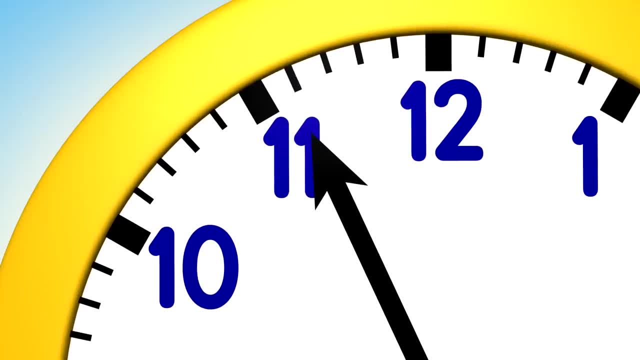 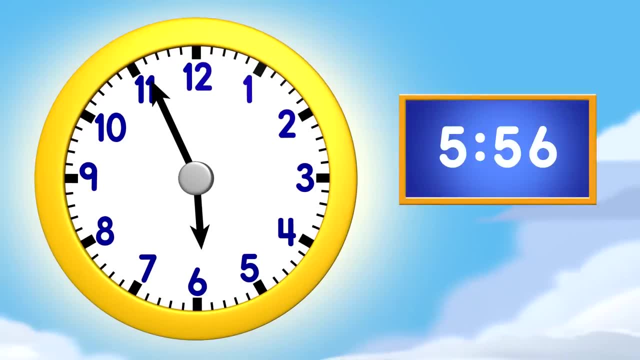 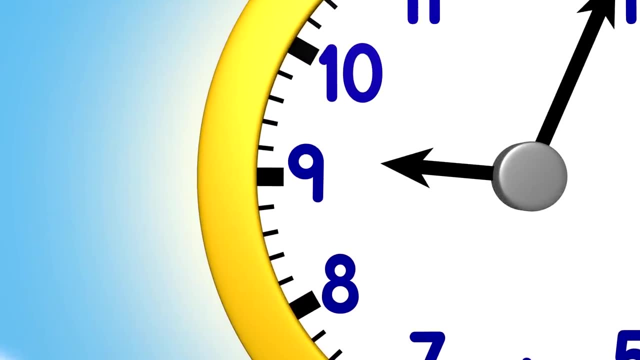 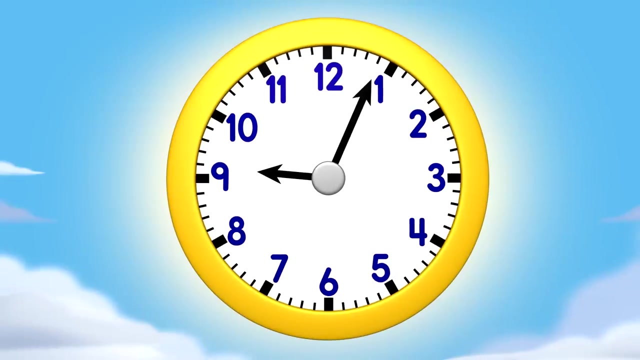 Count the lines. Fifty-six Find the time. Five-fifty-six Find the hour. The hour hands just barely passed the nine. Count by fives. There are no fives to count, so start at zero. Count the lines. 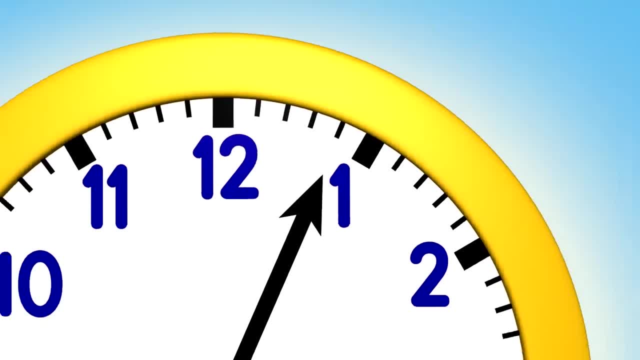 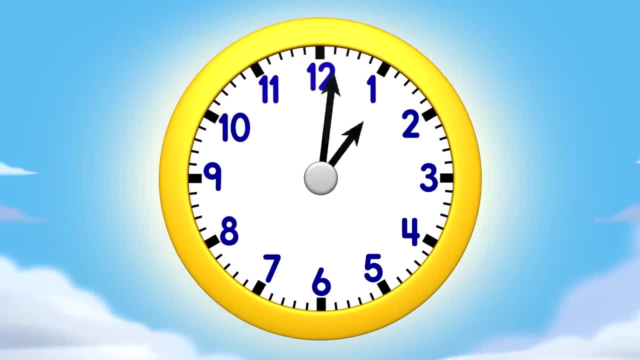 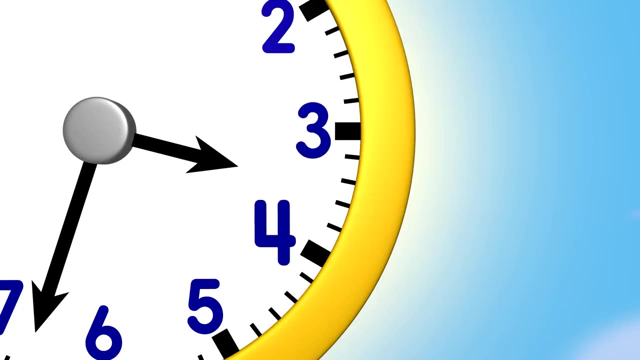 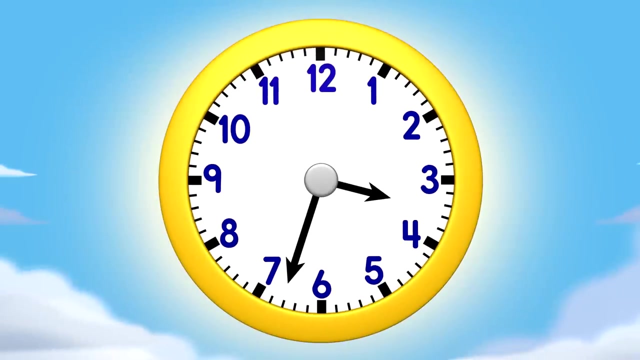 One, two, three, four. Find the time It's nine-oh-four. Find the hour. The hour hands between the three and four Go back to the three. Count by fives. Let's do it. Five, ten, fifteen, twenty, twenty-five, thirty. 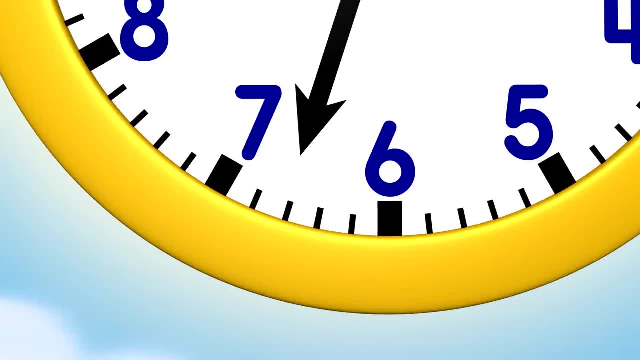 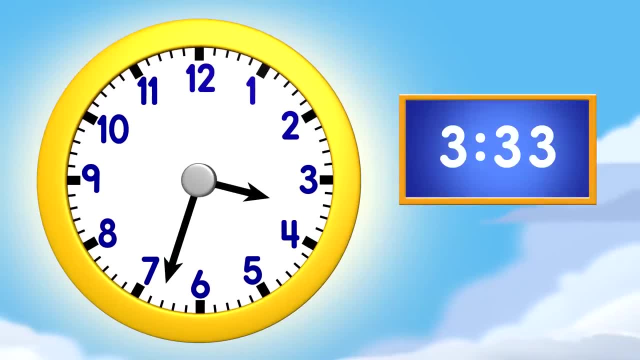 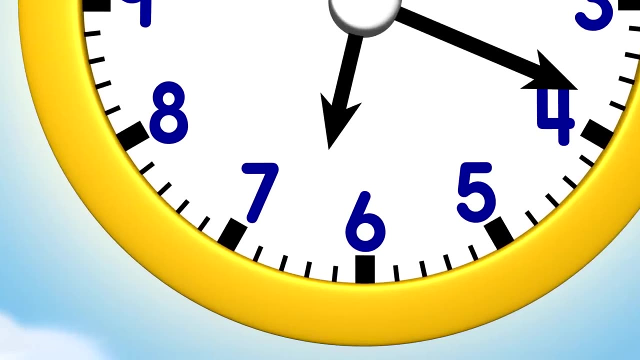 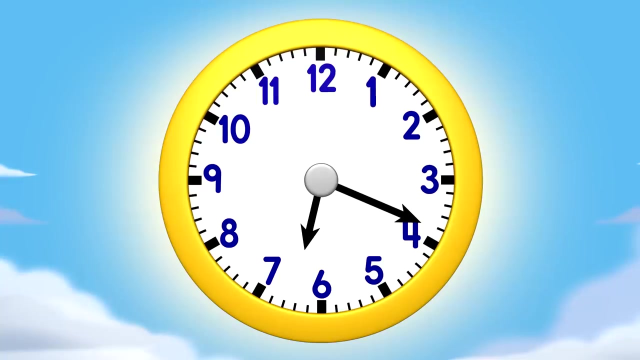 Count the lines. Thirty-one, thirty-two, thirty-three, Find the time It's three-thirty-three, Coo-coo, Find the hour. The hour hands past the six. Count by fives. Five, ten, fifteen. 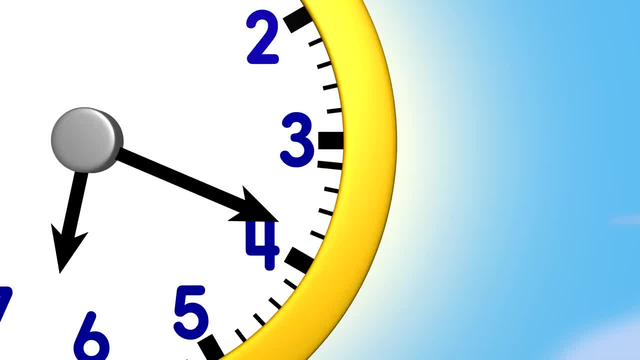 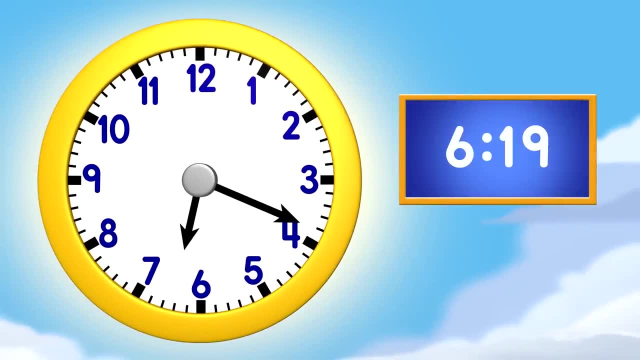 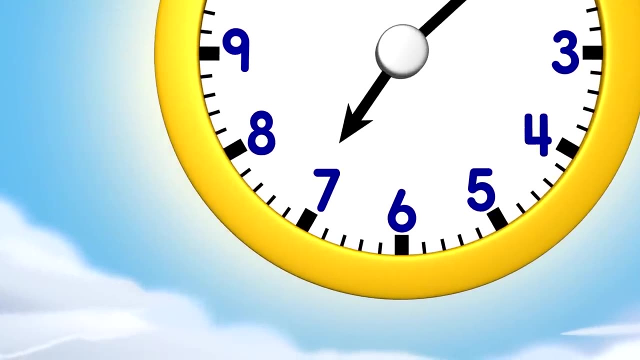 Count the lines. Sixteen, seventeen, eighteen, nineteen Find the time. Six-nineteen, Coo-coo. Fifteen, eighteen, nineteen Find the hour. The hour hands just barely past the seven. Count by fives. 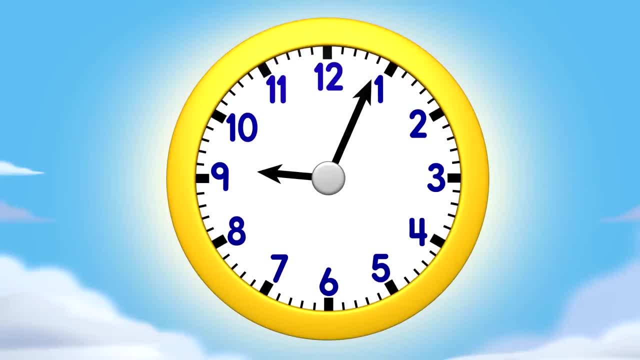 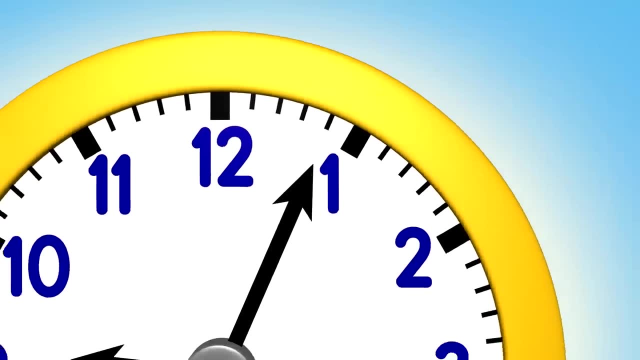 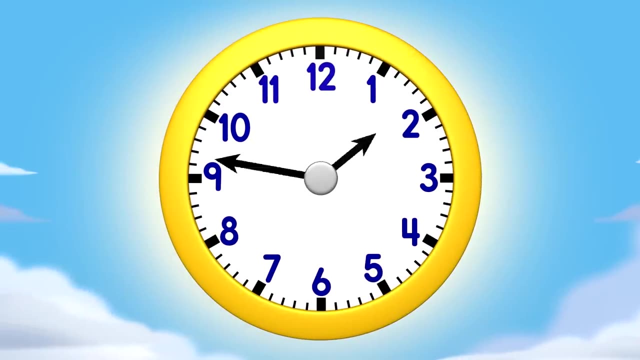 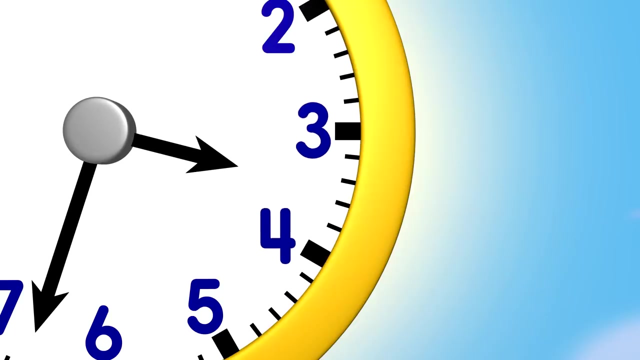 There are no fives to count, so start at zero. Count the lines One, two, three, four. Find the time. It's nine-oh-four. Find the hour. The hour hand's between the three and four. Go back to the three. 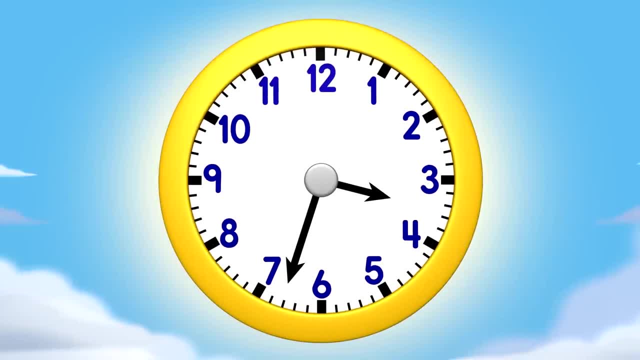 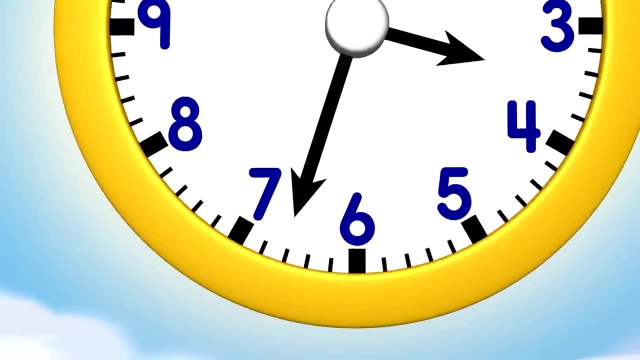 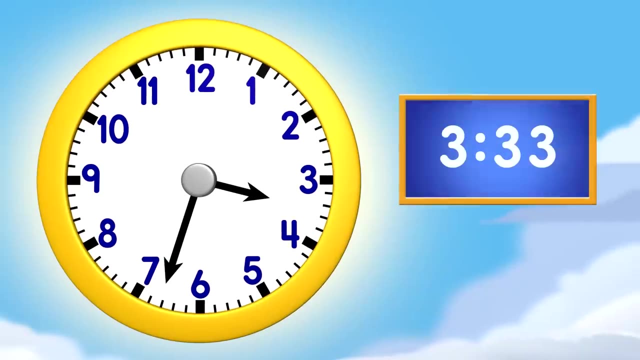 Count by fives. Let's do it. Five, ten, fifteen, twenty, twenty-five, thirty, thirty, thirty. Count the lines. Thirty-one, thirty-two, thirty-three. Find the time, It's three-thirty-three. 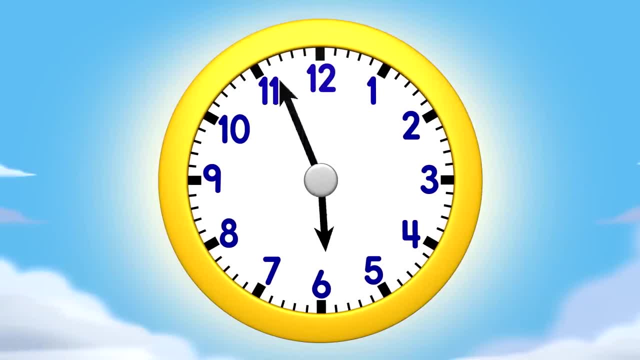 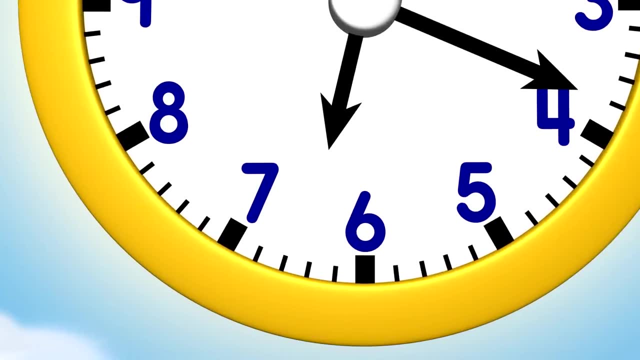 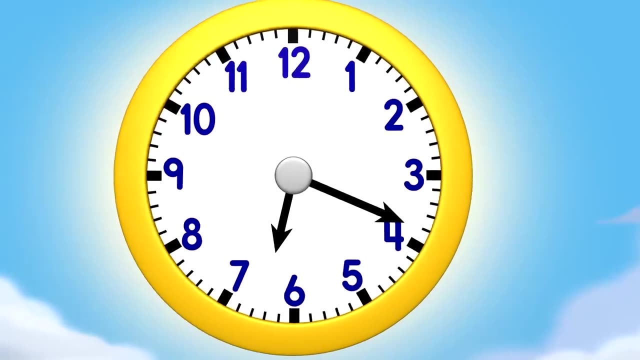 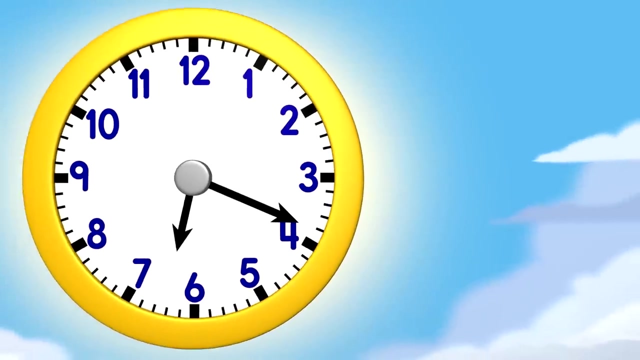 Cuckoo. Find the hour. The hour hand's past the six. Count by fives. Five, ten, fifteen Count the lines Sixteen, seventeen, eighteen, nineteen. Find the time. Six-nineteen, Cuckoo. 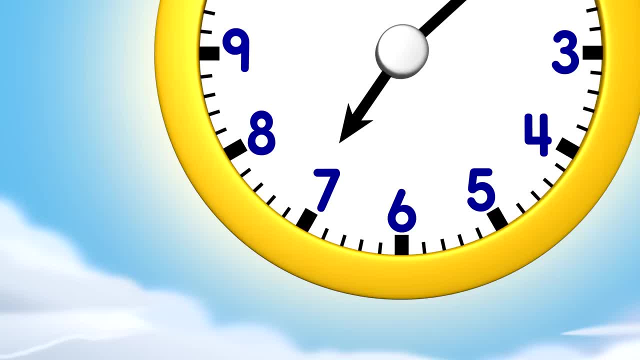 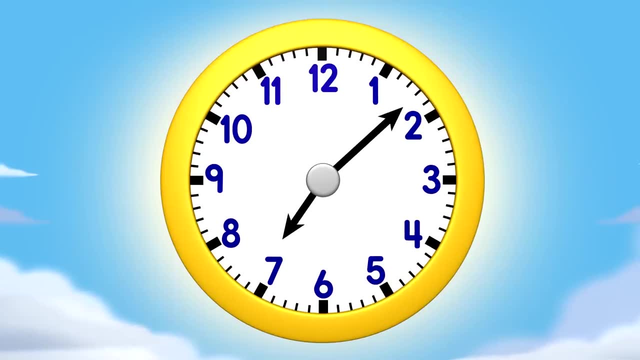 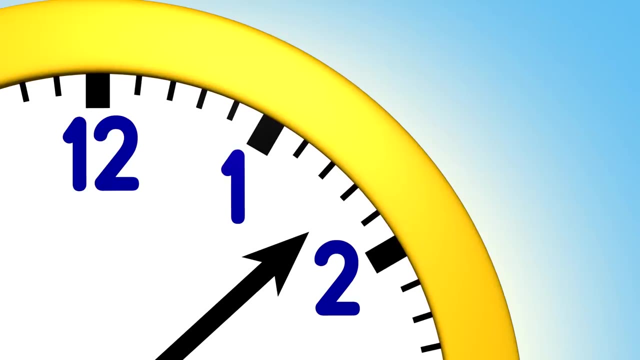 Find the hour. The hour hand's just barely past the seven. Count by fives. Five Count the lines Six, seven, eight Count by fives. Find the time. It's seven-oh-eight, It's seven-oh-eight. 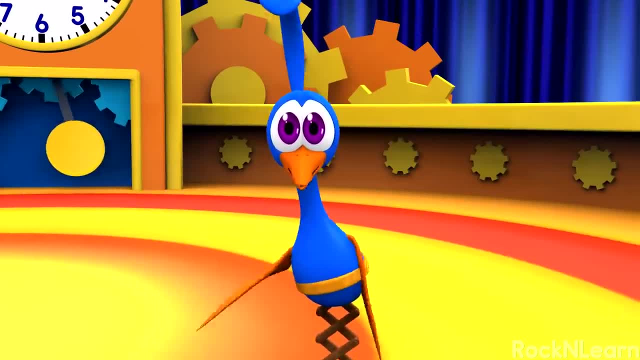 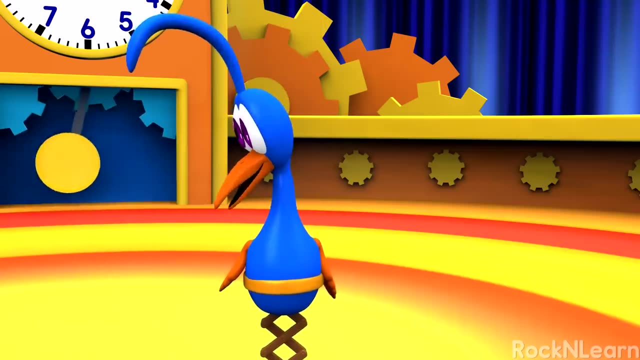 Whoa Hey, watch out, Take cover Incoming Cuckoo, Cuckoo, Cuckoo, Relax Cuckoo. That's my friend Digi. I thought it was an air raid. Don't be silly, Digi isn't attacking. 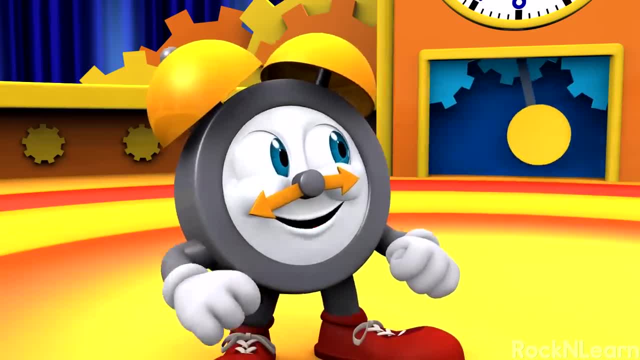 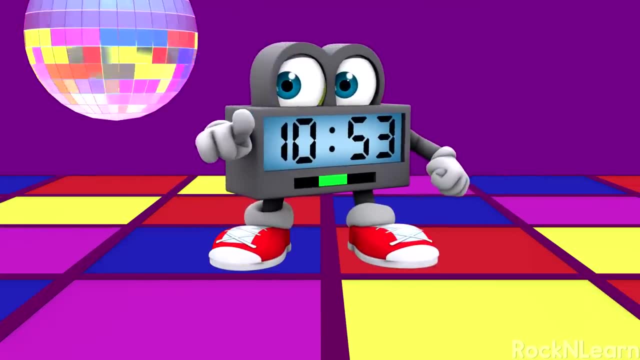 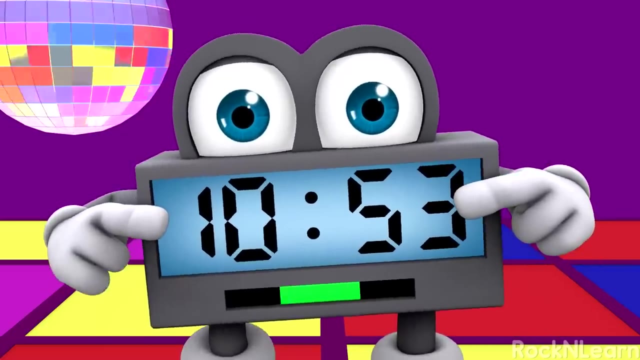 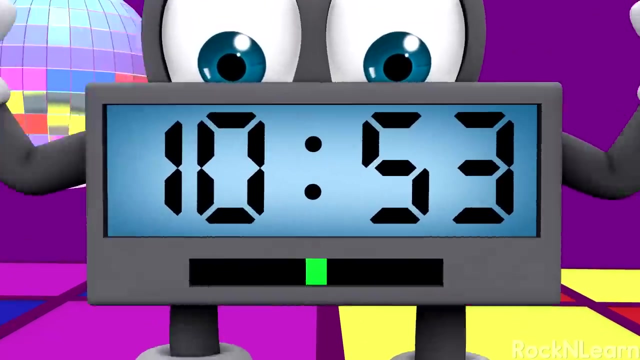 He's come to teach us about telling time with digital clocks and watches. Oh brother, I guess time really does fly. fly when you're having fun, that's right. everybody. i'm digi. i'm the man. let's tell time with the digital watch. i'll show you how you can. just look at my face, look at my face. look at my face. 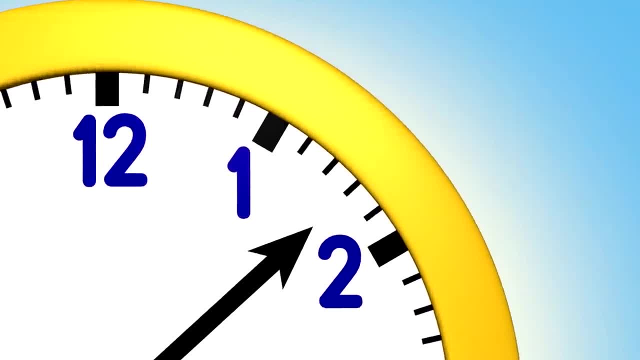 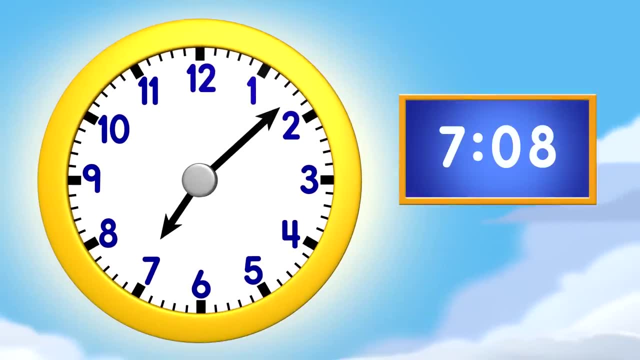 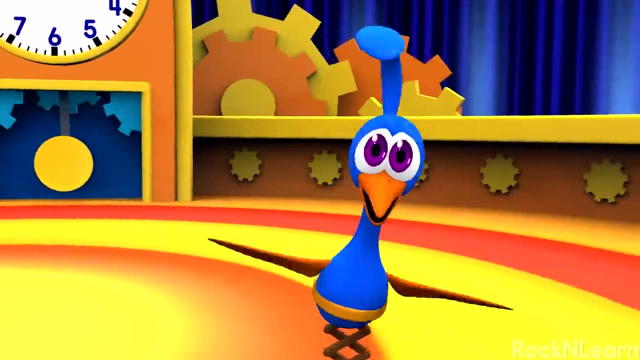 Five, Count the lines Six, seven, eight, Find the time It's seven-oh-eight. Woah, Hey, watch out. Take cover Incoming: cuckoo, cuckoo, cuckoo, cuckoo, cuckoo, cuckoo. 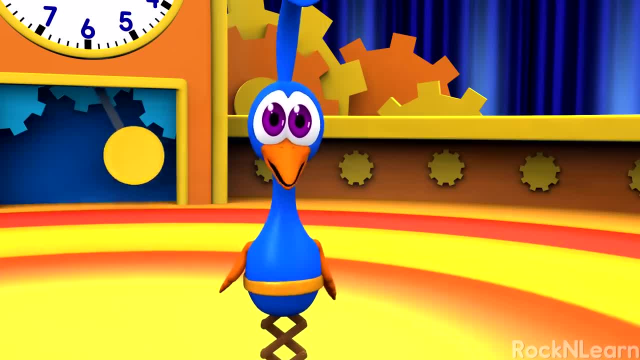 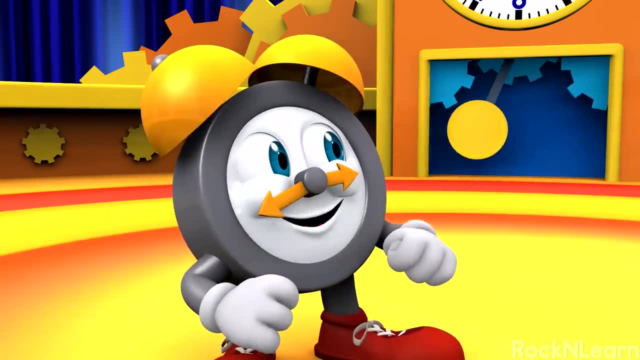 Relax, cuckoo. That's my friend Digi. I thought it was an air raid. Don't be silly, Digi isn't attacking, He's come to teach us about telling time with digital clocks and watches. Oh brother, I guess time really does fly. 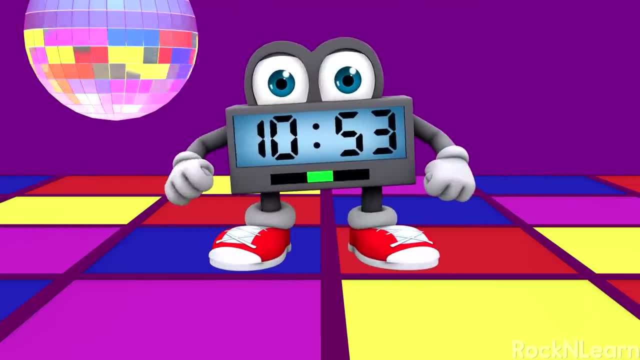 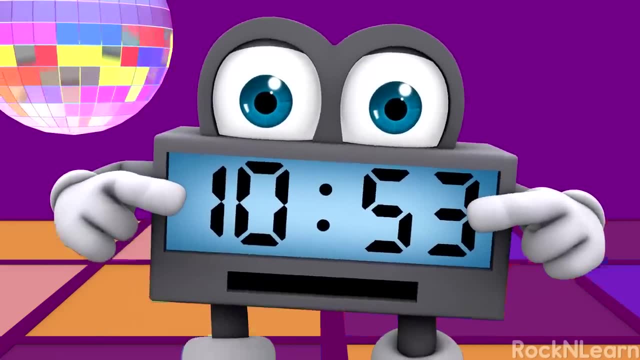 When you're having fun. That's right, everybody. I'm Digi. I'm the man. Let's tell time with a digital watch. I'll show you how you can. Just look at my face, Look at my face. Look at my face. 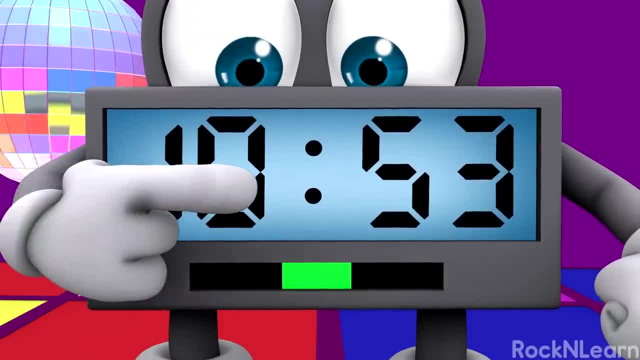 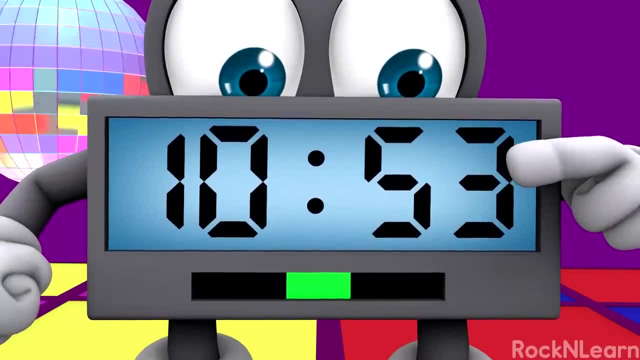 The first number is the hour before the little dots. They are called a colon, those funny little spots. The last numbers are the minutes. They're so easy to read. Just look at them and say the time. Now try a few with me. 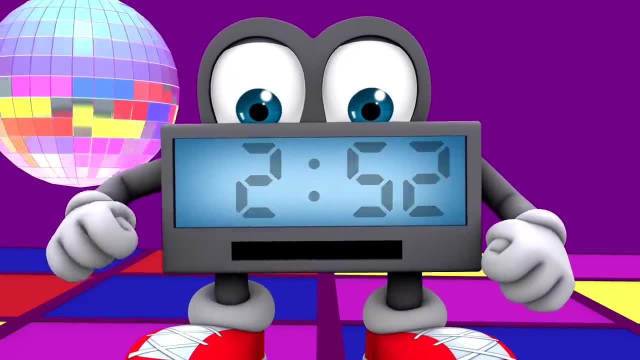 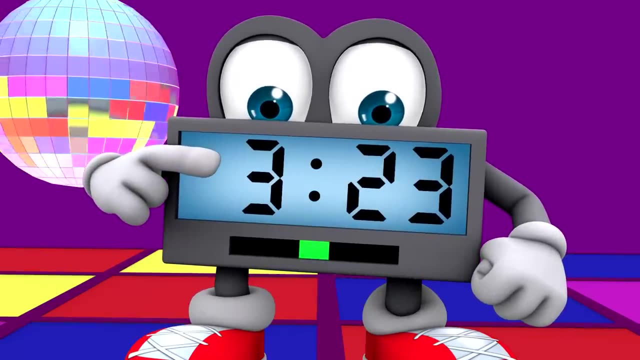 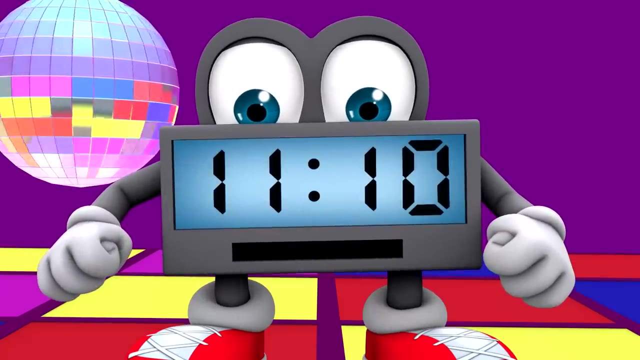 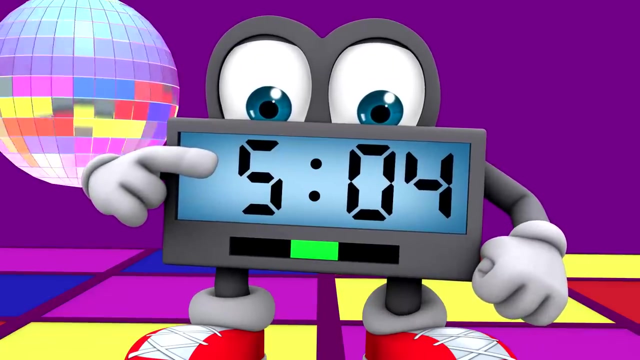 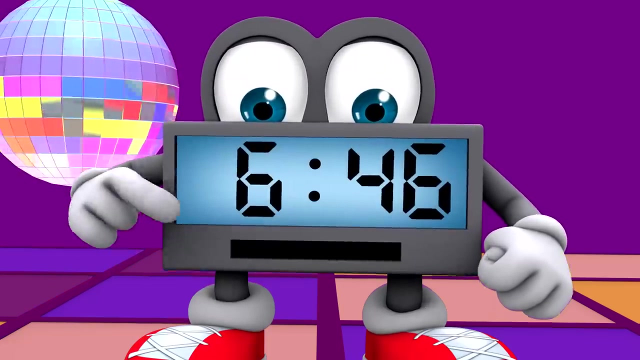 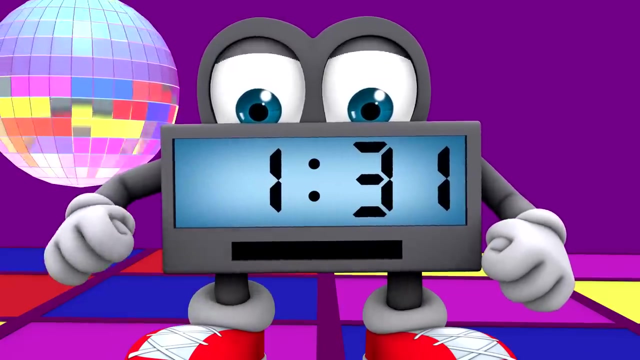 Two-fifty-two, Nine-thirty-nine, Three-twenty-three, Seven-fifty-seven, Eleven-ten, Five-oh-four, Ten-twenty-seven, Six-forty-six, One-thirty-one, Eight-forty-eight, 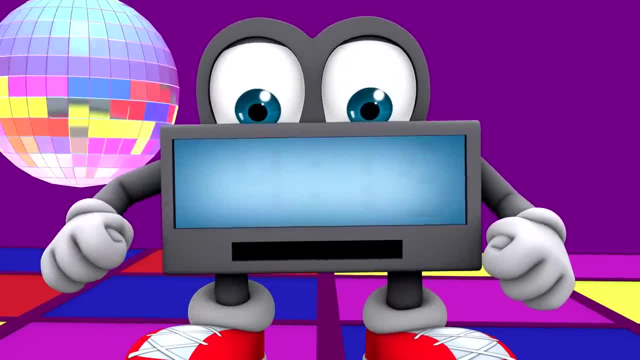 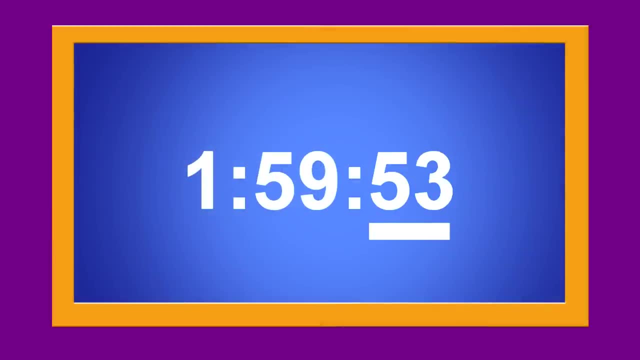 Four-fifteen, Twelve o'clock. Sometimes you see two more Numbers on the face After another colon In the rightmost place. These numbers show the seconds That move so very fast, The seconds past the minute, Past the hour that has passed. 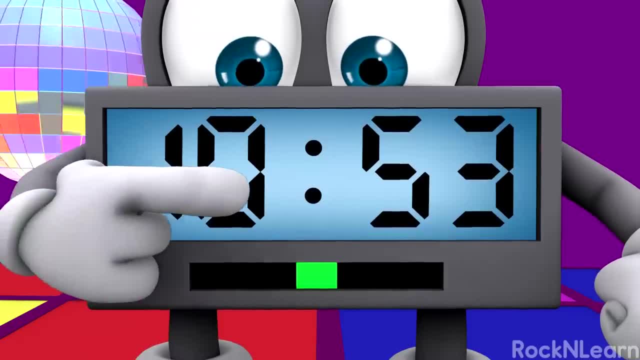 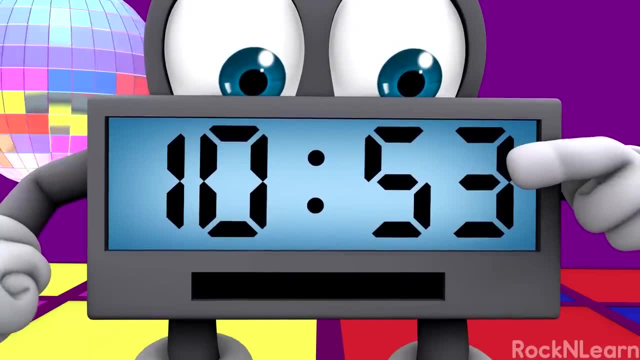 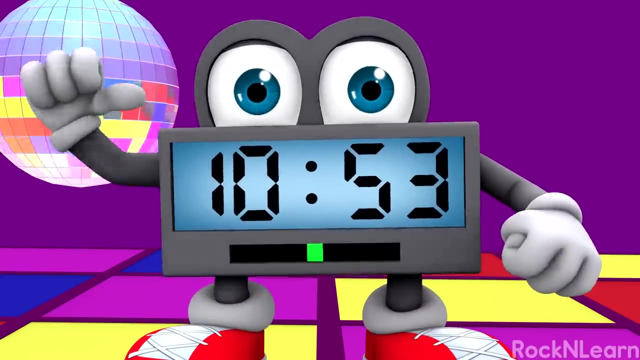 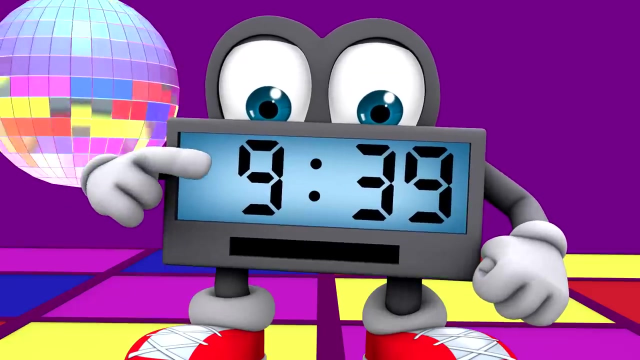 the first number is the hour before the little dots. they are called a colon, those funny little spots. the last numbers are the minutes. they're so easy to read. just look at them and say the time. now. try a few with me: 252 939 323. 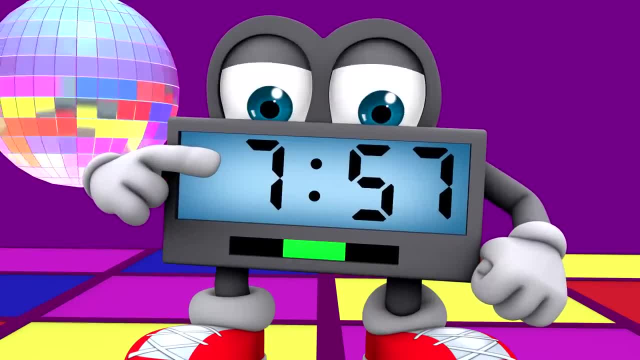 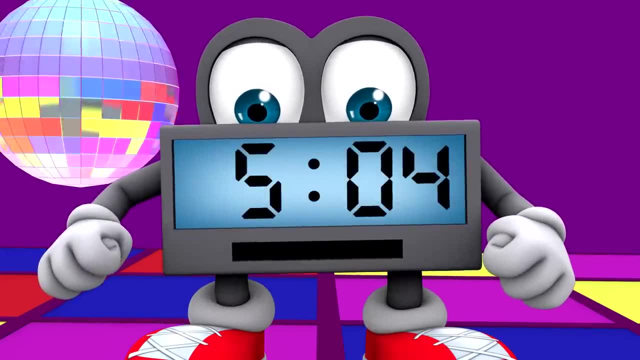 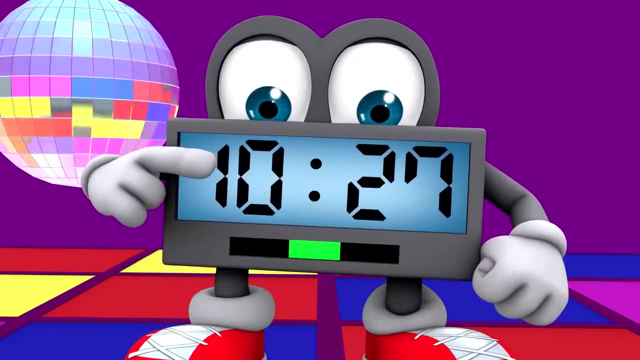 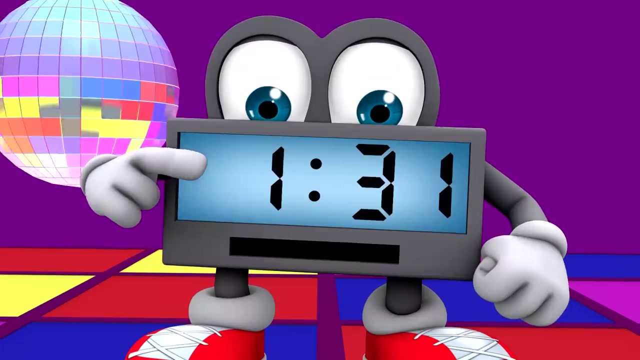 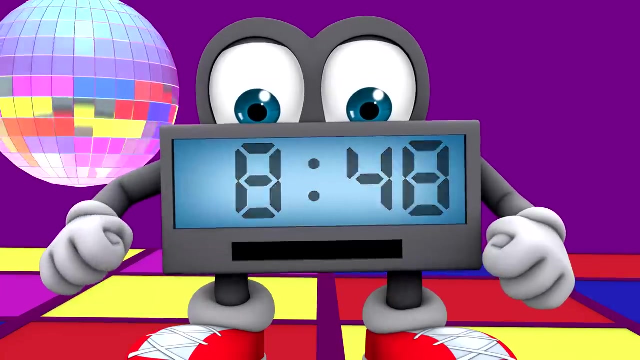 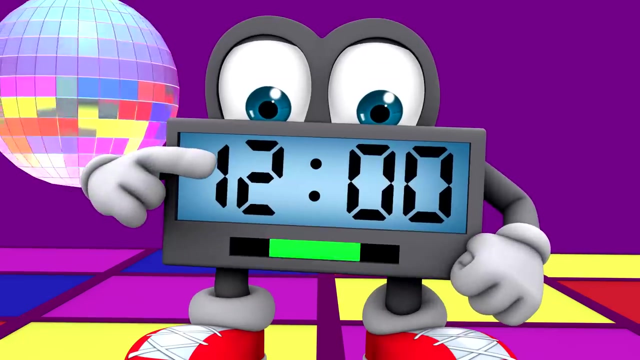 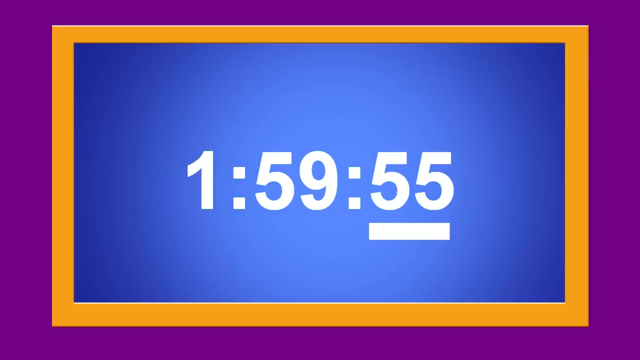 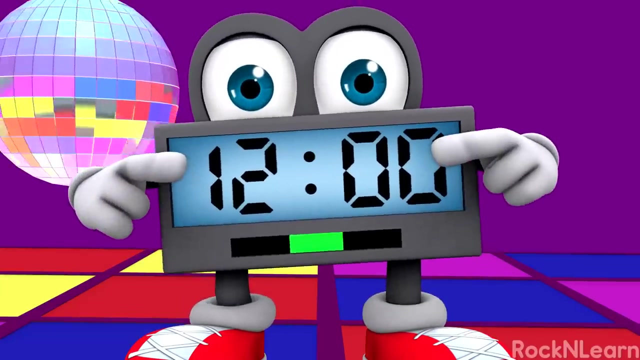 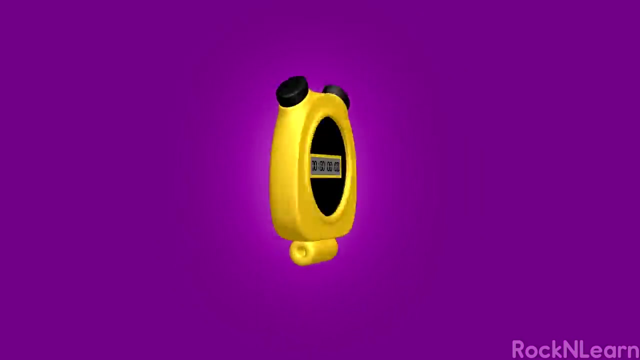 757, 1110, 504, 1027, 646, 131, 848, 415, 1519 Bis, 선택 236, 138, 3, 259, 259, 700, 300, uno Digi a stopwatch is a special watch for measuring short times. 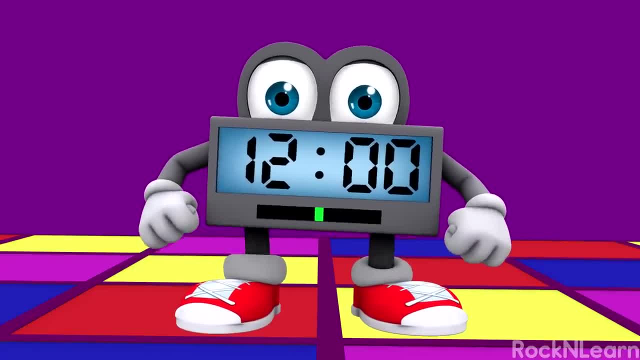 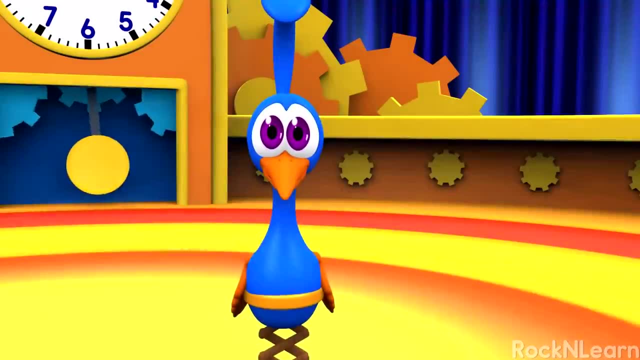 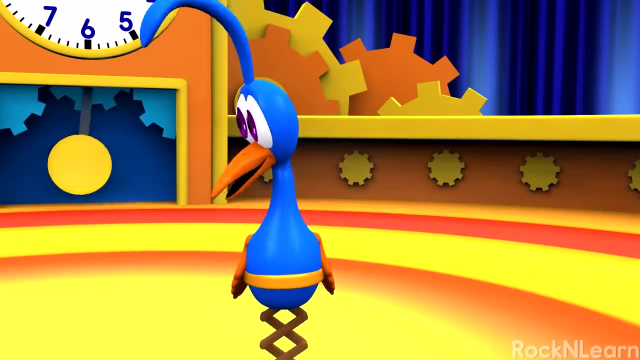 You know it like in a race. Speaking of races, I'm outta here. Whoa, Wow, I guess we know all about time now. Don't be so sure. You mean there's more. That's right, Cuckoo. 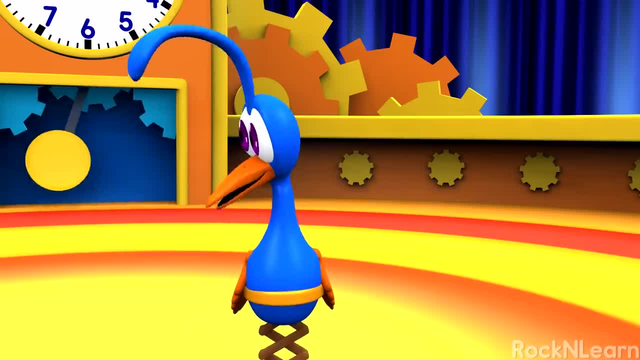 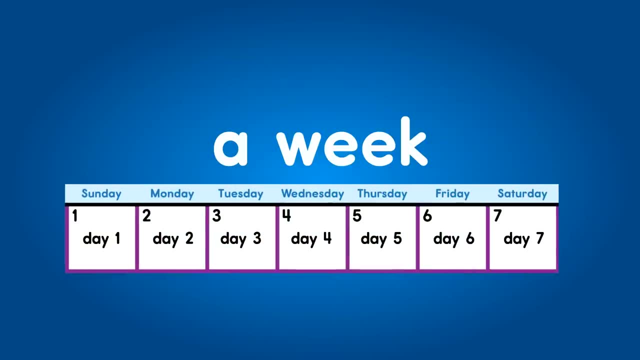 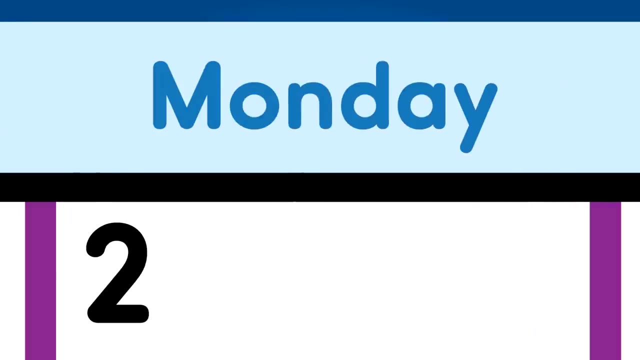 We need to learn about calendars. Okay, There are 24 hours in a day, 7 days in a week. Each day has a special name and each name is unique: Sunday, Monday, Tuesday, Wednesday, Thursday, Friday, Saturday. 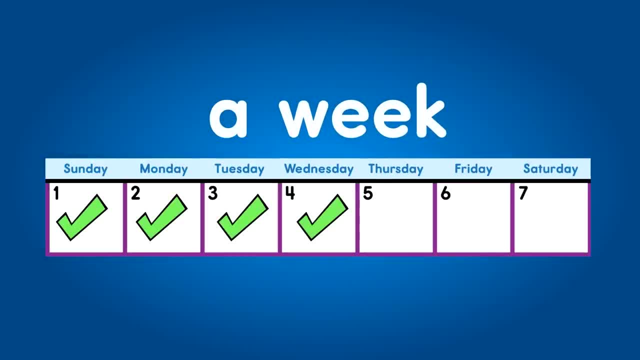 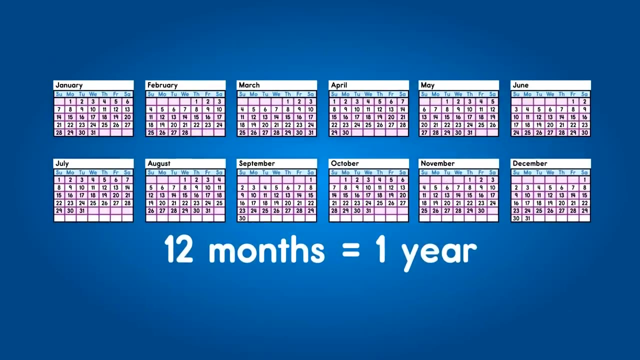 Faster now: Sunday, Monday, Tuesday, Wednesday, Thursday, Friday, Saturday, Sunday, Monday, Tuesday: 52 weeks make up a year, but there is something more. We also have 12 months a year. Come on, let's explore. 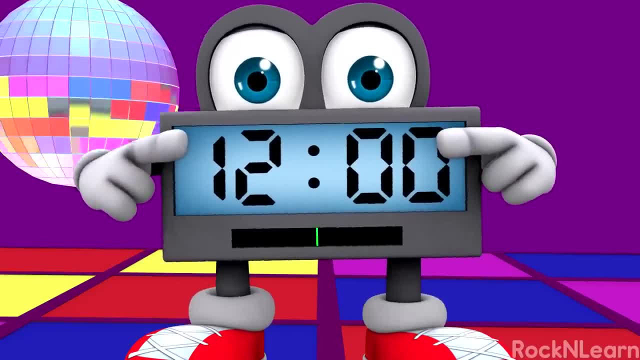 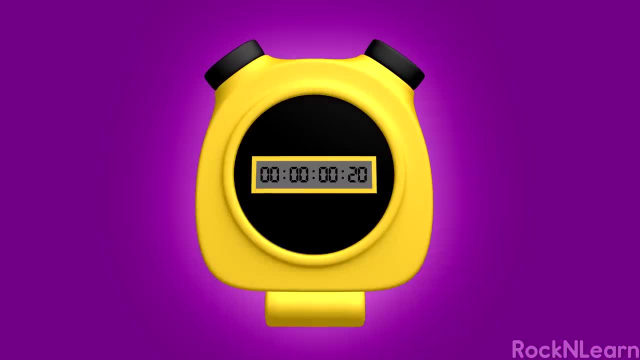 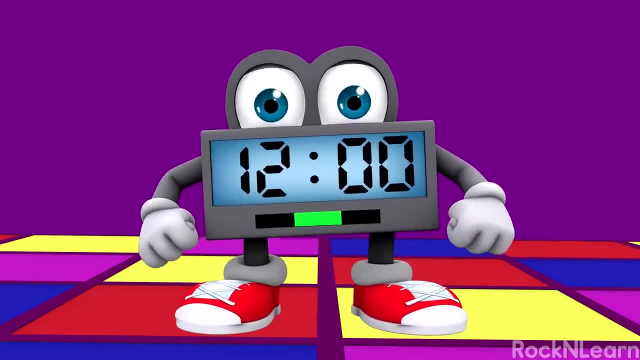 If you see more numbers, it's really not a clock. More likely, it's a gadget That we call a stopwatch. That's right, Digi. A stopwatch is a special watch for measuring short times. You know it, Like in a race. Speaking of races, I'm outta here. 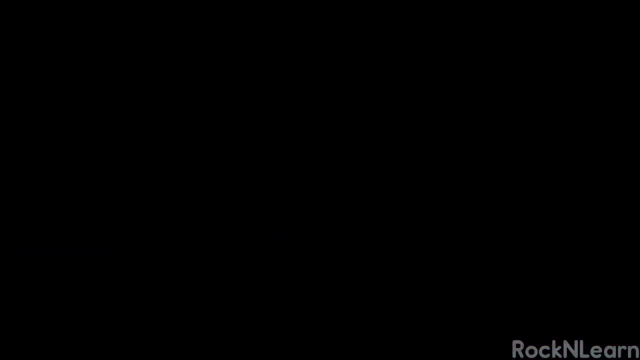 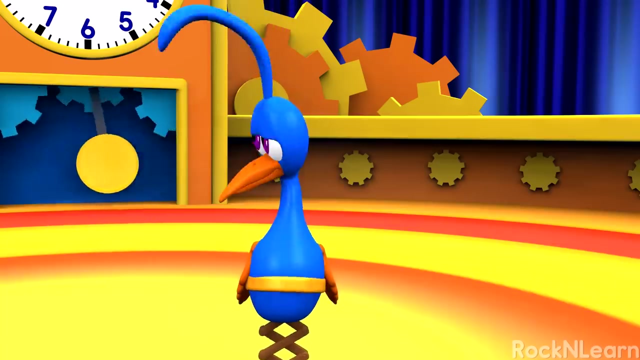 Whoa, Wow, I guess we knew all about time. now Don't be so sure. You mean there's more. That's right, Cuckoo, We need to learn about calendars. Okay, There are 24 hours in a day. 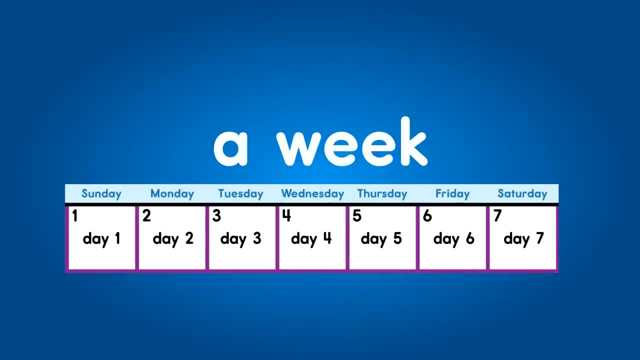 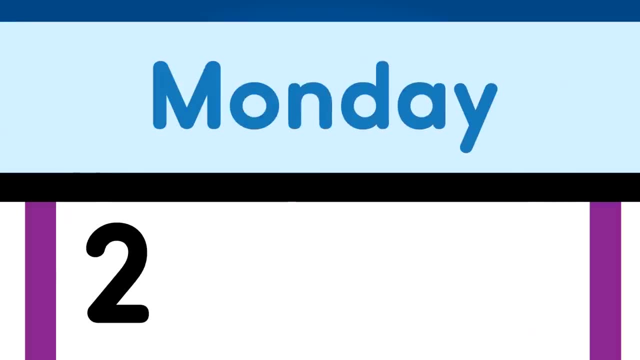 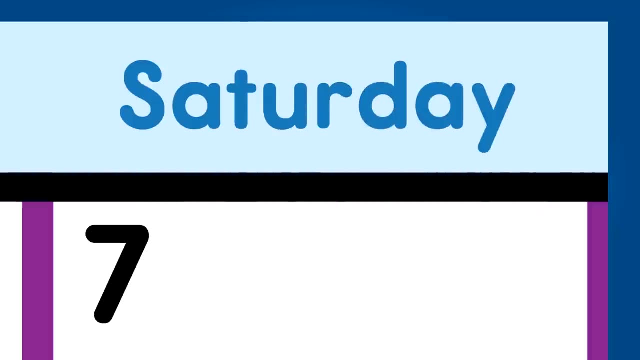 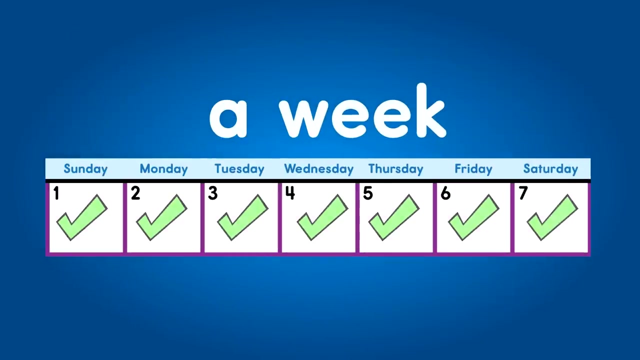 There are 24 hours in a day, Seven days in a week. Each day has a special name and each name is unique. Each day has a special name and each name is unique: Sanday, Sun'tey, Sun'tey, Monday, Tuesday, Wednesday, Thursday, Friday, Saturday- faster now- Sunday, Monday, Tuesday, Wednesday, Thursday, Friday, Saturday, Sunday, Monday, Tuesday, Wednesday, Thursday, Friday, Saturday. 52 weeks make up a year, but there is something more: we also have 12 months a year. 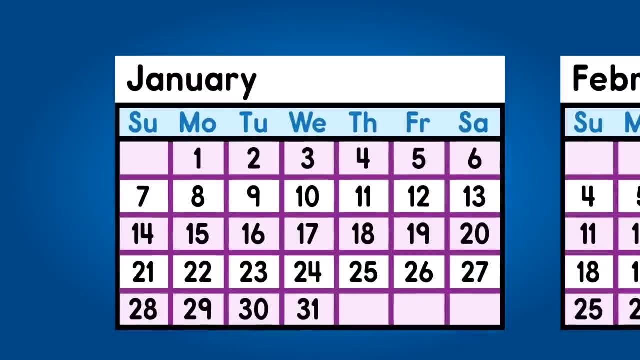 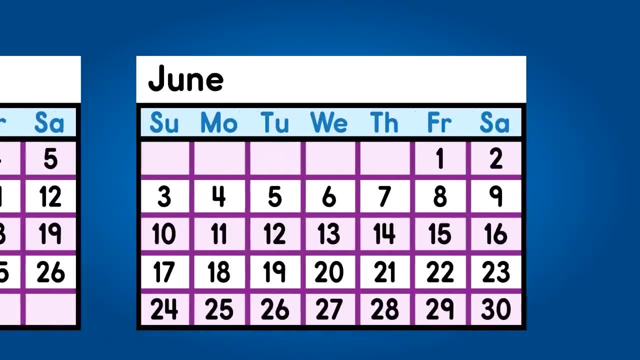 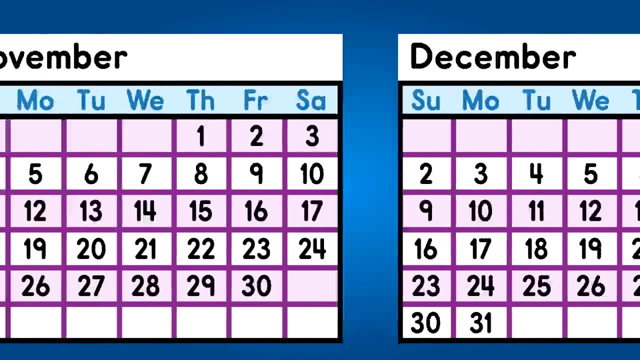 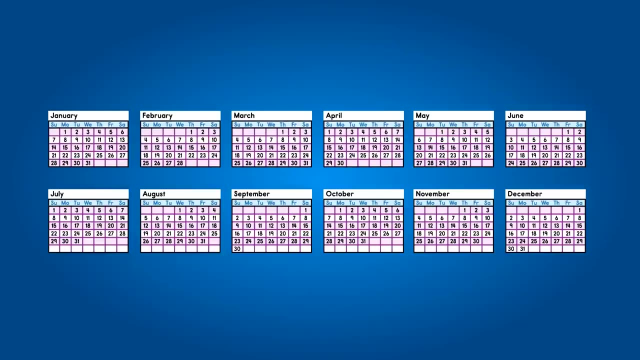 Come on, let's explore January, February, March, April, May, June, July, August, September, October, November, December. let's go a little bit faster now. January, February, March, April, May, June, July, August, September, October, November, December. 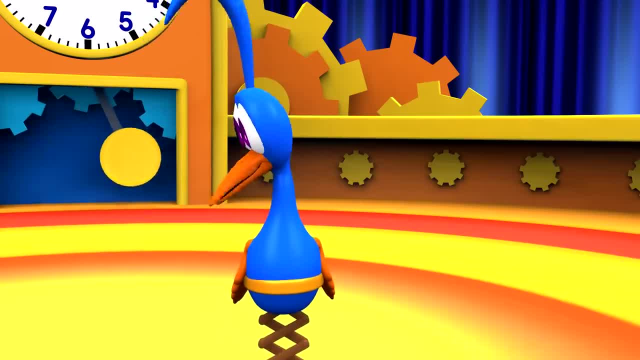 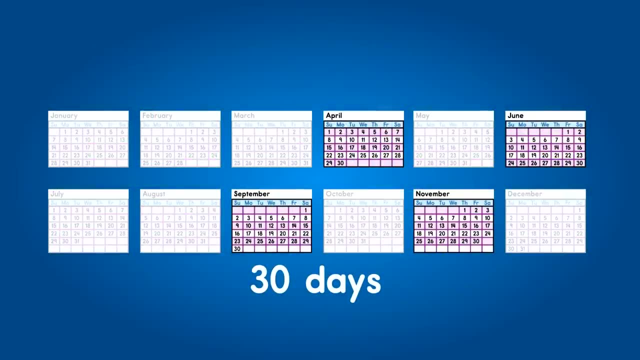 But how many days does a month have? That all depends Cuckoo. 30 days are in September, April, June and November. all the rest have 31,. except for February alone it has 28 days clear and 29 in each leap year. 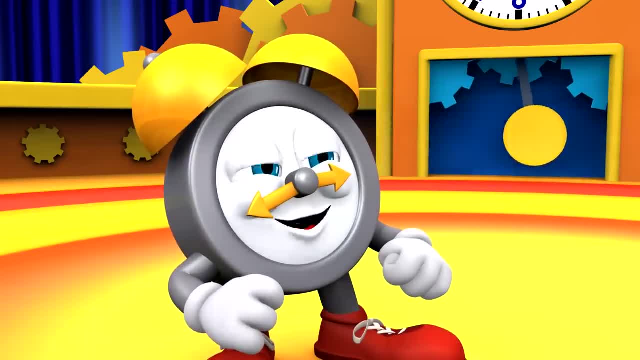 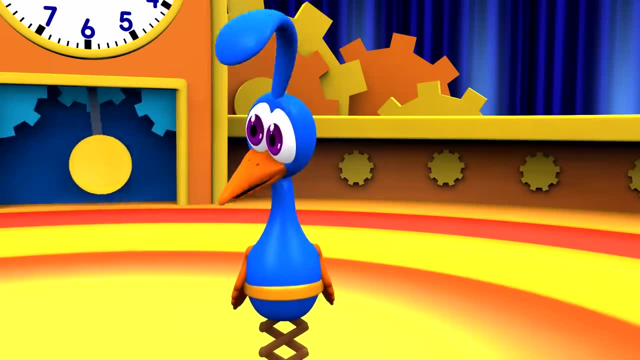 Do we have to jump over it? No, Cuckoo, a leap year is when we add an extra day. Hey, they come every four years most of the time. But how will I know which years are leap years? You can look at a calendar. if the calendar has February 29th on it,